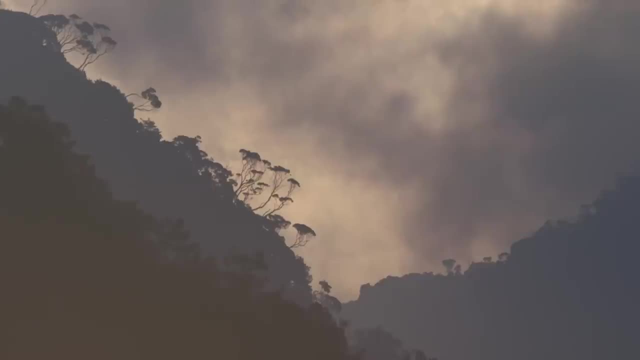 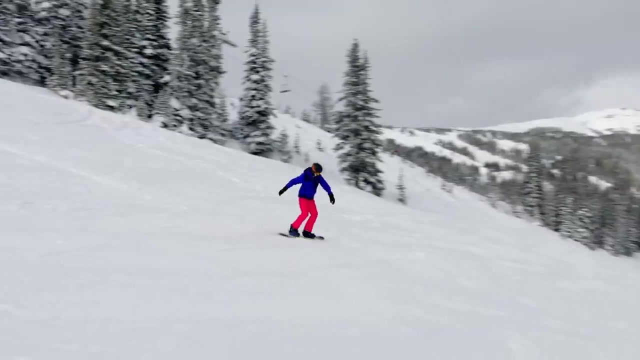 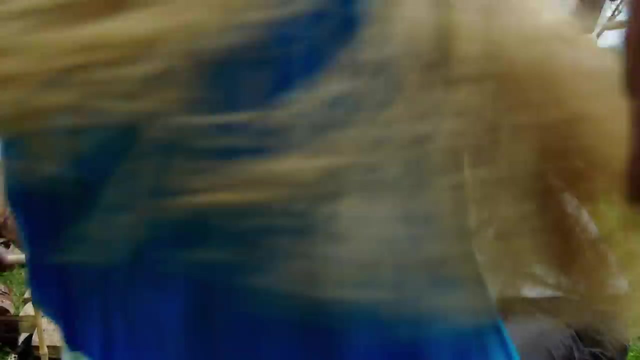 From the peaks of the Korean Peninsula To the Rwenzori Mountains of Africa, From the Alps To the Andes, From the Rockies To the Himalayas, This is the global story of humanity in high places, Of mountains and life. 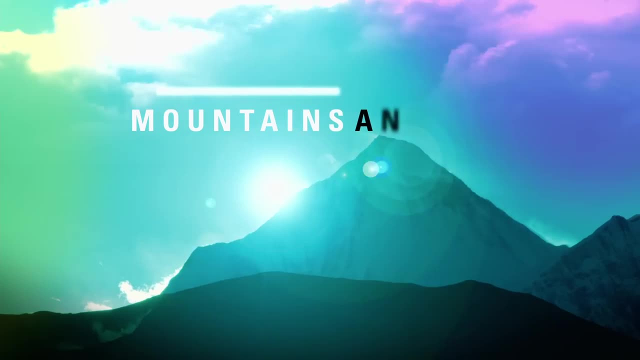 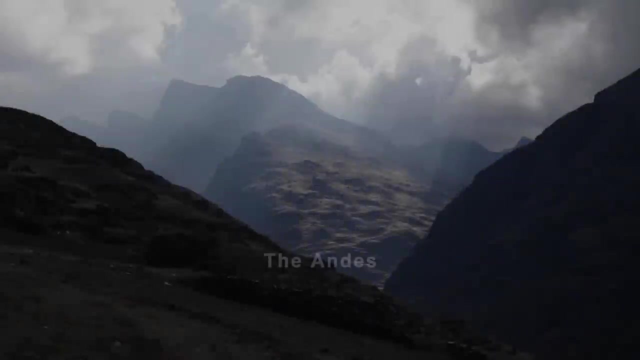 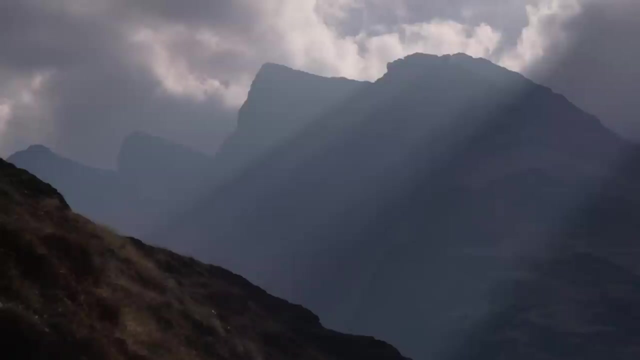 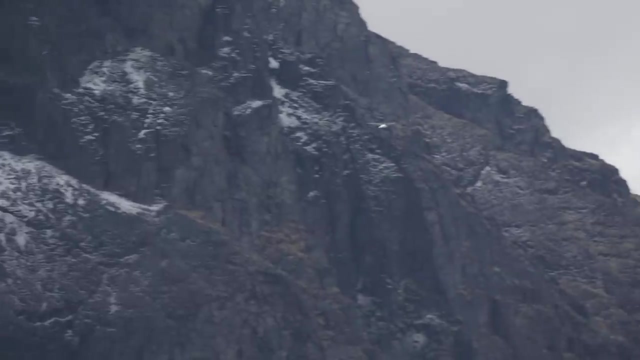 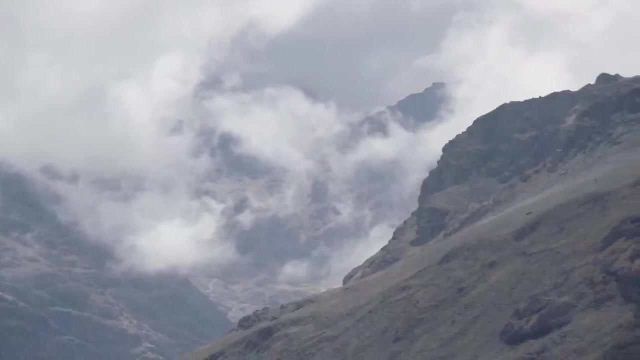 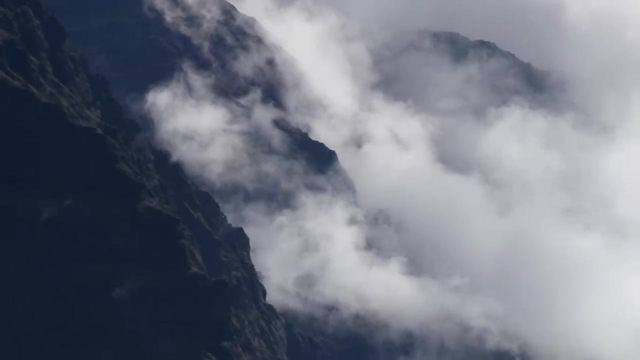 And the world. They span an entire continent, A string of high plateaus and peaks Stretching 7,000 kilometers, From the tip of South America To the Caribbean. The Andes Forged millions of years ago in a series of rapid tectonic upheavals. 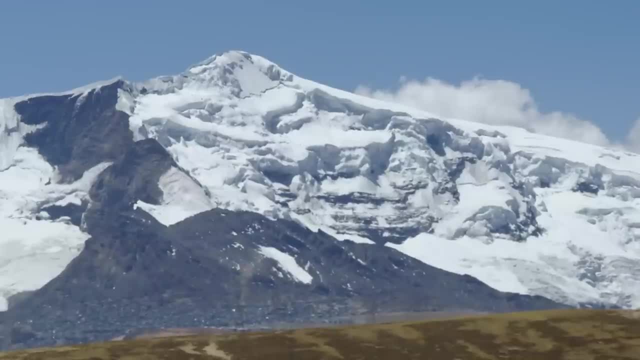 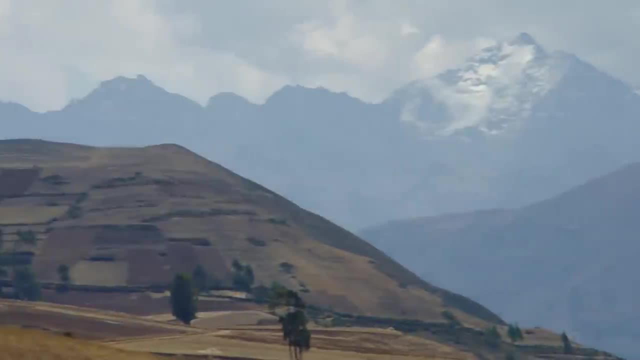 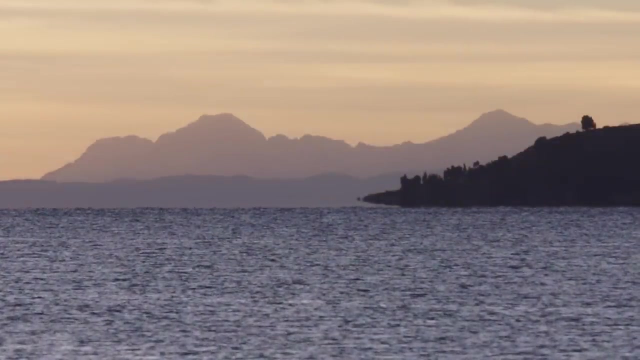 Today, the legacy of that seismic turmoil is a landscape which, on so many counts, surpasses all others: The planet's longest mountain range, The highest navigable lake on Earth, The world's highest town And even what's said to be its highest gymnasium. A mountain domain of extremes, Extreme altitude From this place. the fountain runs from here all the way to the top of the mountain range. Se Thinkame is the highest mountain range in Bangladesh. This is the source of water that runs through the altiplano and reaches the sea. 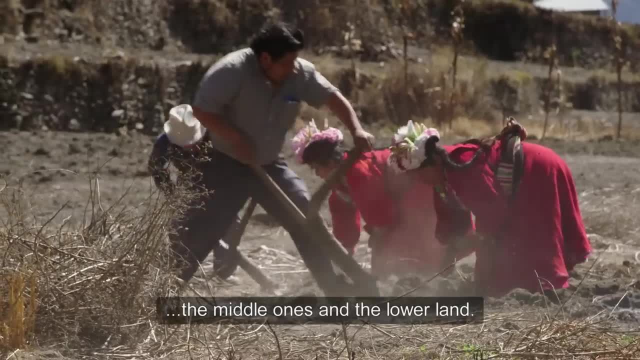 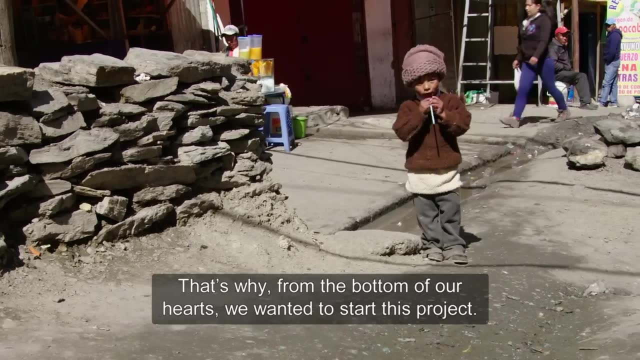 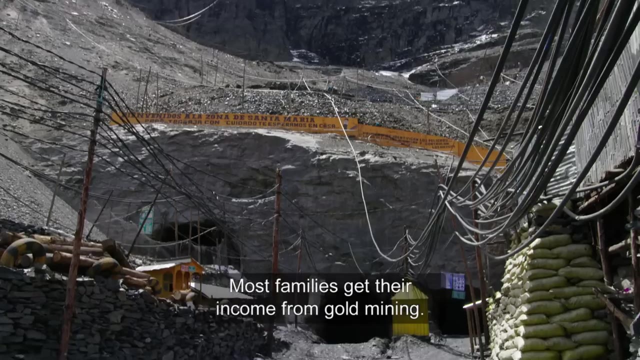 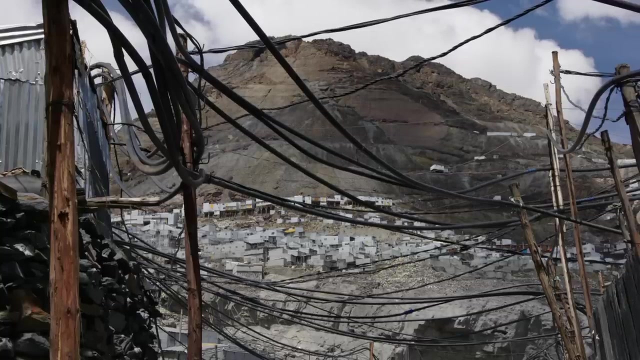 Our ancestors already know perfectly well what to grow in the middle and lower part. So the only income for the families would be the minimum wage. The only income for the families would be mining, particularly the gold in this area. That's where they produce the asphyxia, where they do the gassing. 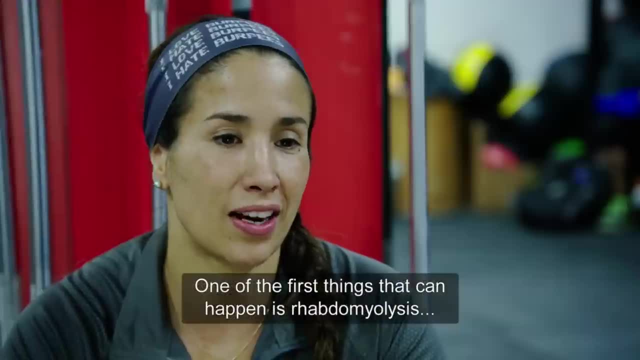 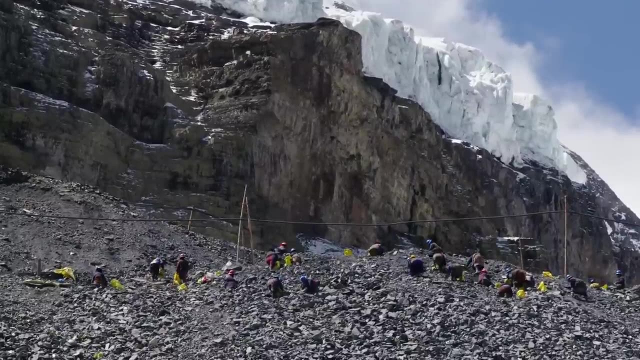 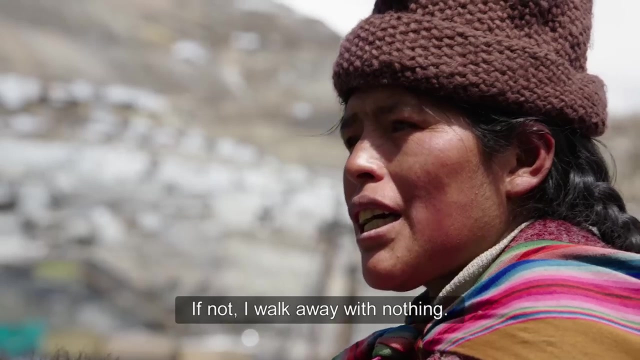 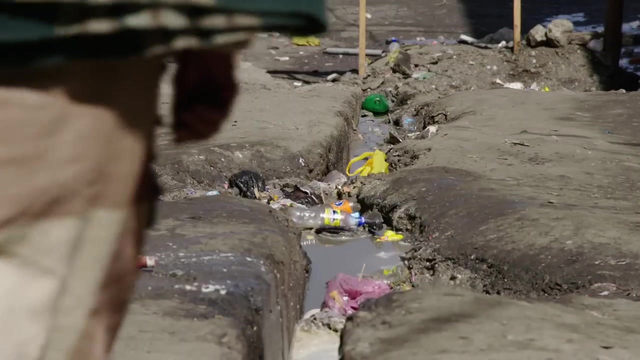 Well, one of the first things that can happen to you is the rhabdomyliosis, which is a physical condition that can lead you to death. How can human dignity survive when the scrabble for gold at the top of the heap becomes a desperate race to the bottom in terms of living conditions, health and safety? 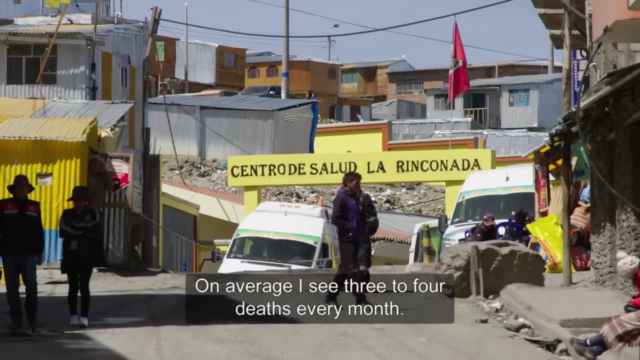 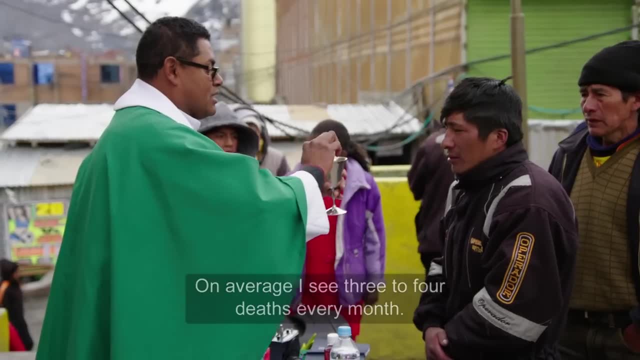 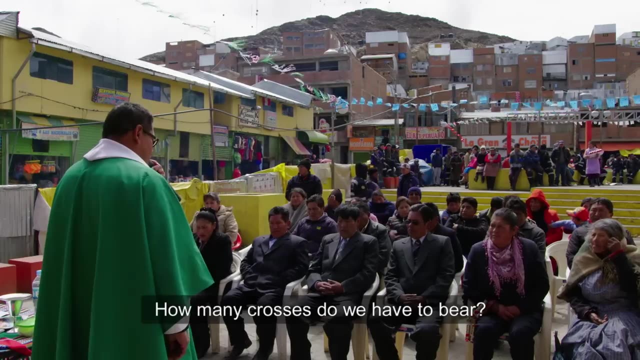 Places where they shouldn't enter. they do Monthly also about three to four people. That's the average death rate per month. And what happens to the human soul when it's driven to such extremes? How many crosses do we sometimes have to carry? 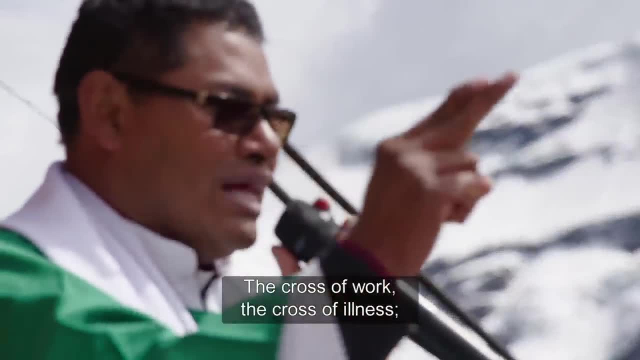 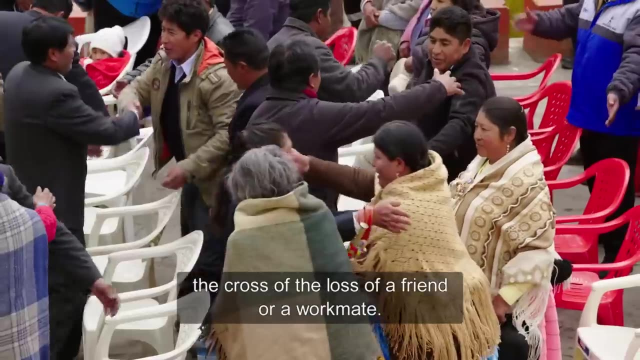 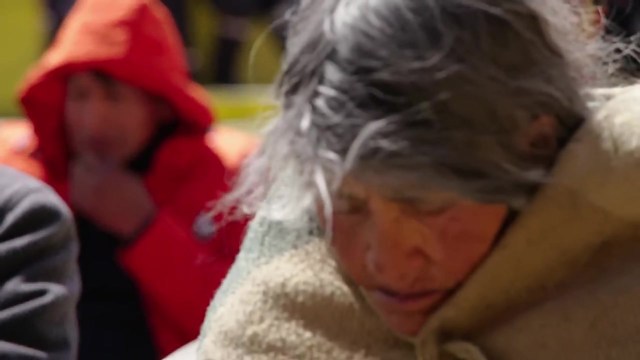 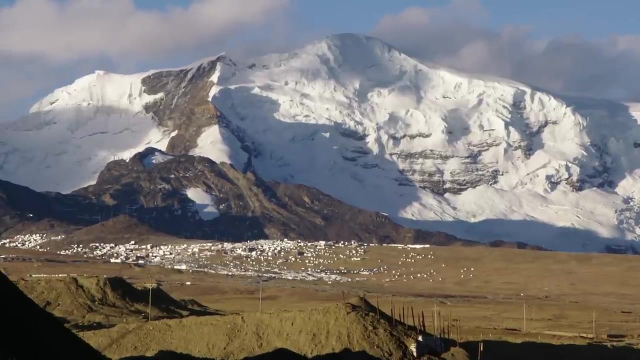 The cross of work, the cross of illness, the cross of the departure of the son or of the partner. This is life in the Andes, At the edge Of human endurance. The Andes are high Due to the bulge straddling the equator caused by the planet's rotation. 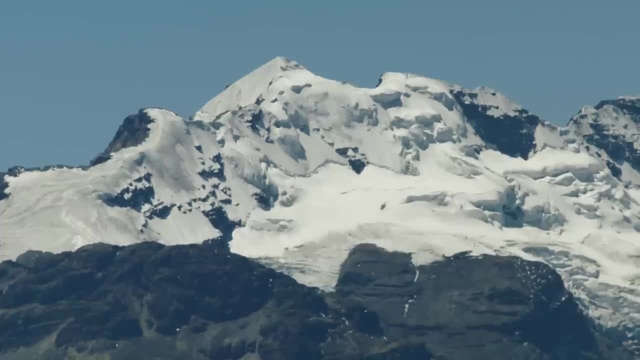 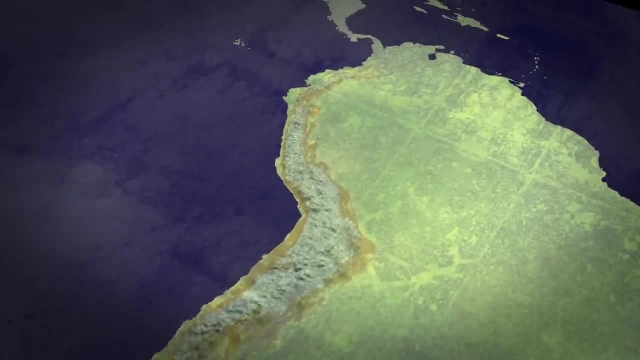 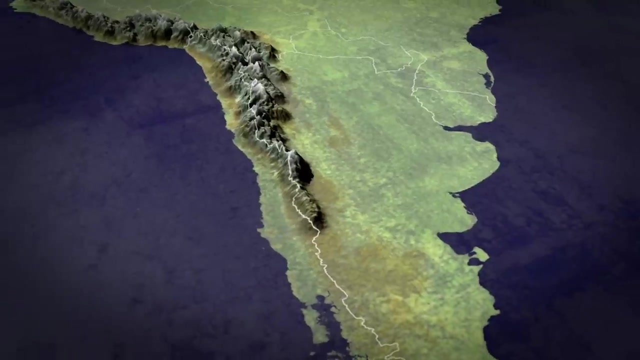 one of the Andean summits reaches further from the centre of the Earth than any other mountain, even Everest. From north to south, the range extends through seven South American countries. On average, the peaks stand a heady 4,000 metres above the sea. 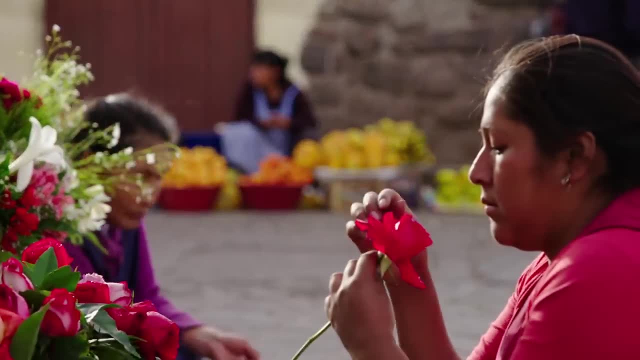 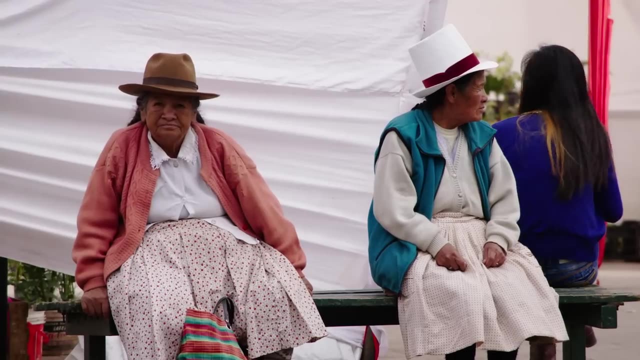 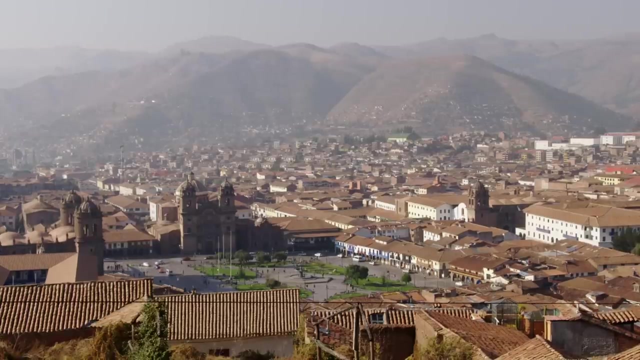 Altitude can do strange and worrying things to the human body. Visitors to this city know that from experience. Three and a half kilometres above sea level, and built on rocks that once lay on the ocean floor, Cusco is a World Heritage Site. 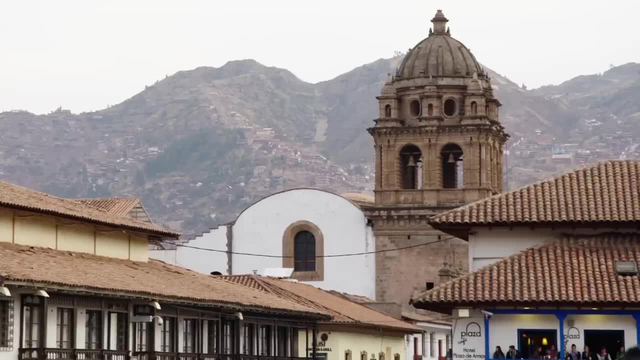 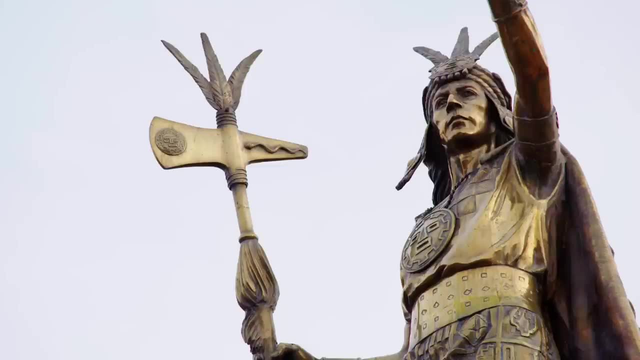 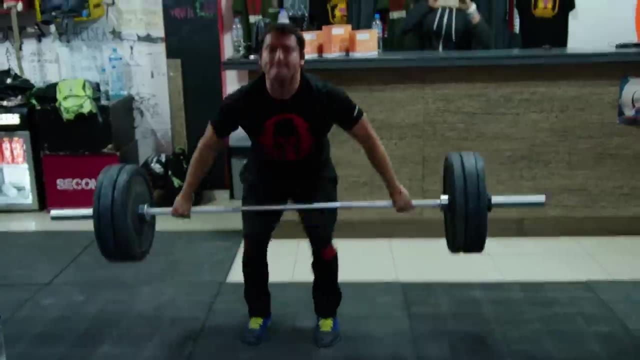 This was the capital of the most powerful indigenous empire ever seen in the Americas: the Incas. By day, Cusco dazzles. At night, it can really take your breath away. Every evening, locals and backpackers come to this gym. 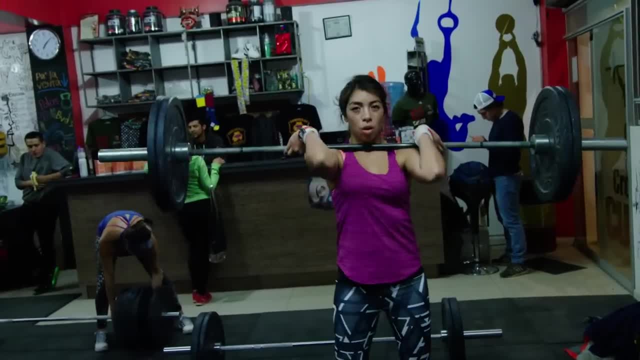 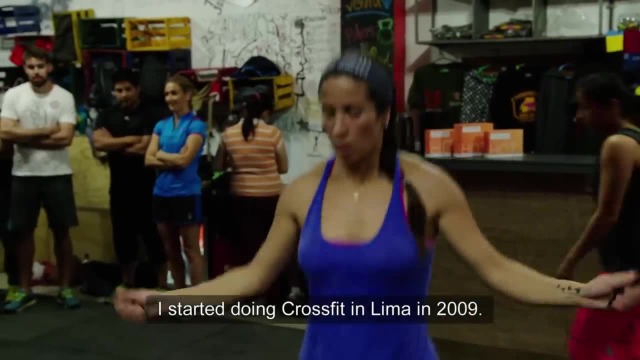 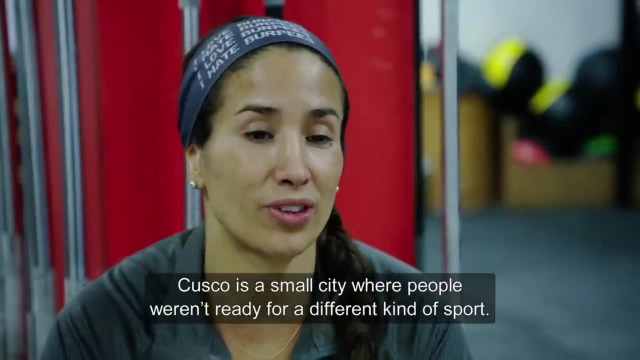 to push themselves to the limit In the name of the latest aerobic craze. I started CrossFit in Lima since 2009.. Cusco is a small city where people were not yet prepared for a different sport, But I came to live here. 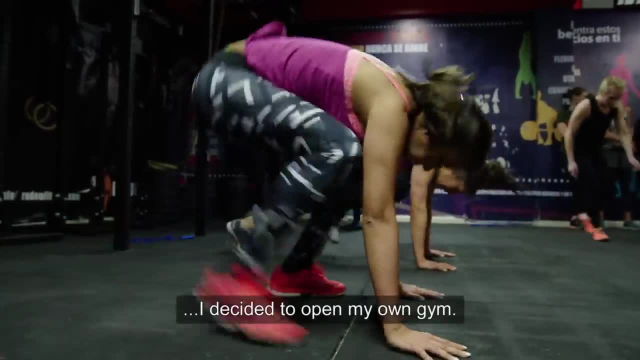 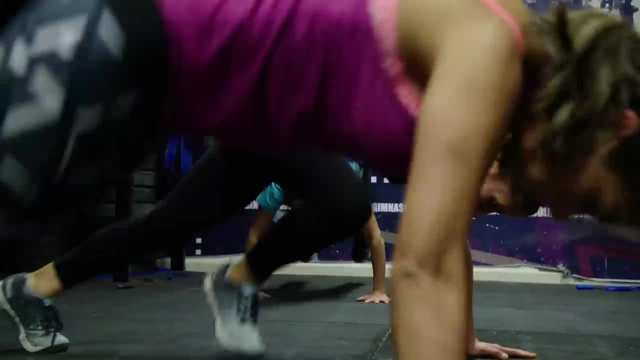 and because of the need for CrossFit in my life, we decided to open a box with some friends. The exercise regime that Briella wanted to share with her new neighbours was a kind of CrossFit, as a kind of cross between gymnastics and weightlifting. 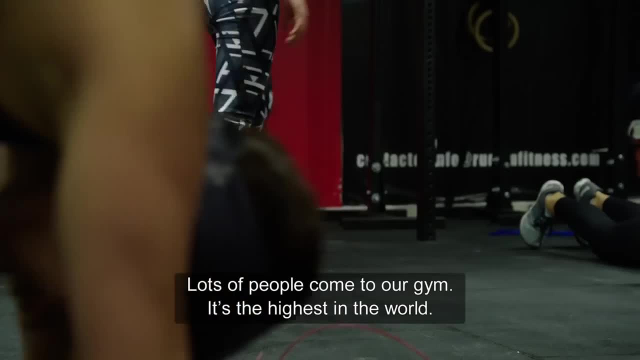 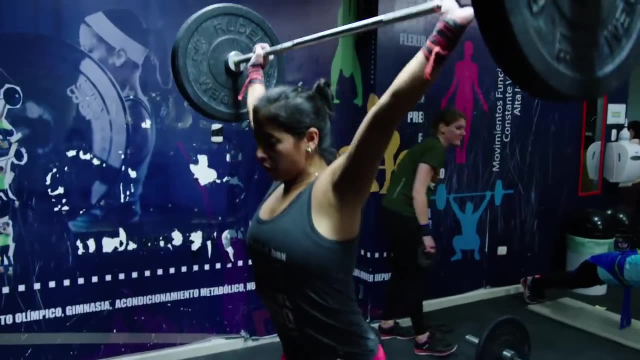 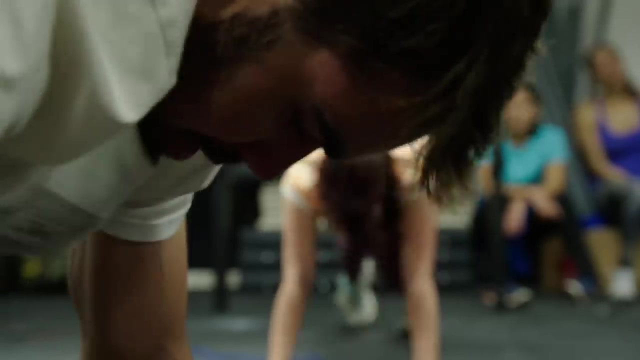 A lot of people come to our box. It's the highest in the world And obviously it's very difficult to adapt to this altitude. For tourists, the altitude only adds to the appeal. It's cool to return home after this session in the world's highest gym, under your belt. 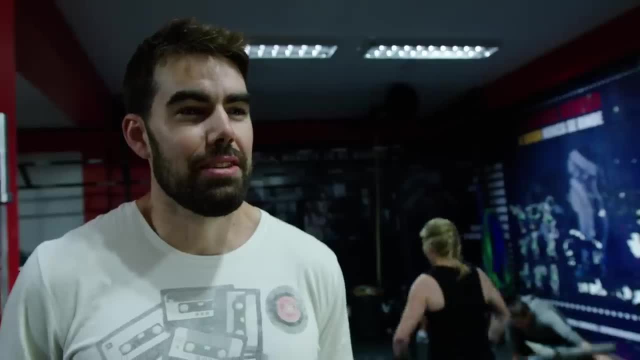 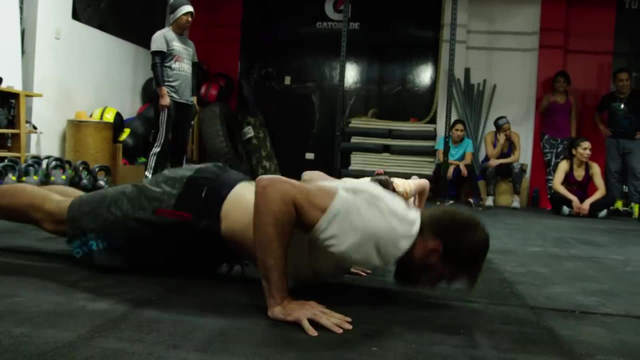 So I'm staying here for two weeks. Today is actually my second one. So I started yesterday with CrossFit And I tried to adapt to the height a little. It's hard, It's tough. You may be fighting fit, but you'll need time to acclimatize to life at 3,500 meters. 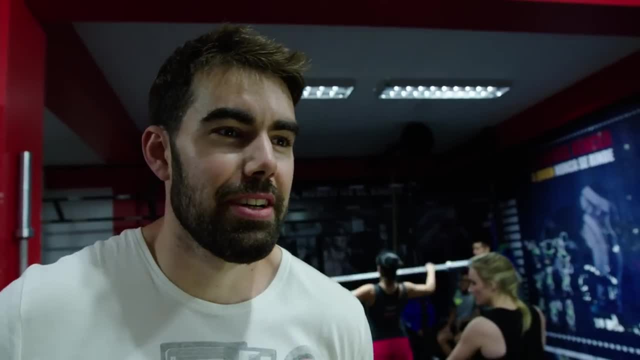 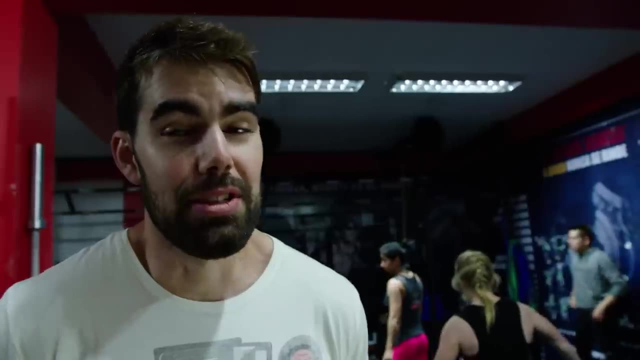 The main problem is probably taking breath. So you really feel it in here that it burns As soon as it inclines or you have stairs or you work out. you'll notice it and it's getting hard to breathe and at some time it starts hurting. 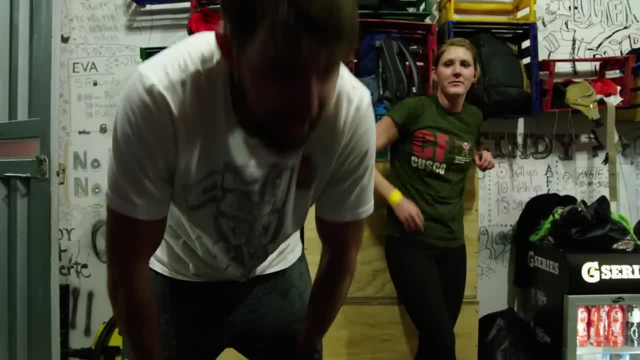 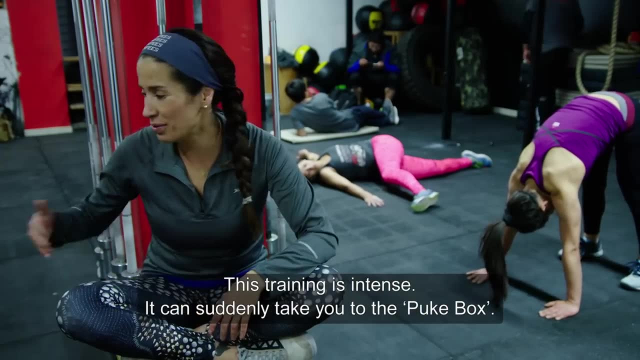 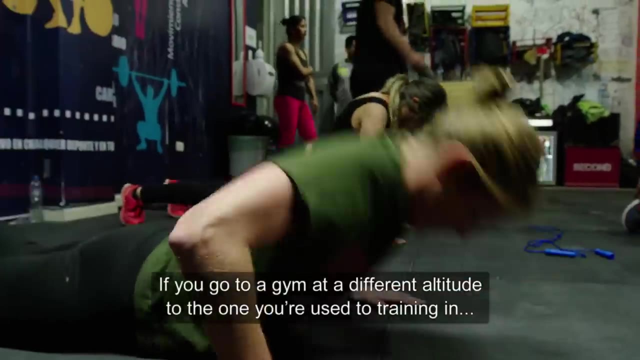 Even the best conditioned clients need to be calibrating their breathing techniques. here in the mountains We know that intensity leads us to Pookie Boxing. Vomiting is unpleasant to move. Other risks can be deadly If you go to a box that has a lot more altitude. 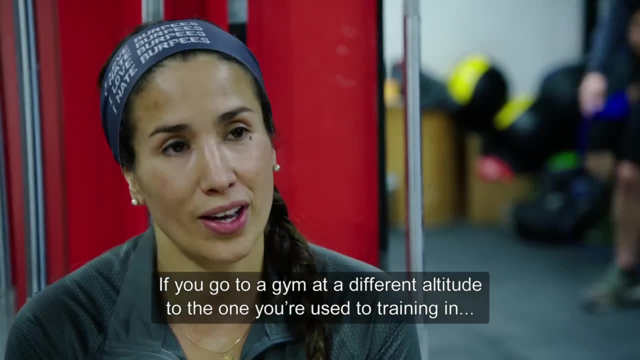 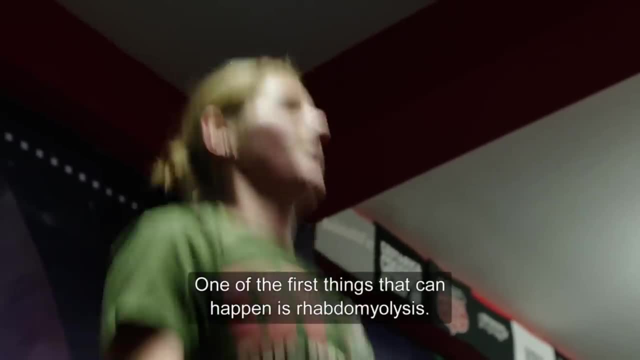 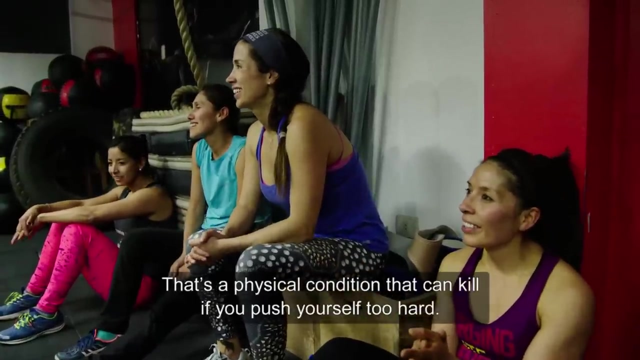 or less altitude and you're used to training at a height, you go to another box with less altitude. it still costs. One of the first things that can happen to you is rhabdomyliosis, which is a physical condition that can lead you to death. 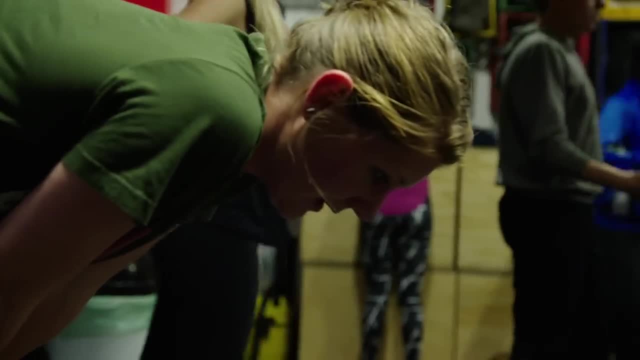 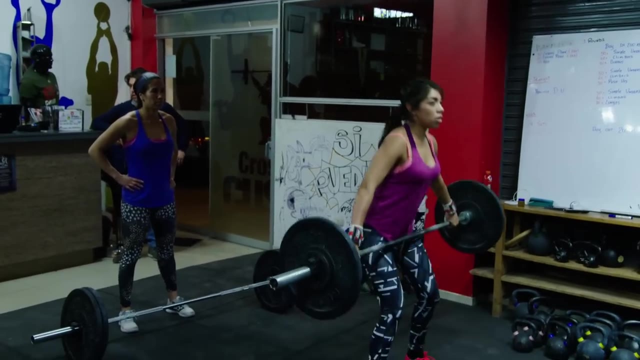 when you demand too much. Cruella's experience is that the effects are unpredictable. This high up, there's no knowing which of the gym's disciplines the customers will find most challenging. It's been a little hard for me. the issue of muscle strength. 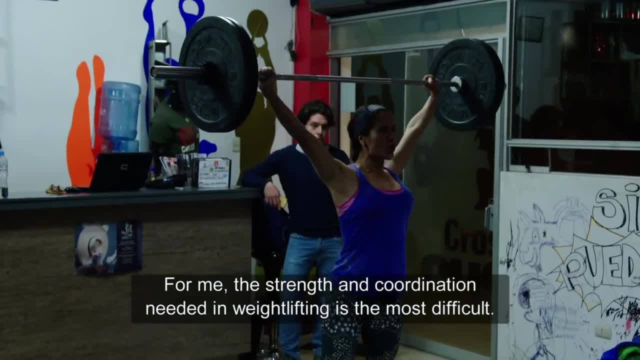 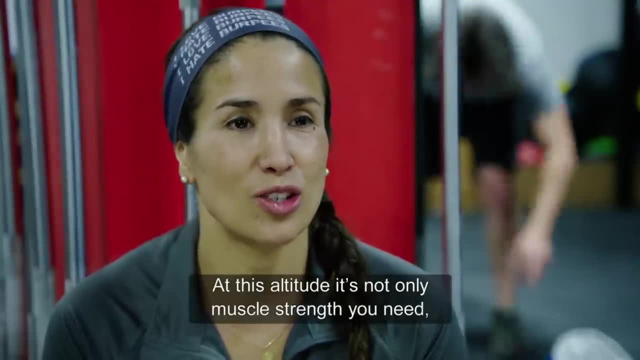 to do Olympic lifting because it's a lot of coordination, a lot of muscle strength. Exactly That's been my difficulty, And this height, in any case, is not only the strength but also the cardio that you use when you do lifting. 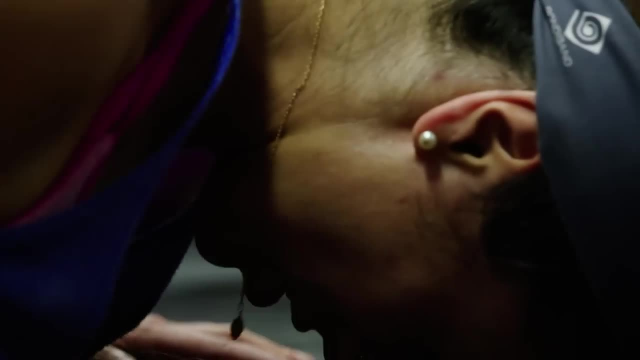 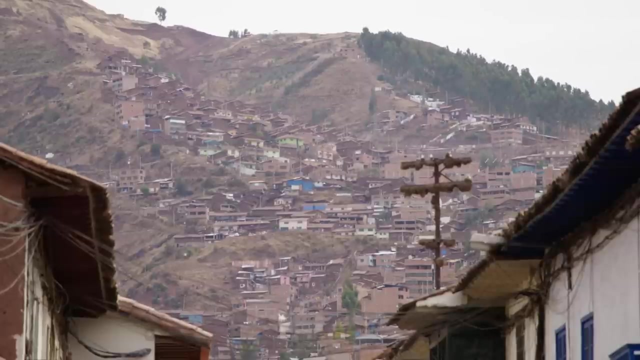 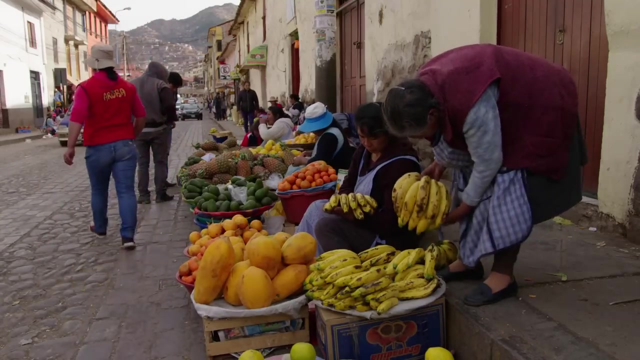 That's been my difficulty. You can't escape the effects of geography if you live in a city like Cusco, But there's no getting away from history either. Just as the crash of tectonic plates forged the geology of the Andes, 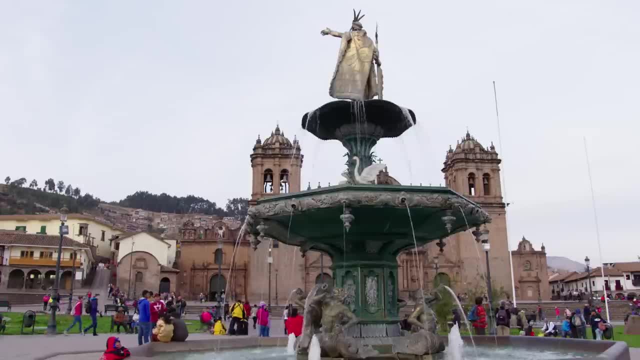 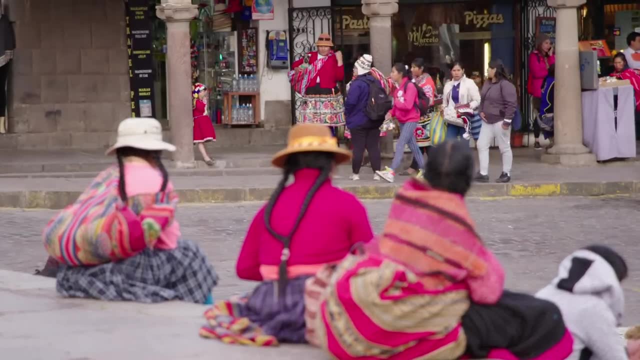 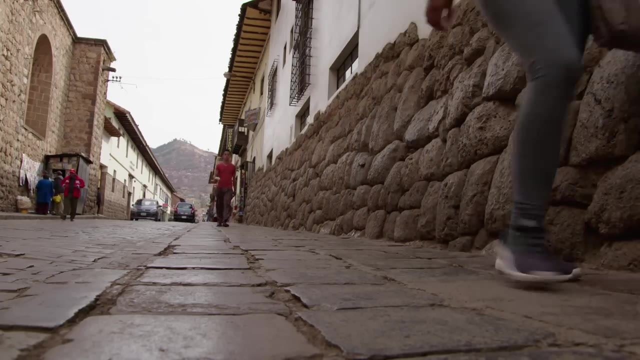 the clash of two civilizations has shaped the backstory of everyone in these mountains. Look more closely at the streets of Cusco and you can see the strata of the two cultures sitting literally one on top of the other. The foundations of the old Inca capital are still here. 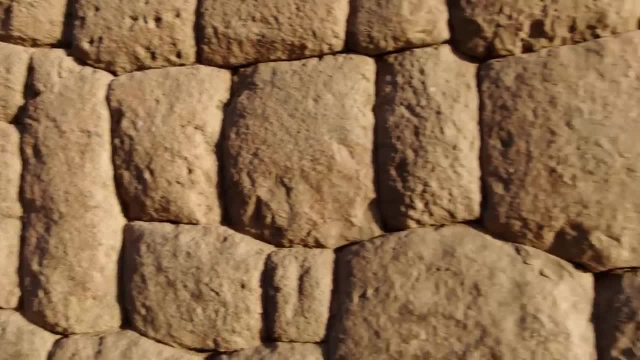 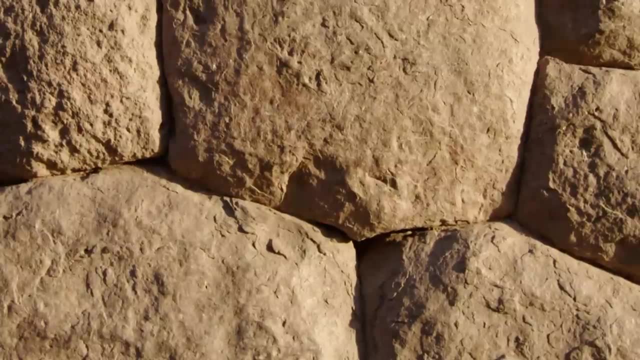 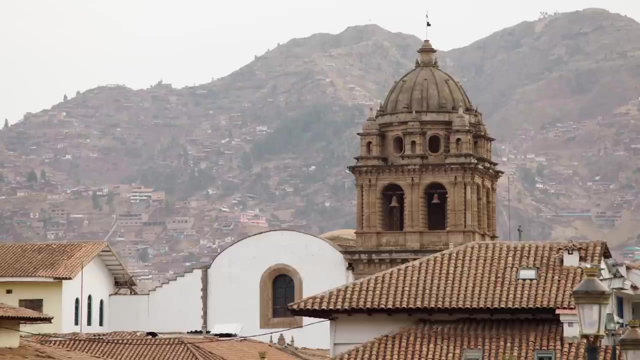 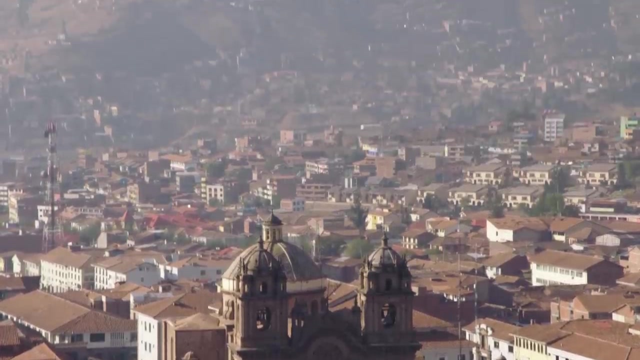 Every stone individually shaped and fitting perfectly into solid walls which still mystify archaeologists with the skill of their construction. But above them are the colonnades and terracotta rooftops of the Spanish conquistadors. The Spanish may have conquered by military might. 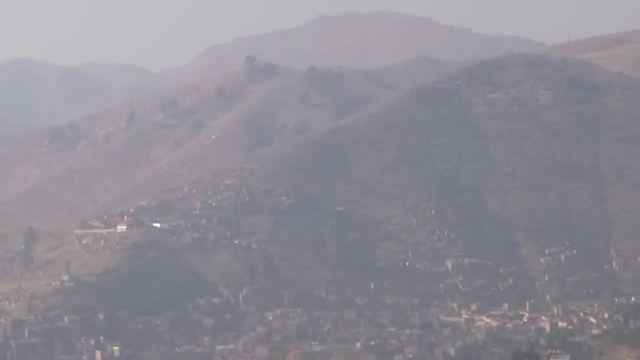 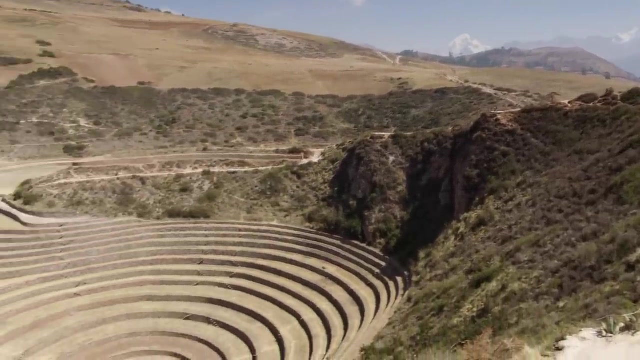 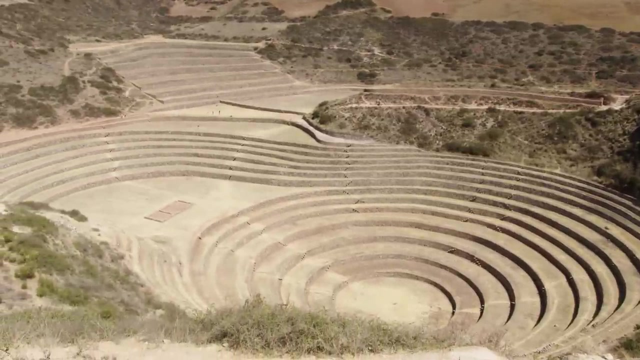 but it was the Incas who were the true masters of high-altitude living. This site, Moray on the edge of Cusco, is proof of that. The people used to think that it was an amphitheatre because the steps and the circular shape. 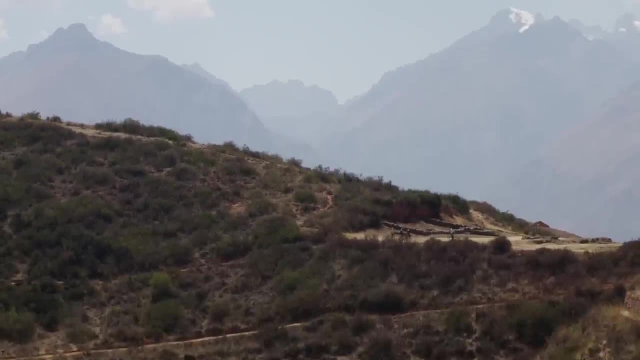 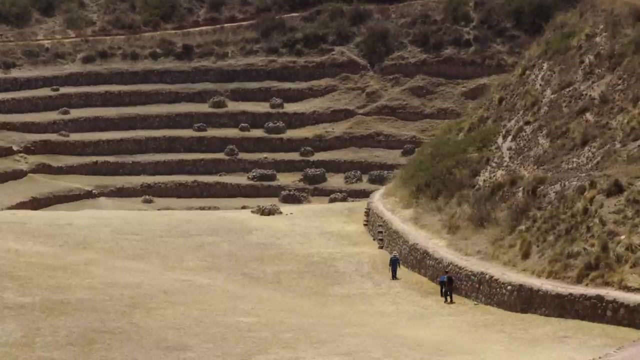 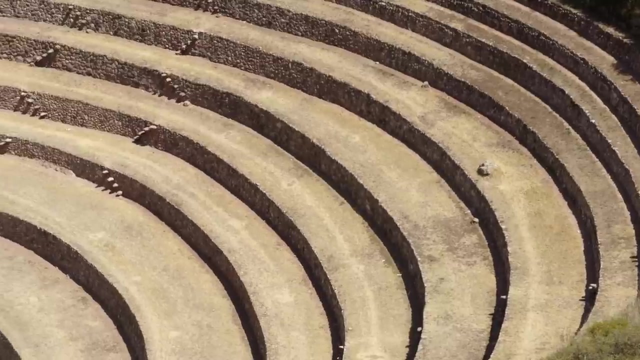 Detailed archaeological investigation uncovered the true nature of this hollow in the landscape: It was a natural depression. It's a natural formation. They took advantage of that and, according to the natural formation, they started building the terraces in a round shape. The terraces were actually part. 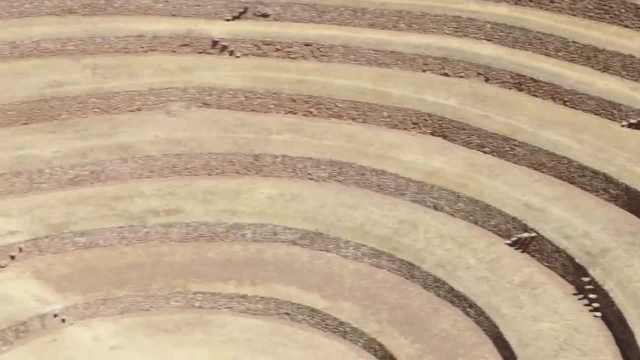 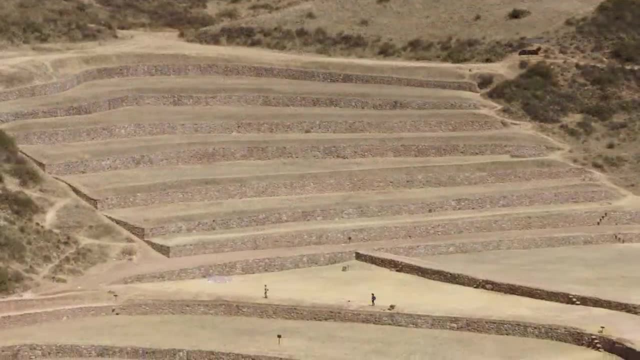 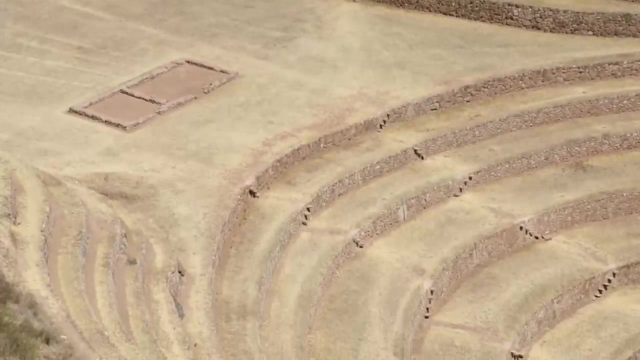 of a huge agricultural laboratory. One of the site's most remarkable design features is the large temperature difference between the top and the bottom terraces- as much as 15 degrees Celsius. The microclimates created allowed the Incas to experiment to find the ideal growing conditions. 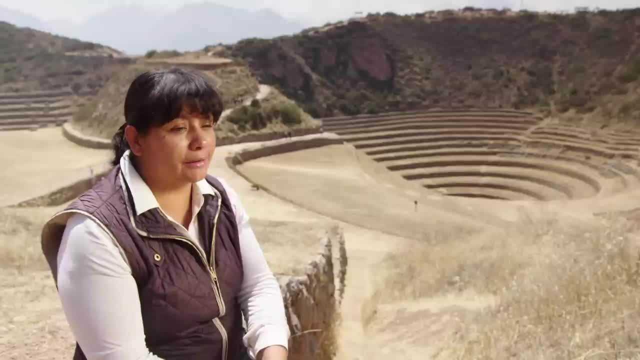 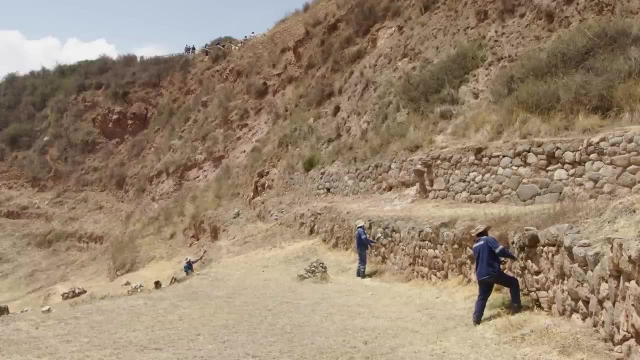 The high priest, astronomers, the leaders, the people that organized them was a kind of a secret group. This elite was able to learn which crop varieties grew best at different temperatures in the soils found across a wide swathe of the Andes. 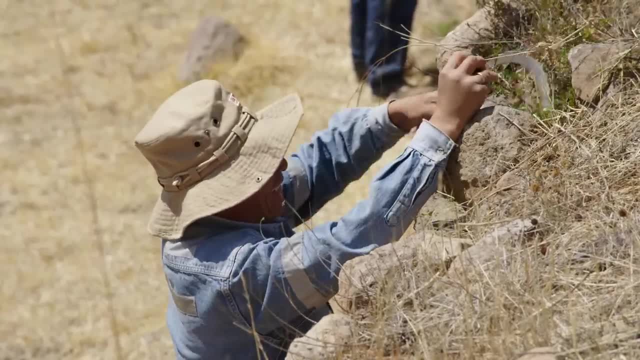 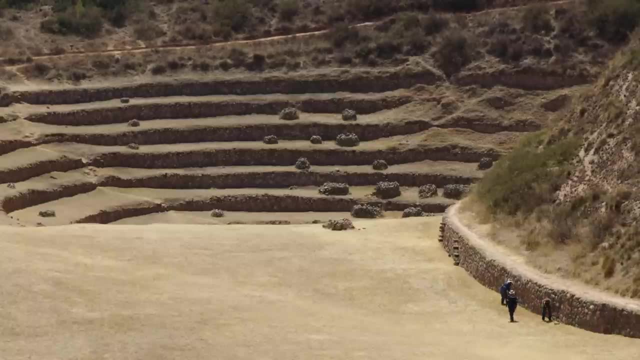 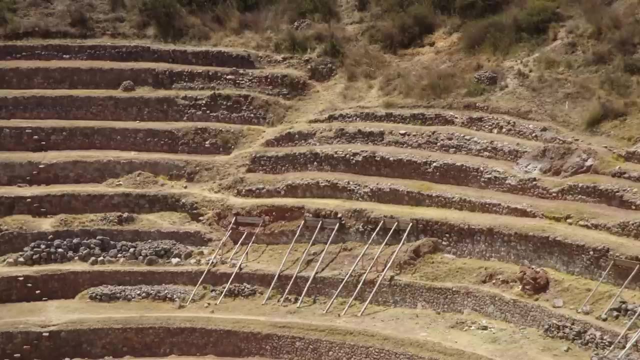 And Moray was their mission headquarters, So they sent their technicians, astronomers, engineers to faraway places to make studies. In that way, they used this place as an important experimental center to adapt and breed the crops like corn potatoes, squash beans and grains. 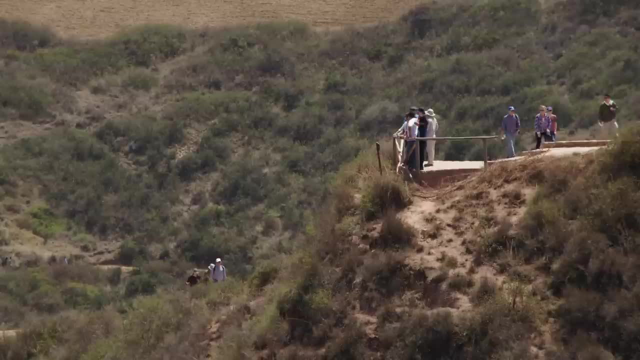 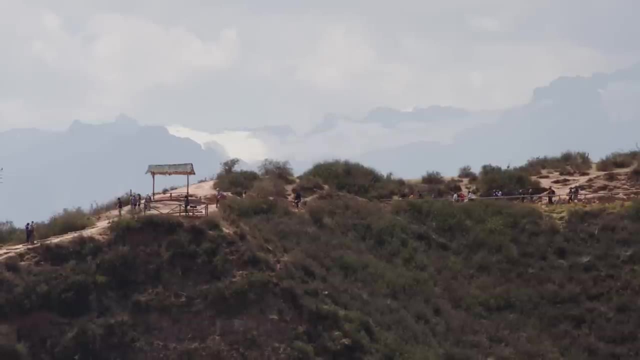 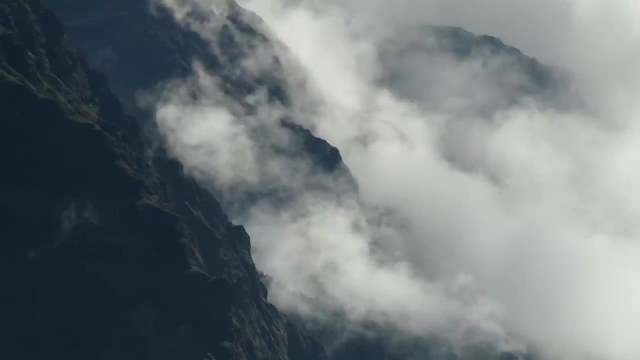 The impressive roster of produce remains important to this day. It's said that 60% of the world's food crops originate from plants grown in the Andes. Some of them would have been cultivated right here. Moray is the only place in the world. 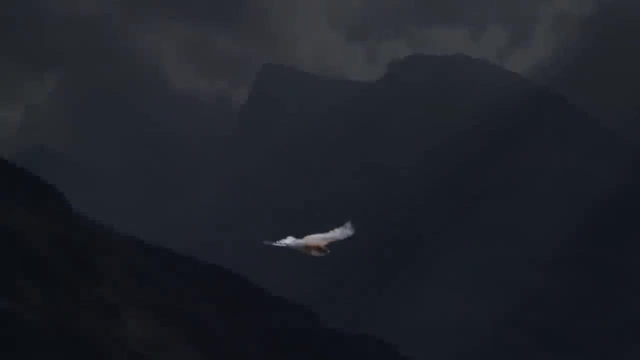 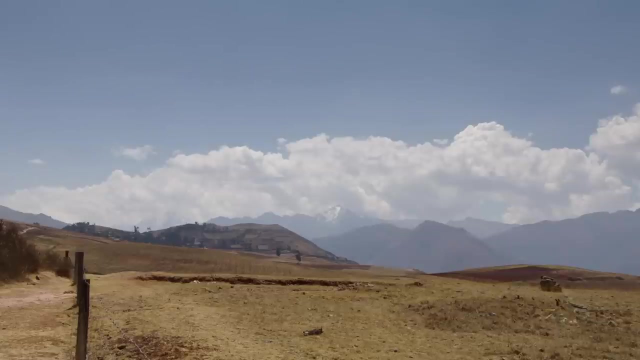 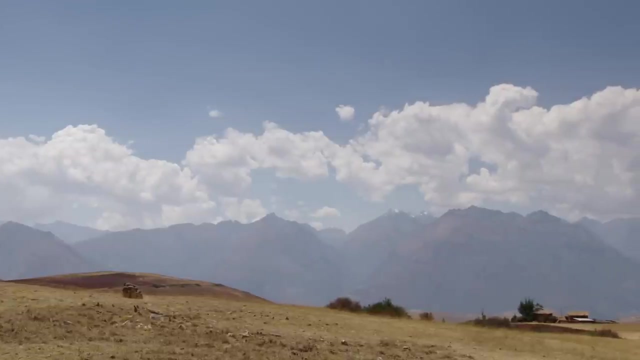 where the Incas lived. Moray is the only place in the world where the Incas lived. The secrets of Moray helped the Incas keep their grip on a vast empire. Their success in turning the high plains into fertile ground didn't go unnoticed. 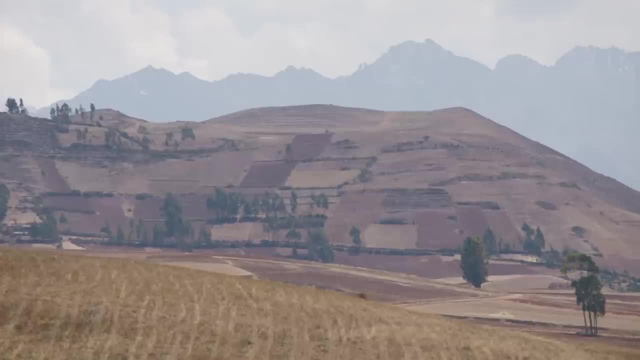 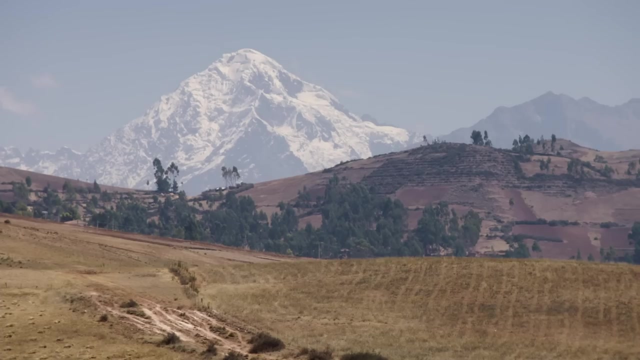 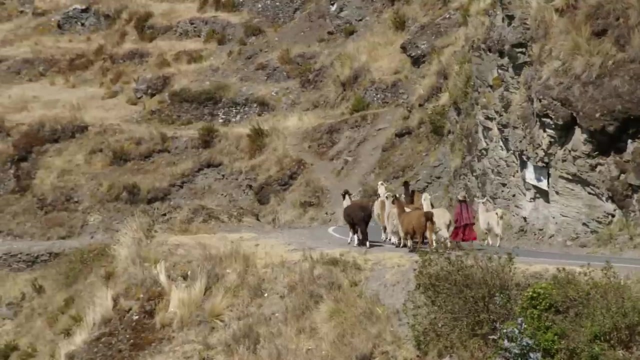 when the conquistadors stormed the Inca citadels, Spanish eyes looked with envy at the prime agricultural land. Spanish might swept the Incas away from it. The natives were forced to move even higher up the mountains, so high that farming seemed impossible. 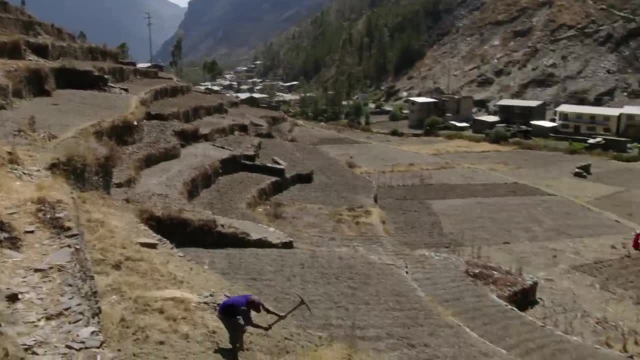 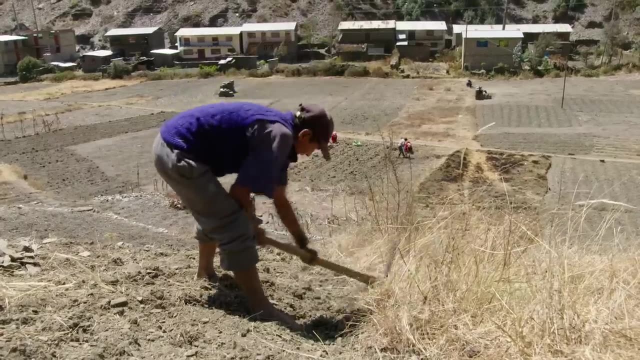 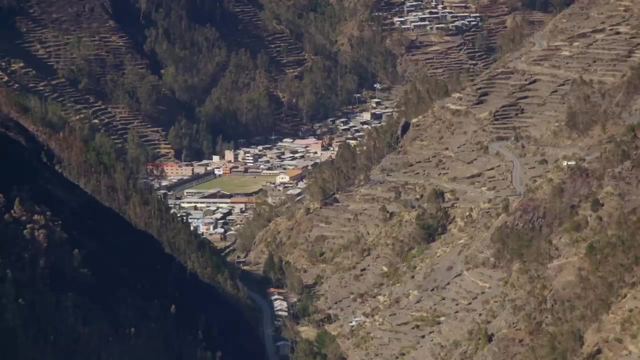 And impossible it may have been to all but the Incas. Today, centuries later, evidence of their ingenuity is still to be seen If you travel high enough. Surrounded by 5,000-meter peaks, this is the valley community of Cuyacula. 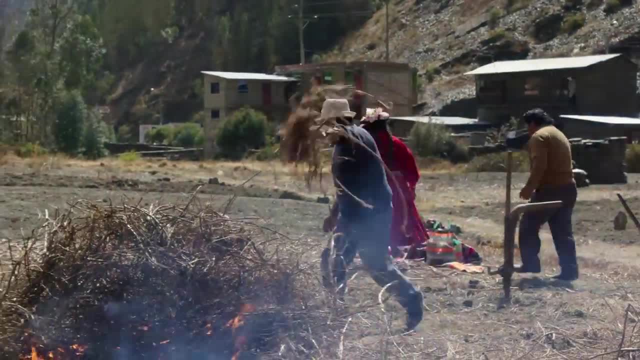 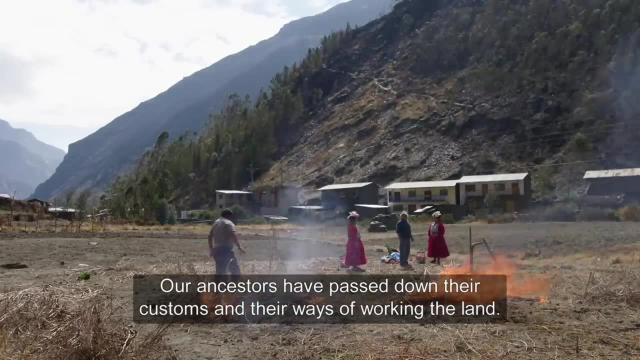 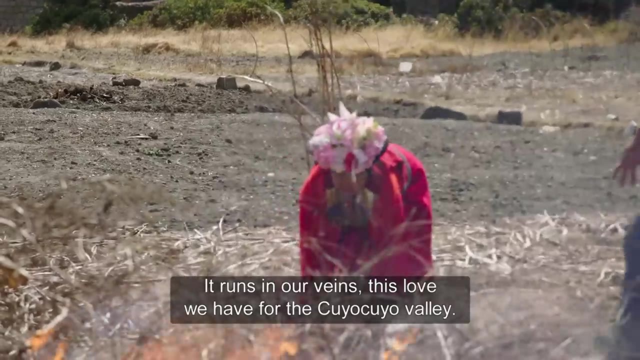 The legacy of the Incas has never quite been extinguished here. Our ancestors seem to have inherited us with the customs, with the work of the land. It circulates in our veins that affection, that love that we find in this Andean trapeze. 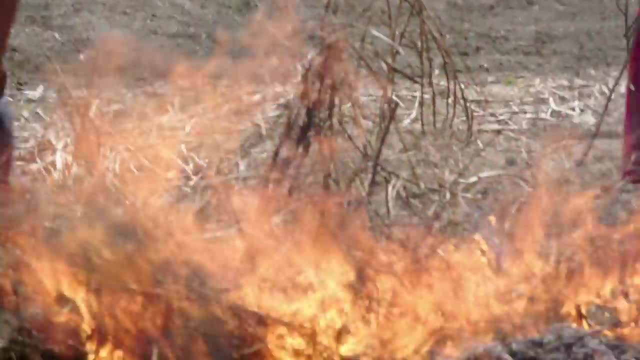 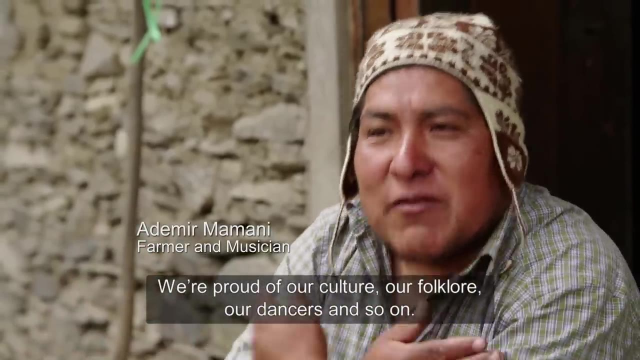 which is our district of Cuyacuyo, And we are proud of our culture, our folklore, our dances, etc. So we are satisfied with what our ancestors have inherited us with Ademir. Mamani is a man of many parts. 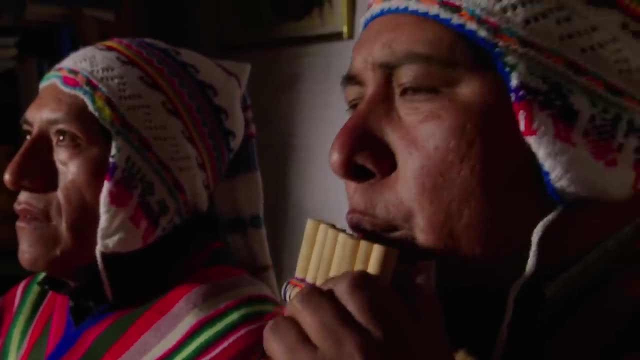 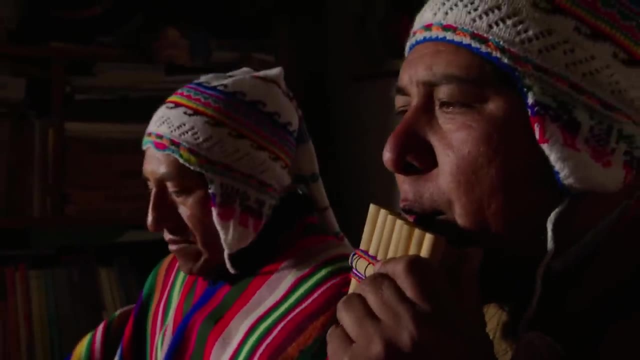 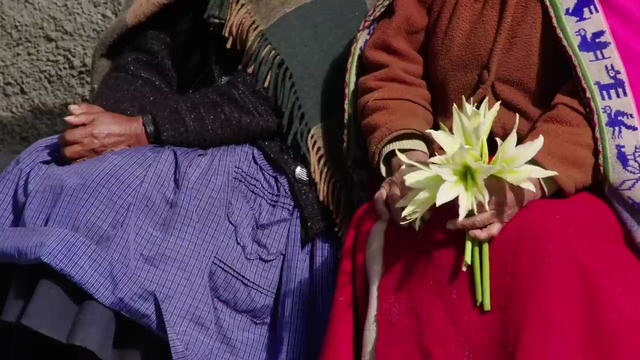 Musician, farmer teacher. When he's not in the classroom or the fields, he loves to practice playing the siku or zampoña, an instrument as traditional as the region's colorful costumes, Nowadays the distinctive music of the Andes. 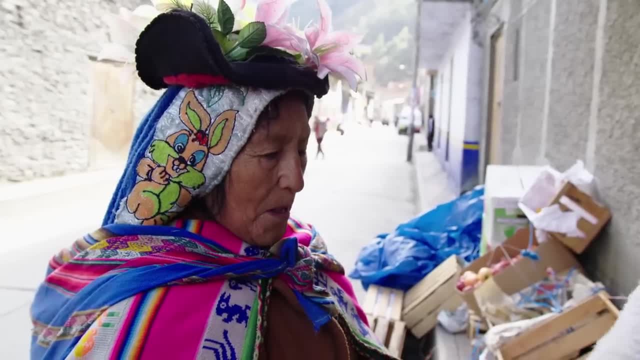 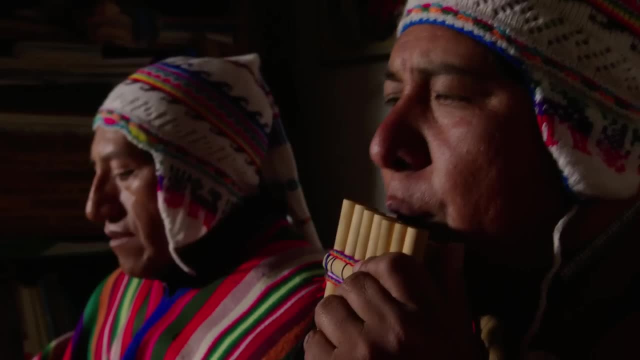 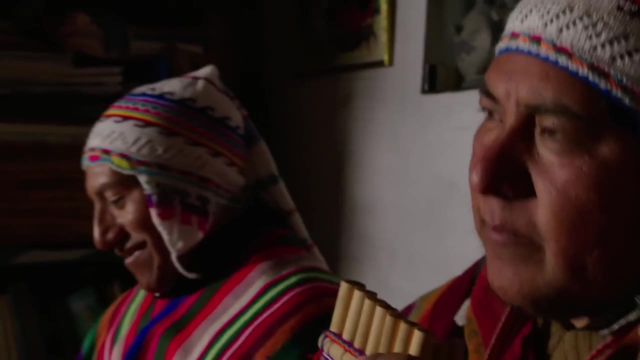 is a familiar sound all over the world. Here it's close to its roots, Played as an expression of human emotion, but also as a peace offering to the presiding local divinities. For these mountain people, pleasing the gods has always been crucial. 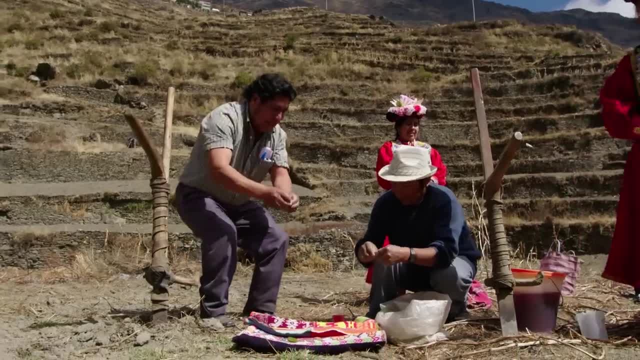 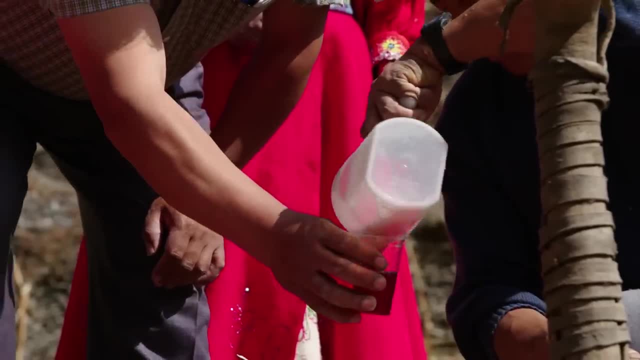 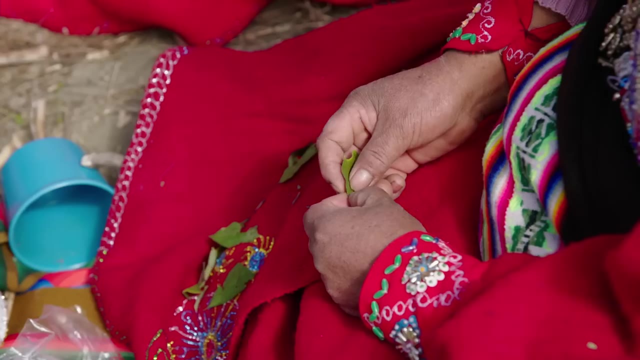 to their very survival. Before planting or harvest, they make an offering to Pachamama, Mother Earth. It's a ritual which has been observed here since humans first shaped this landscape for agriculture. Seeing the andenes, the constructions, that is the construction of the Andes. 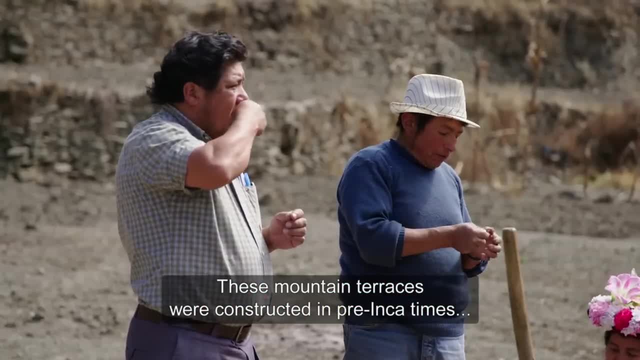 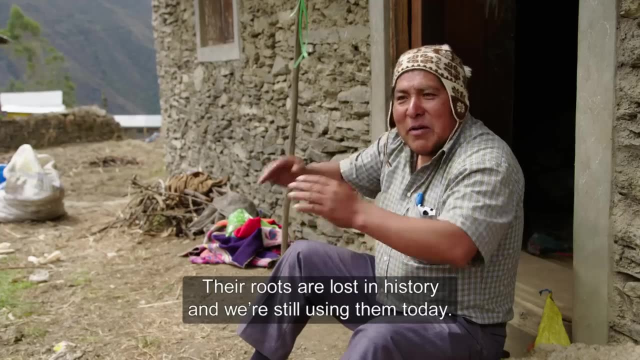 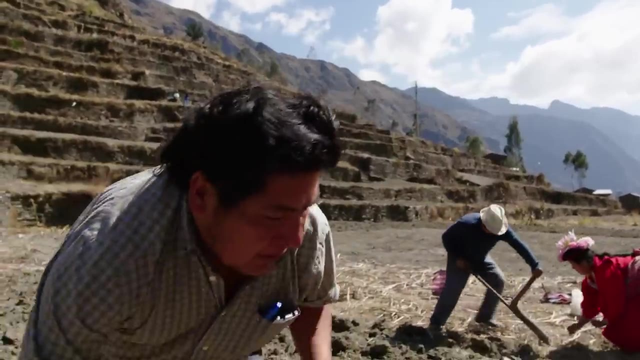 The construction of the Andes is of pre-Inca and Inca-Inca times, So that's also lost in history. but it's still maintained and it's as we can observe. Nothing can guarantee a love for harvest Agriculture. here is a risky business. 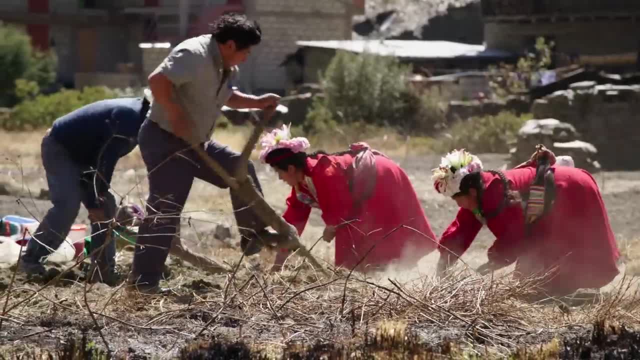 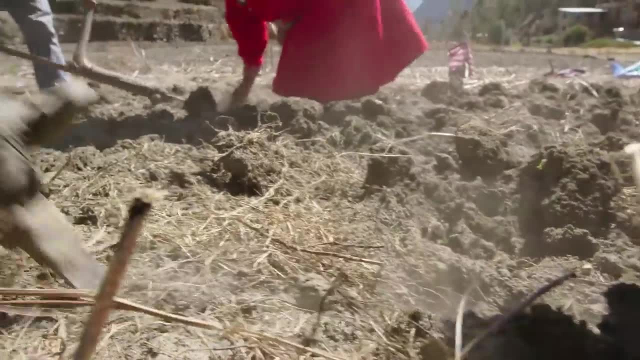 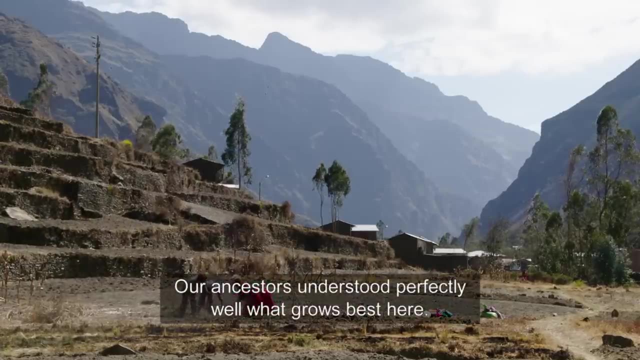 But as well as a little sympathetic magic called down from the heavens, Ademir and his family can draw on many generations of experience in conjuring the best possible results in this challenging planting environment. Our ancestors already know perfectly well what to grow in the middle and the lower part. 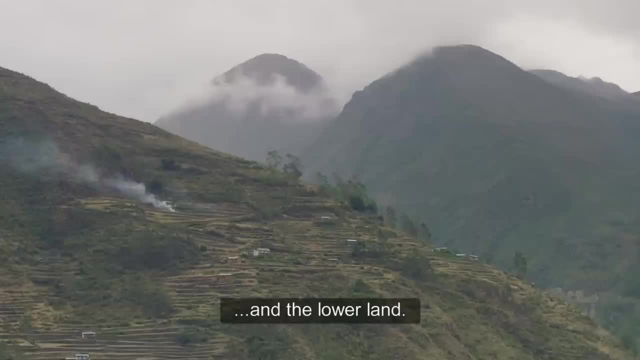 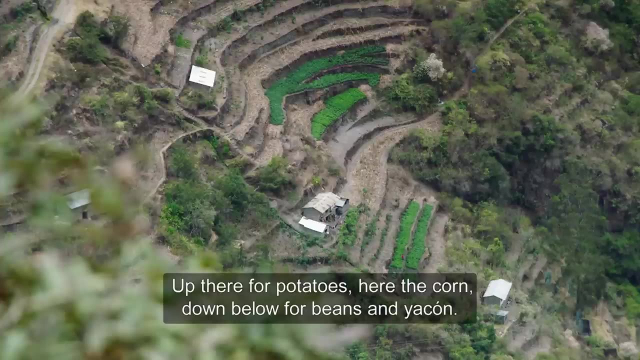 So they know the soil, what it will produce in that place. So they already know this is for the potatoes, for the corn, for the grapes, for the yacon. They already know they have developed a lot, our ancestors, in that aspect. 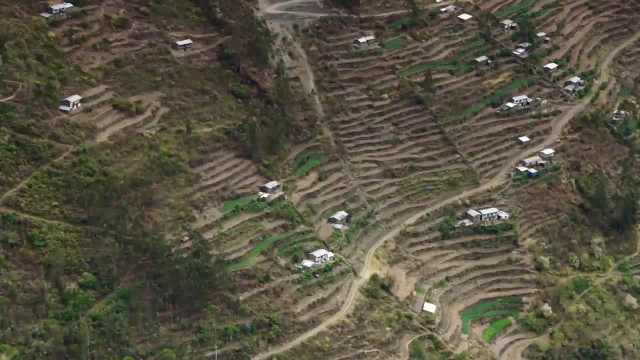 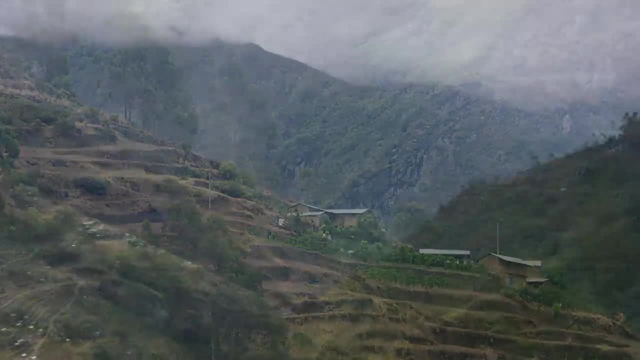 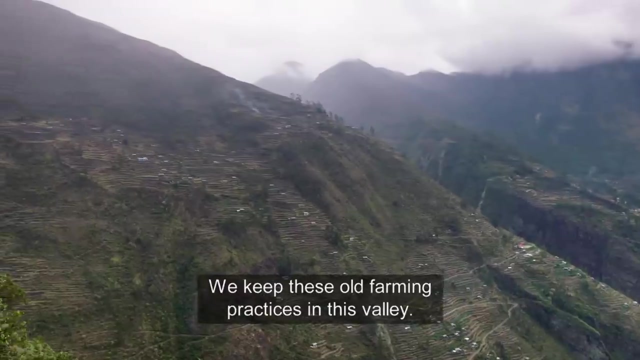 The Inca heritage offers farmers here some insurance against hunger. It's not just ruin. If the crops fail on one terrace, another, with different levels of exposure to wind, sun and rain, may well prove fertile. All this practice of cultivation of these products of this valley. 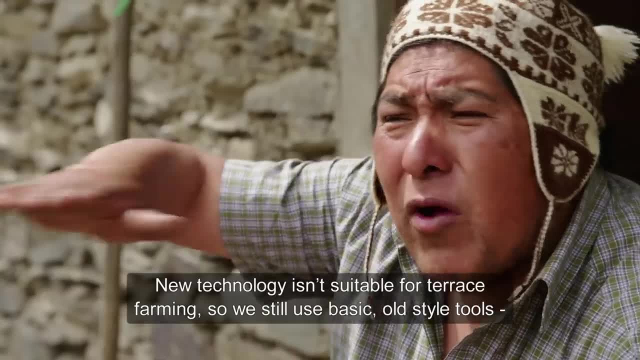 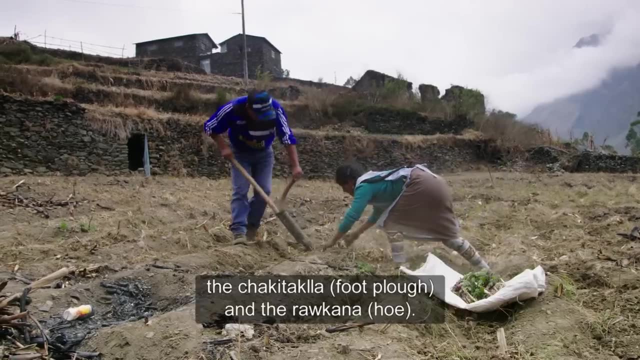 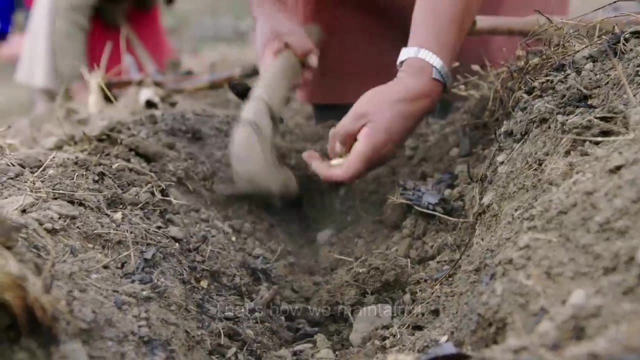 is still maintained. For example, it is not favorable for the dams, the terraces, for the technology, for the technification. It is still maintained with rudimentary tools such as the chaquitaclia, the chavana, Here on these remote eastern slopes. 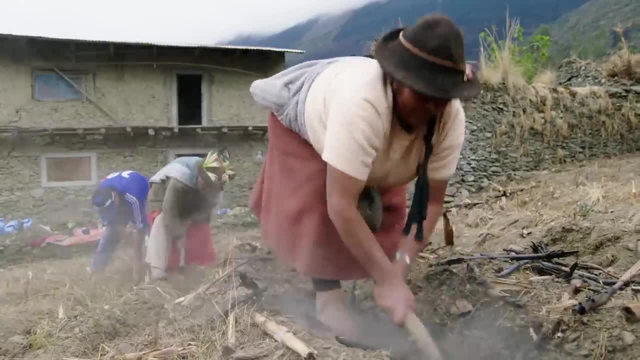 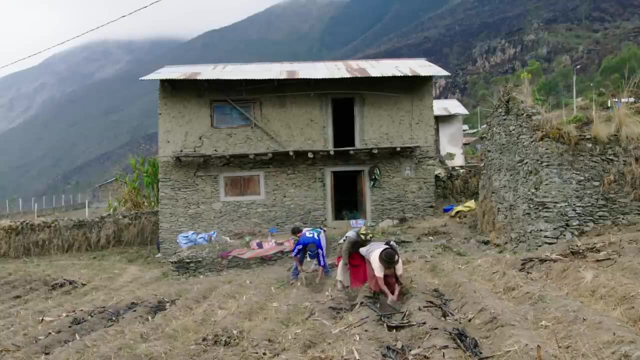 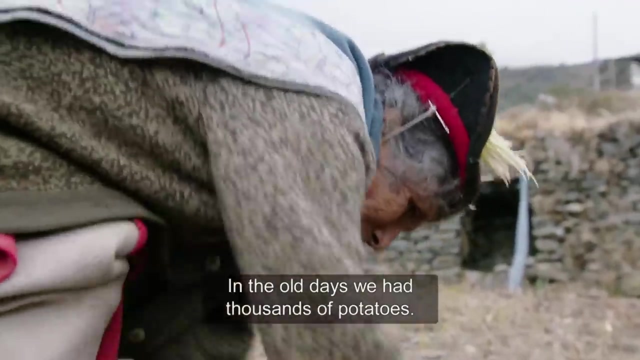 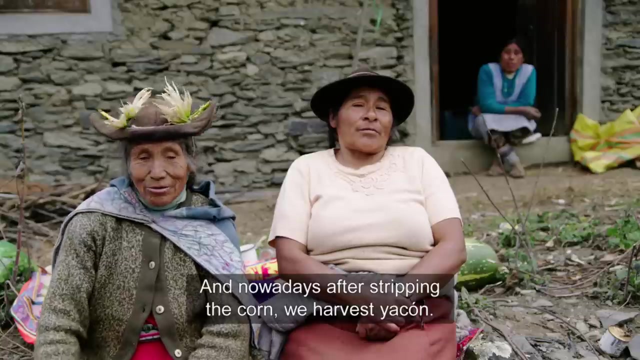 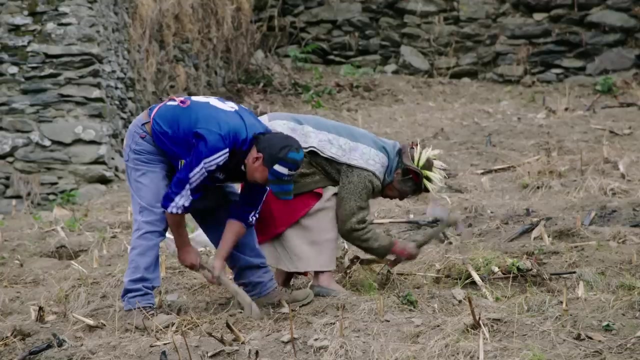 of the Andes, the sinews of communal life are holding together somehow, But they're fragile and highly dependent on these traditional forms of agriculture. As in so many other mountainous parts of the world, the older generation is seeing its young people drawn away. 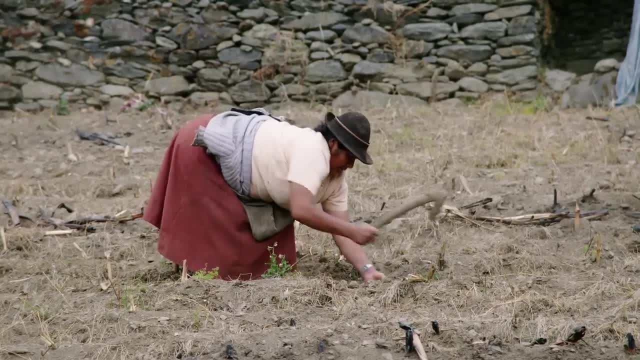 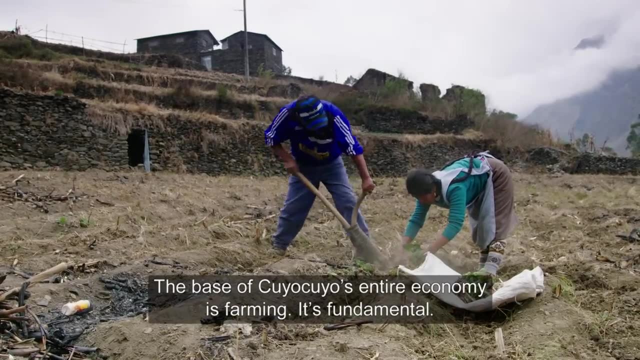 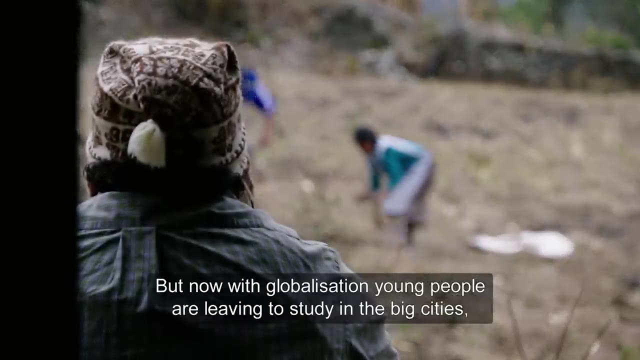 by the bright lights and more secure prospects of the city, leaving only a kind of nostalgia for the way things were. The fundamental base of the economy is agriculture. It is the fundamental base. So now, with the migration, with globalization, it is also being left a little. 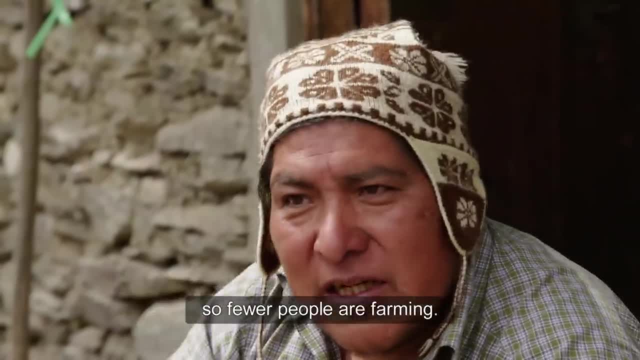 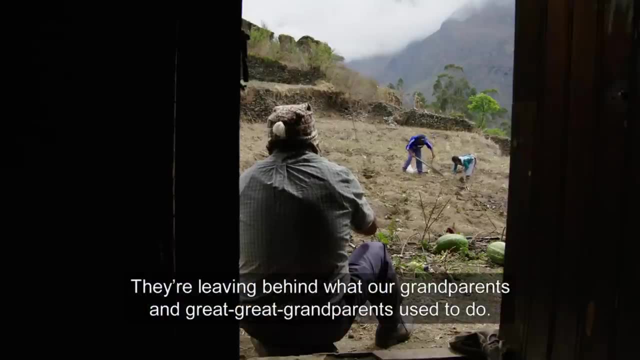 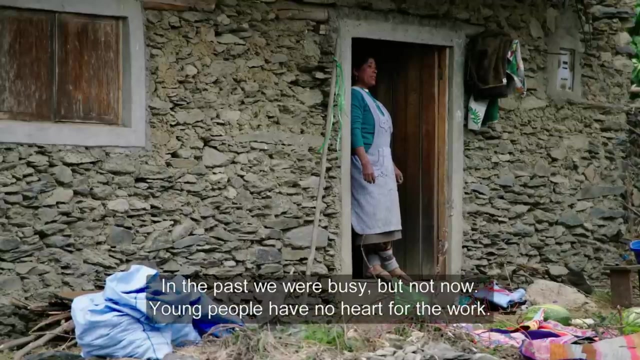 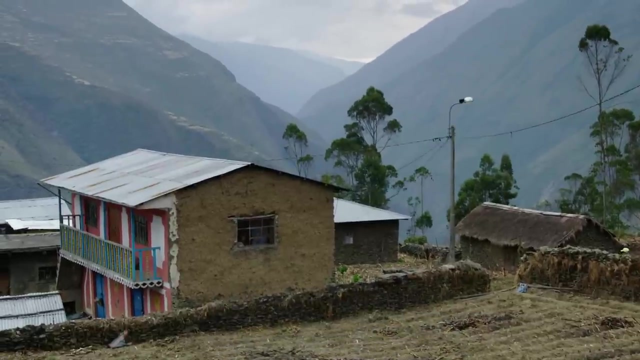 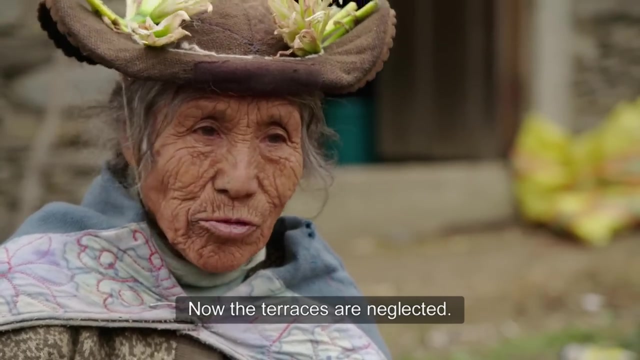 because the young people, the old people are going to the big cities. So our ancestors, our grandparents are still there, but they want to stop it a little. We have to make sure that we don't have to go back and forth. 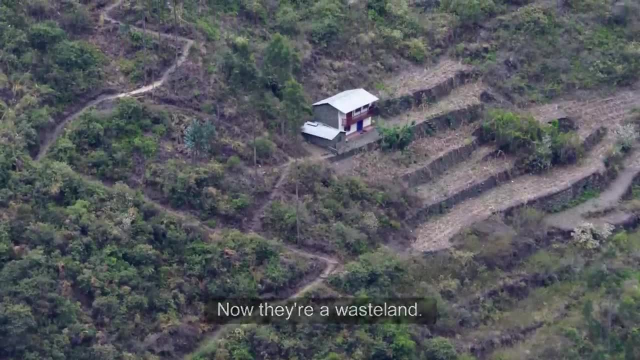 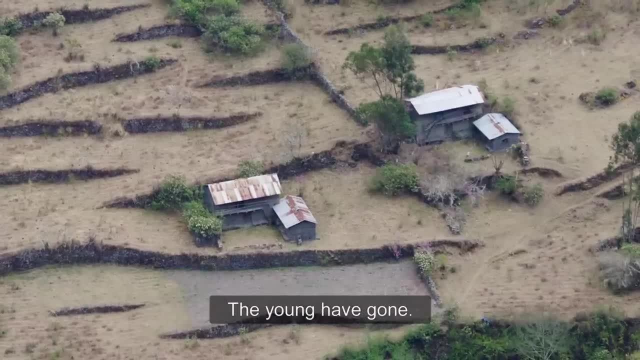 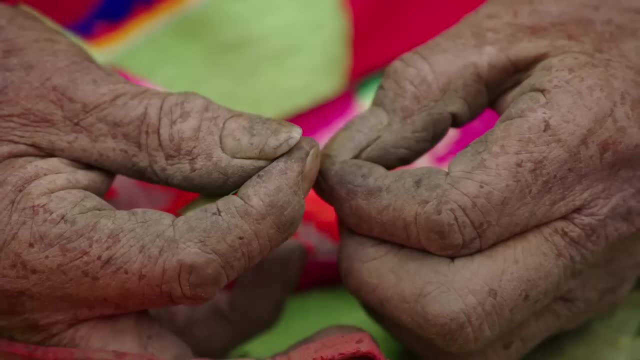 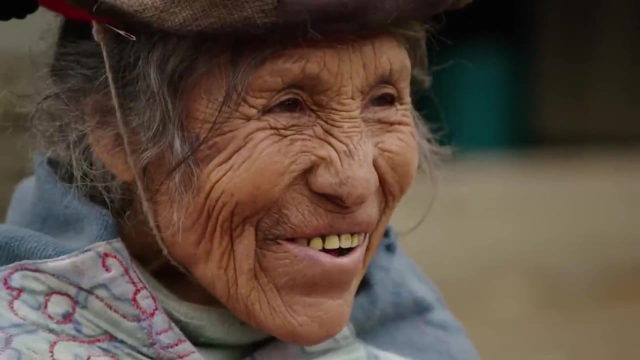 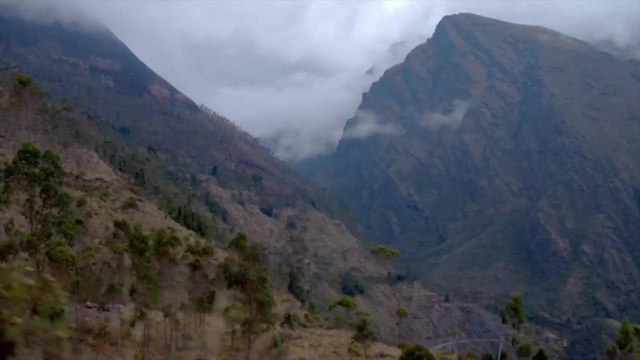 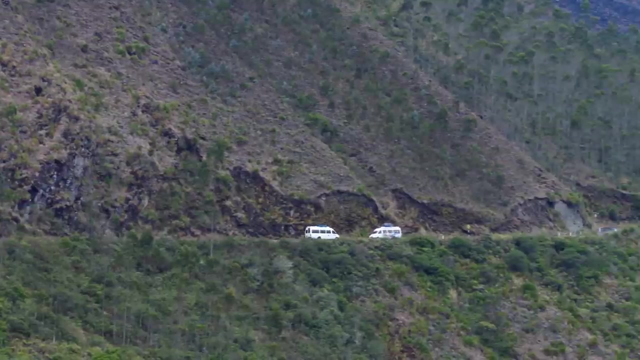 We have to make sure that we don't have to go back and forth. We have to make sure that we don't have to go back and forth. Onwards from Kuyokuyu, the road climbs perilously up the steep-sided valleys. 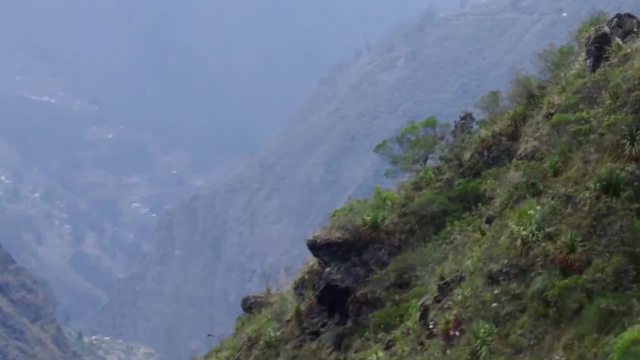 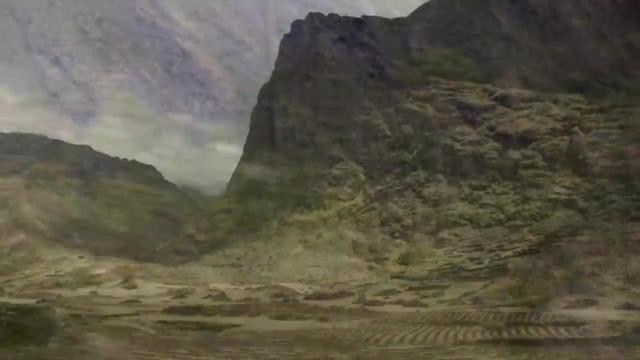 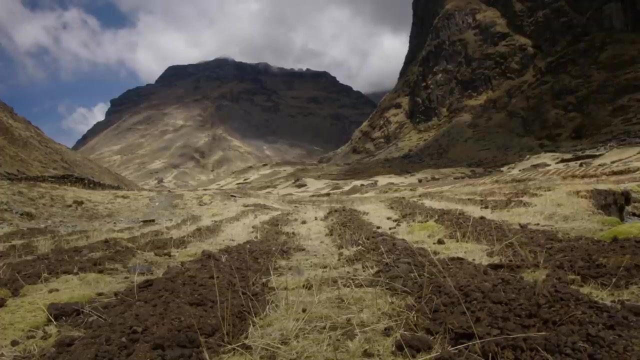 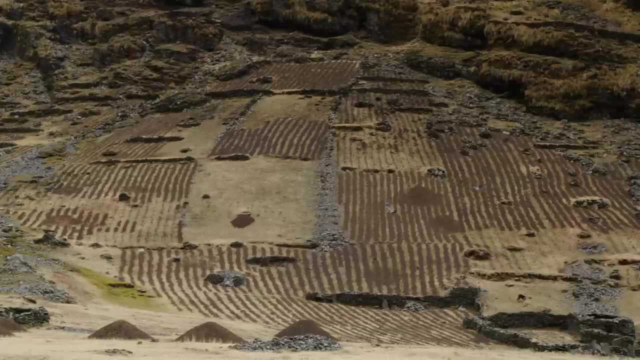 and further into the mountains. Here, what little farmable nature has to offer land exists is massively exposed to the extremes of weather. Above the treeline, the winter snows have melted. The highest terraces of all are fertilised and ready for planting. Those who are heading for the cities are leaving. 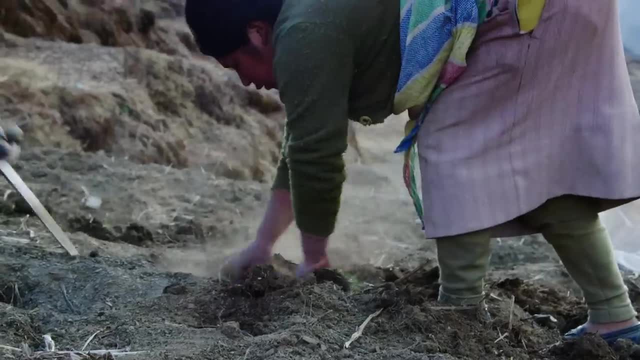 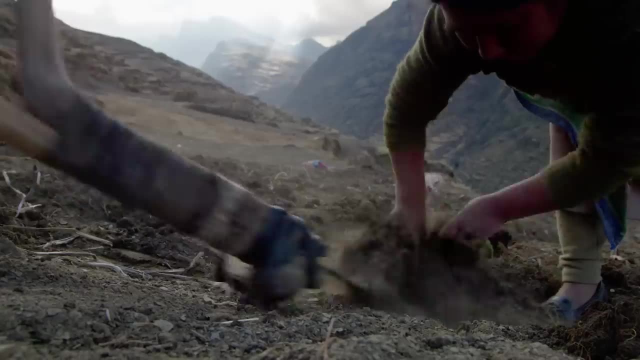 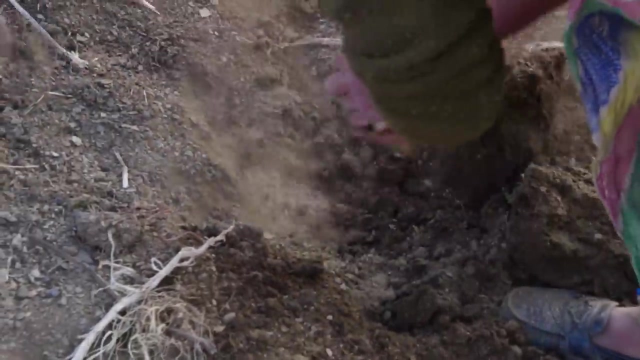 behind work which can have changed little since the Incas were lording it over the peasants of their empire. But those who remain do seem to enjoy one advantage: There's evidence that over the generations, their bodies have adapted to the thin air of the mountains. 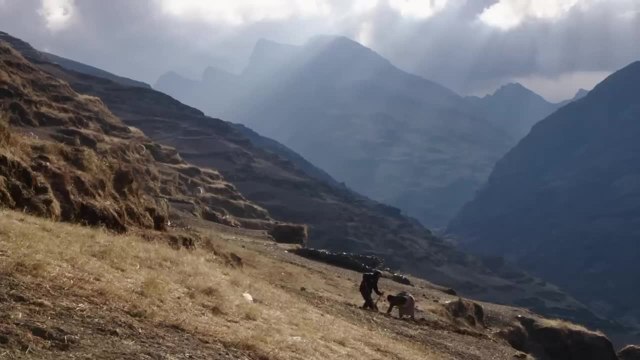 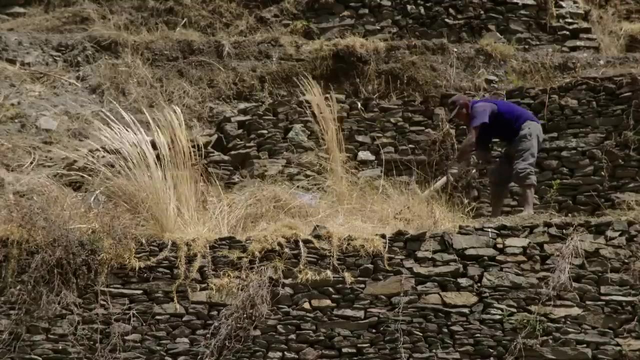 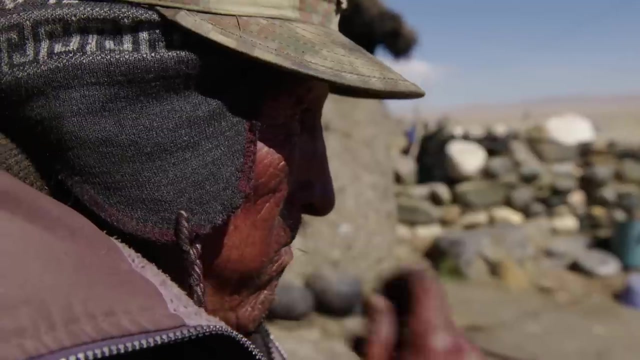 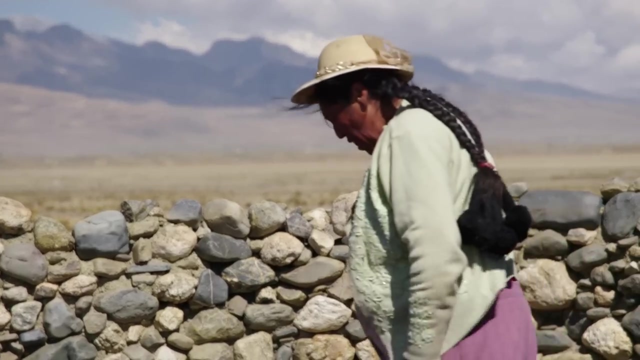 Their lung capacity is noticeably greater than those born at lower altitude. Their capacity for sheer hard work is even more striking, Even if they do depend on the stimulus of coca leaves to keep going. But up on the high plains, hard work and big lungs aren't enough to deliver a decent harvest. 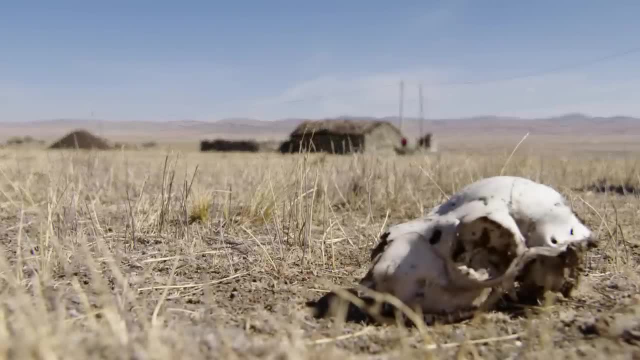 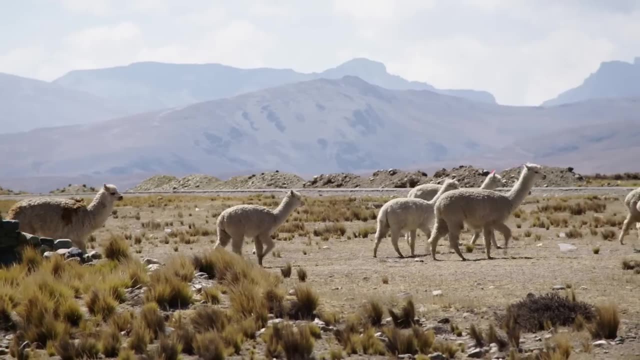 The winds are too strong, the soil too dry, the growing season too short. Rather than cultivate plants, people here have had to learn to breed animals. These are camelids, the alpacas and llamas, which have become synonymous with these mammals. 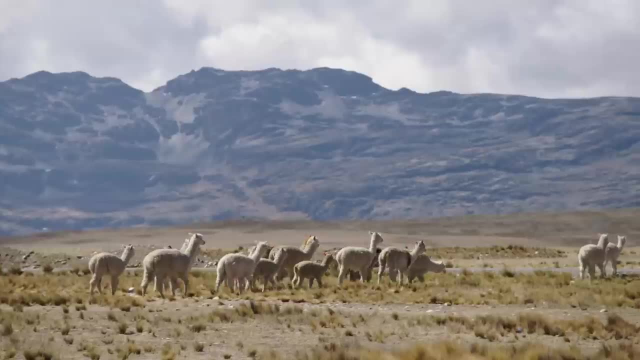 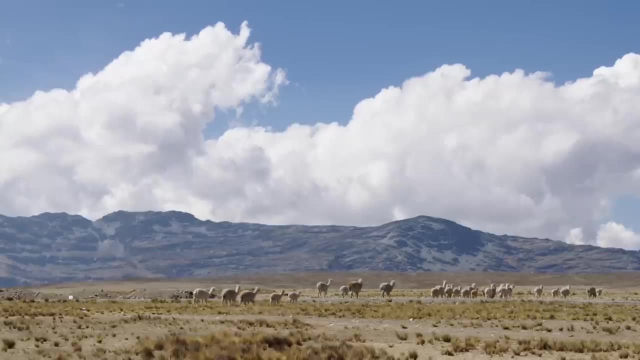 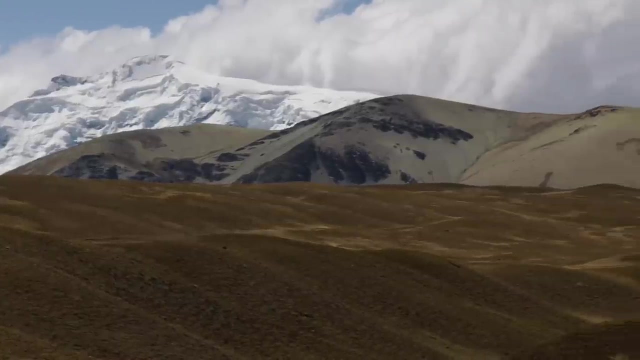 Their thick wool keeps them warm. Large hearts and lungs keep them well supplied with oxygen. These adaptations are inherited from wild ancestors which still survive in parts of the Andes. But up here, even with these advantages, semi-domesticated animals need the most careful husbandry. 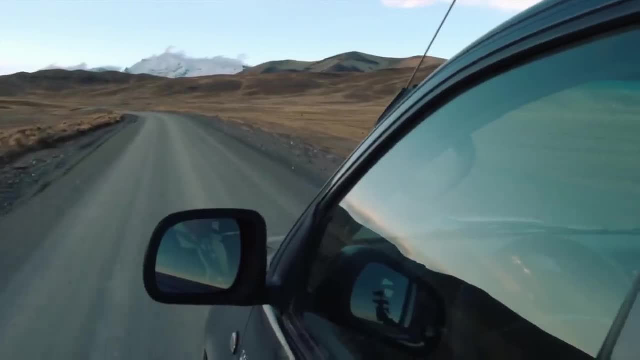 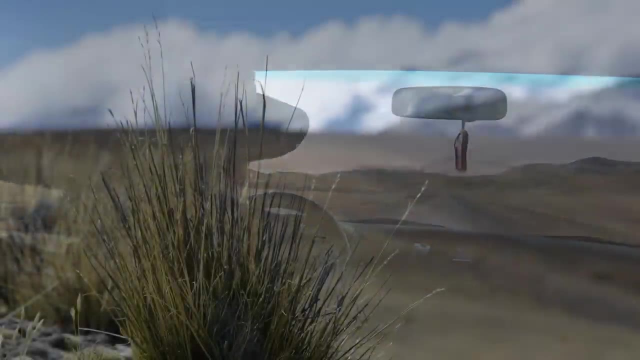 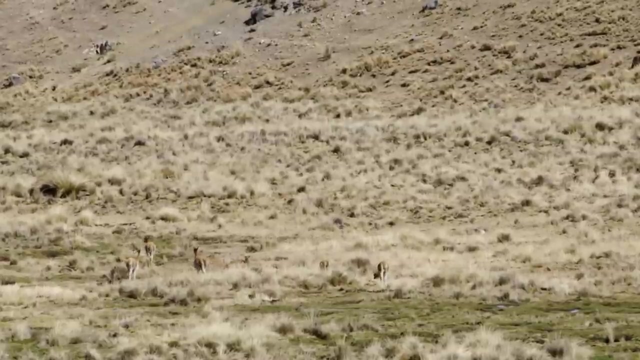 As part of a conservation effort focused on one particular species of camelid. government vet Viktor Ikvisek is on his way to a remote site. Here. herds of vicuñas are protected in large fenced-in compounds on the mountain sides. 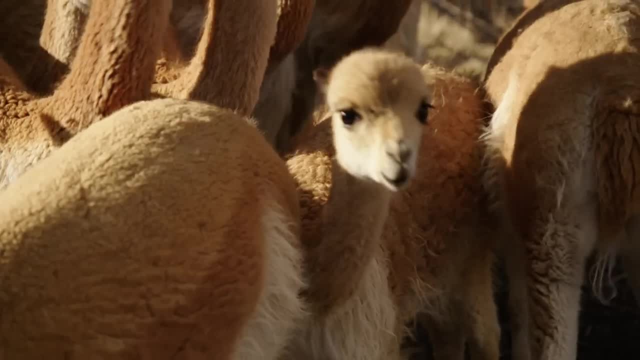 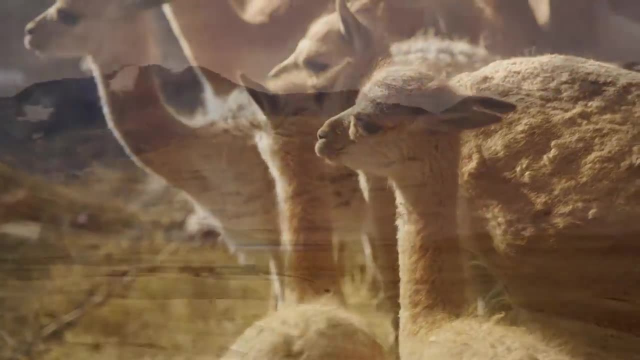 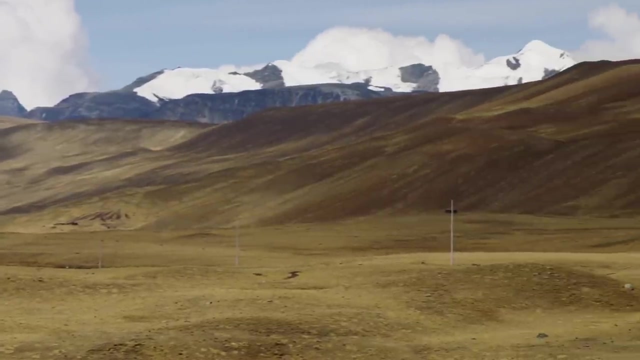 Fifty years ago, only a few thousand vicuñas remained in the Andes. Now, through careful supervision, more than a hundred thousand have grown in the rolling grasslands. They're still a protected species, but once a year local people are allowed to round them up. 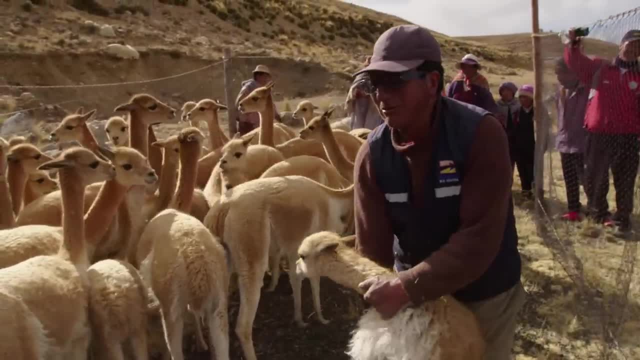 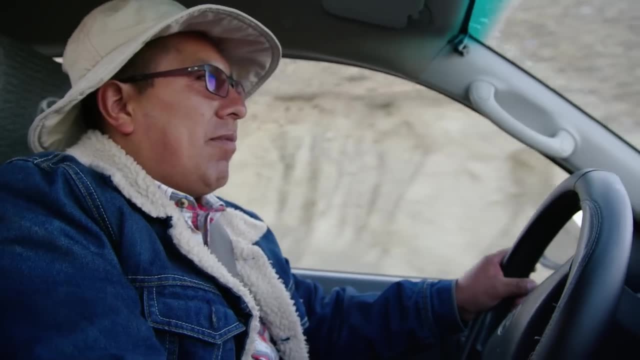 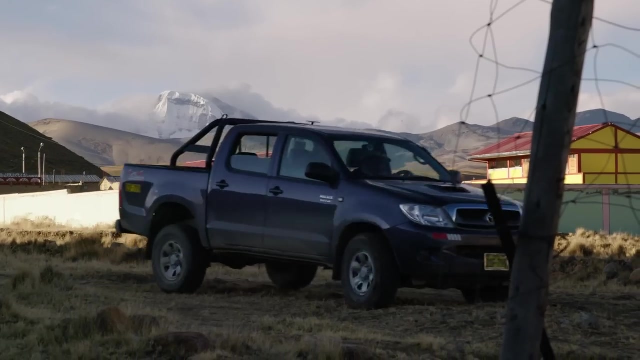 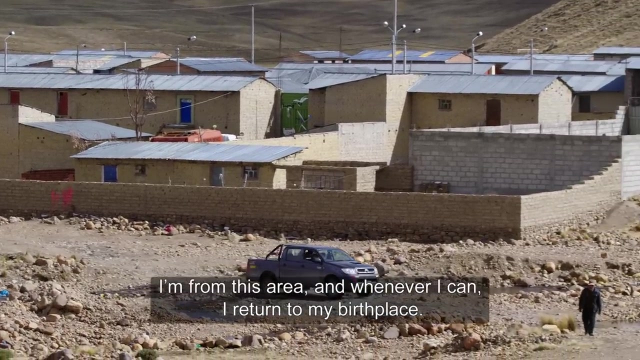 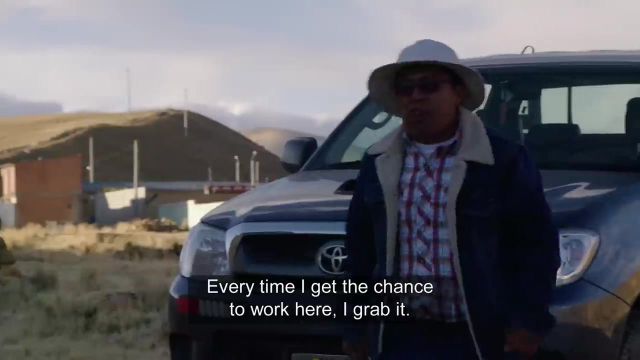 and to shear after them. The cattle town is free of fire. Viktor is coming here to oversee this year's herding. For him, the work is a delight rather than a burden. It's bringing him back to home ground, It's a pleasure. 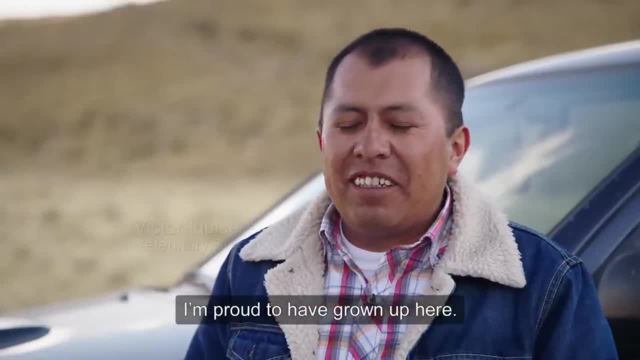 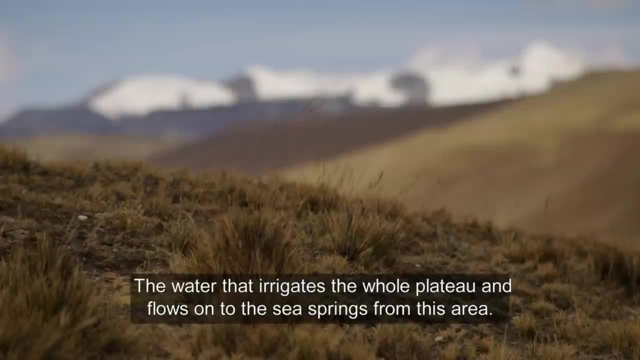 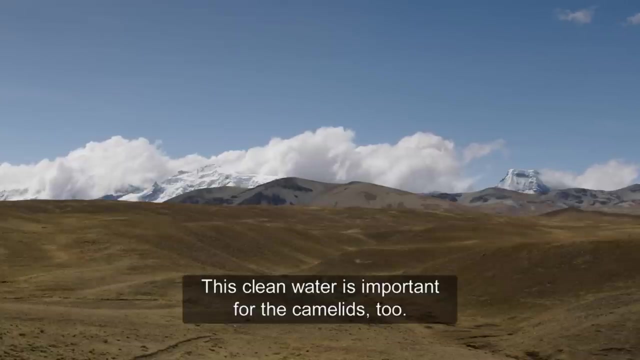 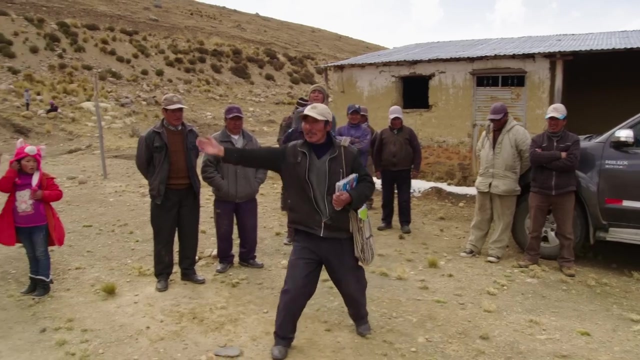 Growing up here means, for me, in particular, pride, Because this is the source of water that runs through the highlands, that reaches the sea. This is where the clean water comes from. This is where the camelids are fed first. We don't close the clock. 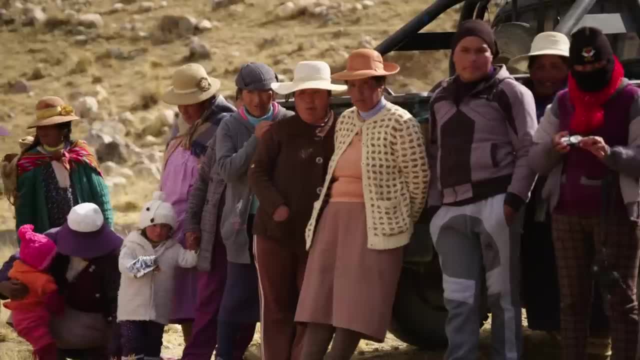 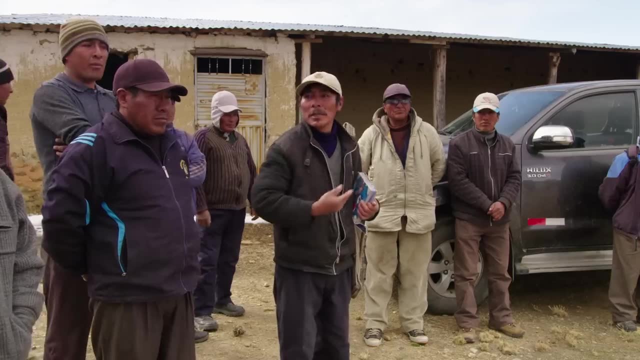 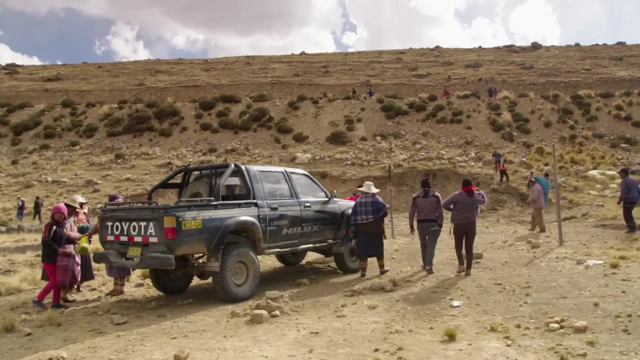 The herding is a big date locally. Most of the residents of Trapiche have turned down. They'll form a human chain spread across the hillside to round up the animals in a ceremony called a chacu. The cuña herding dates back to the days of the Incas. 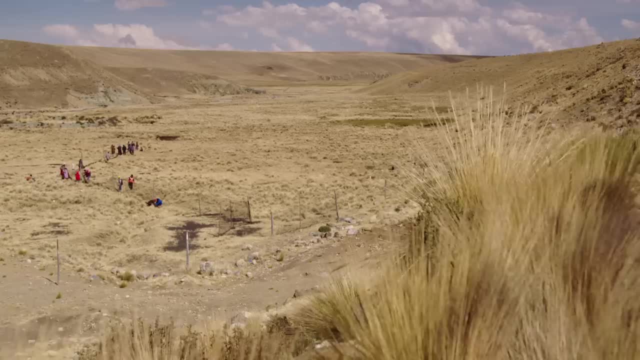 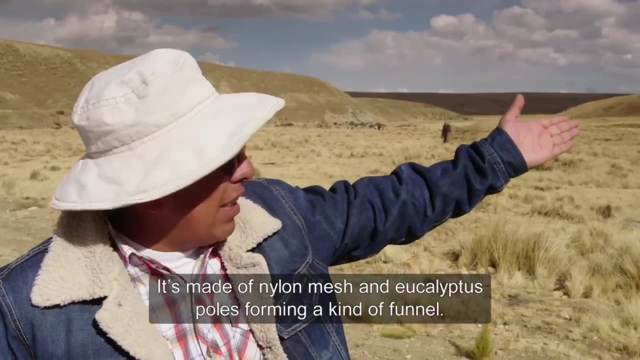 when wearing vicuña garments was a special privilege granted only to royalty. First of all, what is formed is the sleeve. what you see in this, the collectible mesh sleeve of nylon, of nylon material, and the eucalyptus sticks. 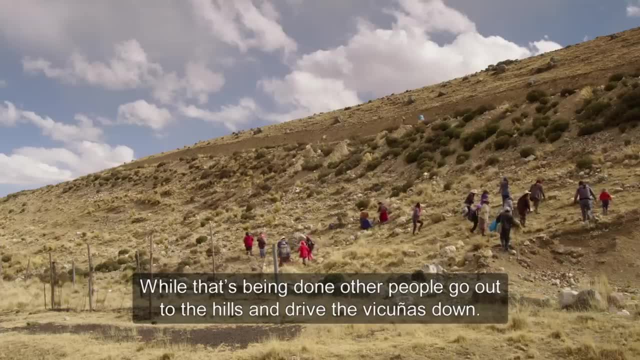 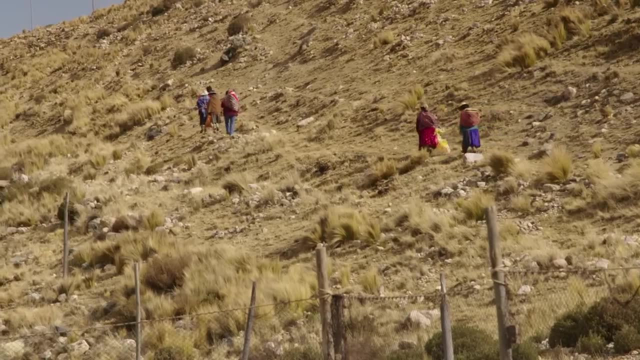 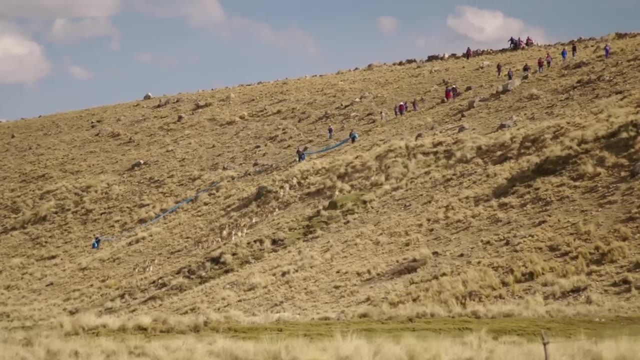 And the people who have gone have gone to collect the vicuñas which are located further down. The rules of engagement are strict. Viktor is here to make sure the villagers treat the animals gently throughout the herding and during the shearing. 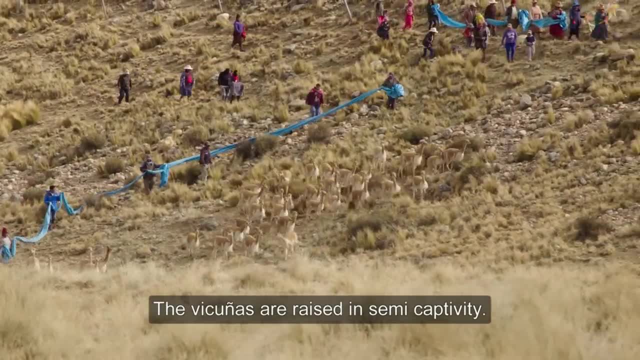 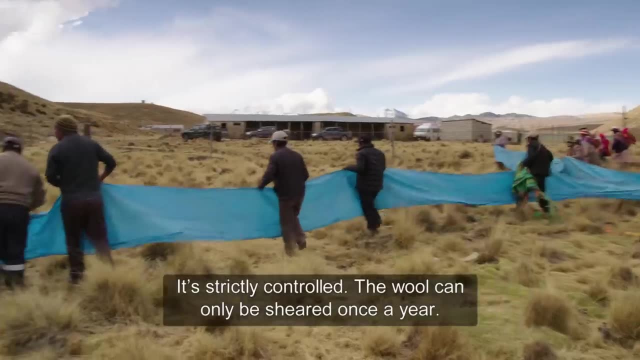 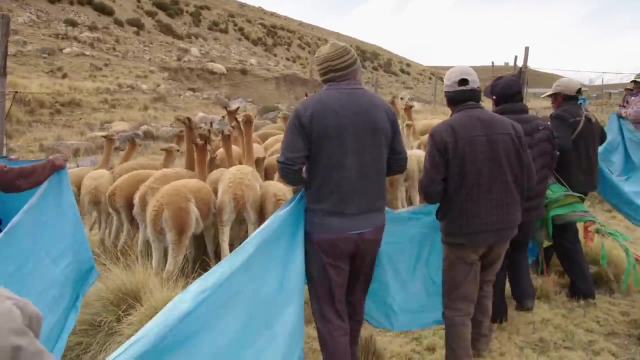 The vicuñas are currently being raised in this place in semi-cautiverio, authorized by the competent authorities. The fiber can only be sheared annually. It looks like fun, But this is a serious business And to ensure the vicuñas aren't under the firm. 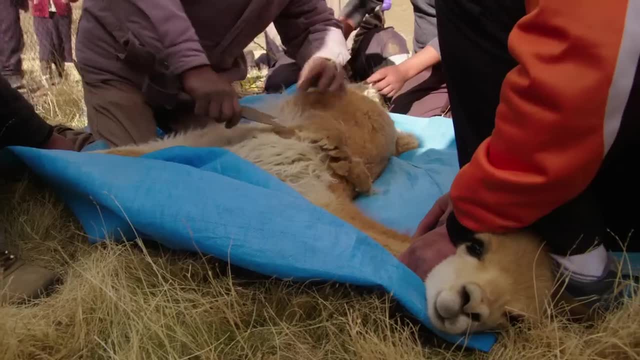 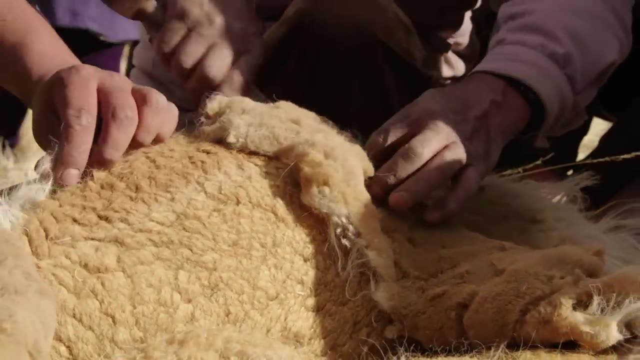 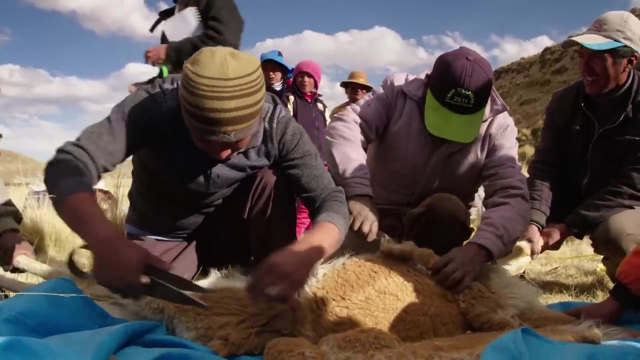 the authorities keep a watchful eye on the whole process. Wow, Nowadays anyone is allowed to wear the fine fibers over the vicuña's golden fleece, But in practice, only the very rich can afford to. A simple scarf costs as much as a thousand dollars. 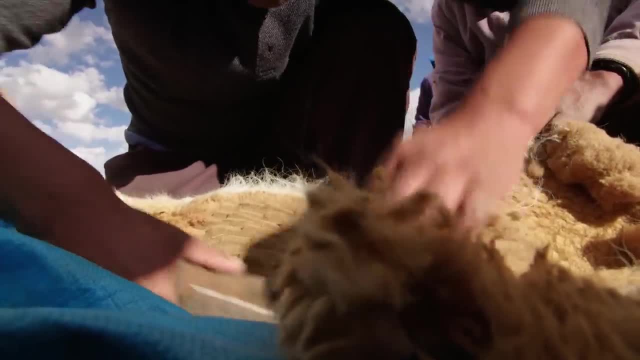 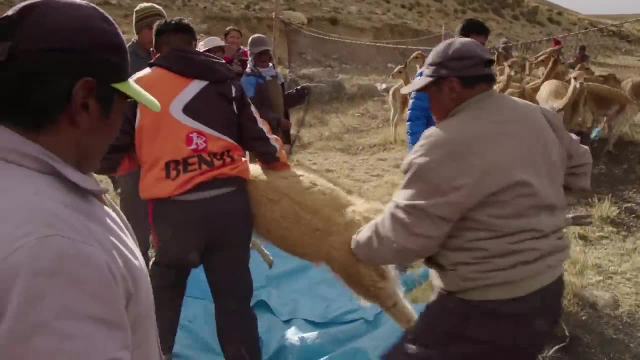 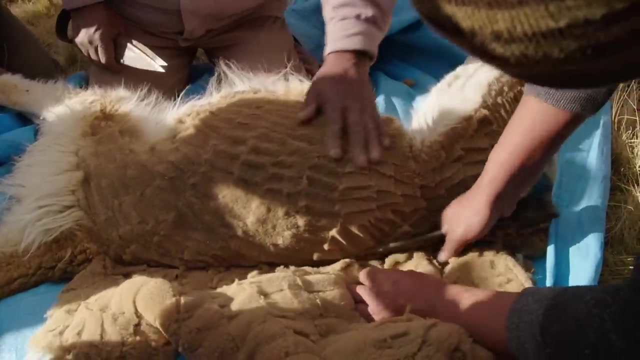 A vicuña wool suit forty times as much. Shearing of vicuña reduces less than 500 grams of fiber. This one has delivered just 200 grams And probably can't be sheared again for another two years. The scarcity value means that vicuña wool 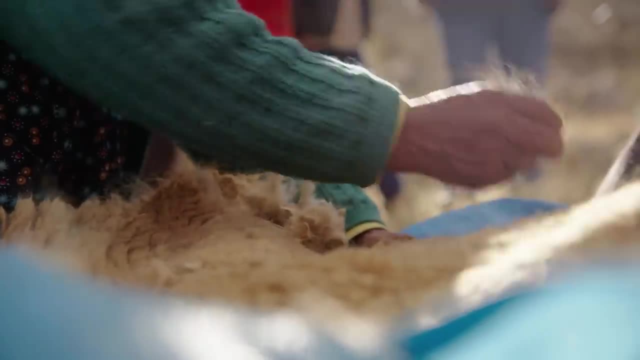 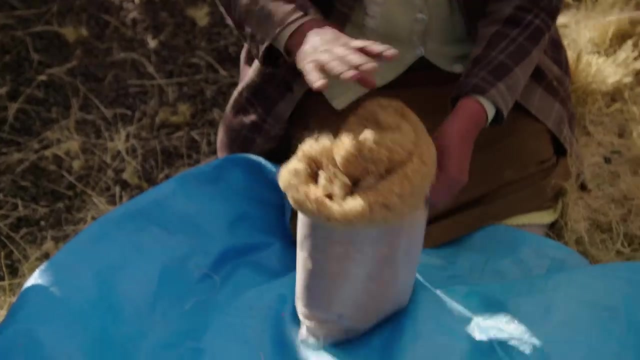 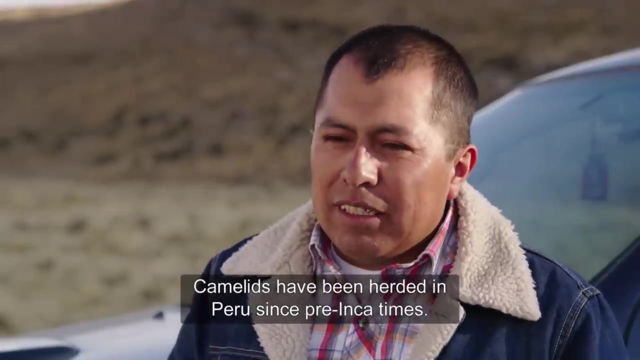 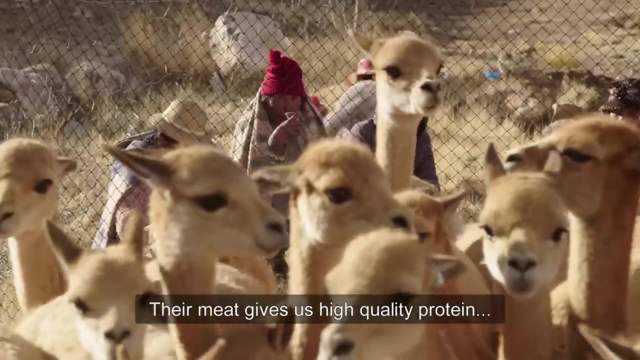 is one of the most expensive fibers in the world. It generates vitally needed cash for poor Andean communities like Trapiche, Camelidos have been used by the Peruvian man since pre-Incanato, before the Inca Empire. Since then, the Peruvian people 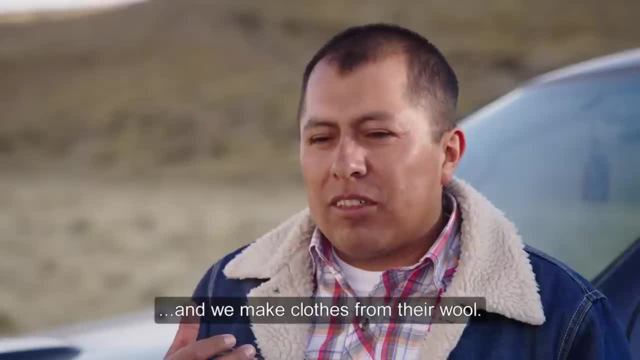 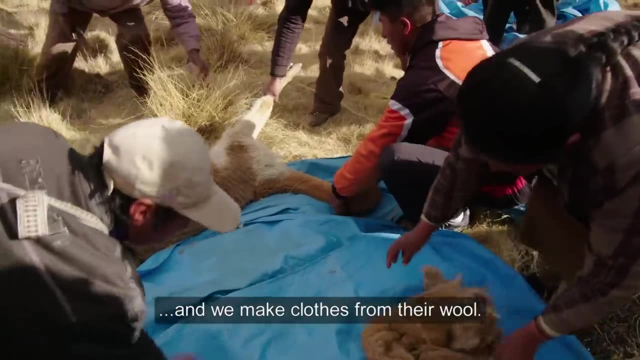 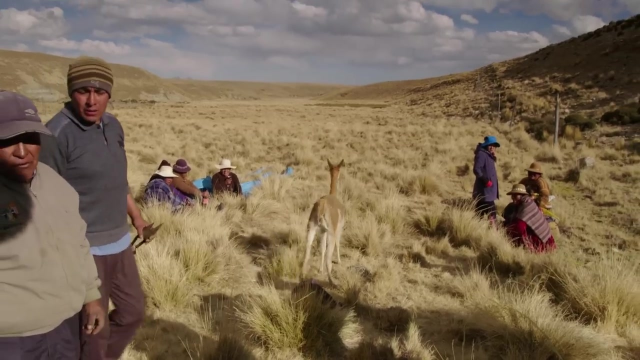 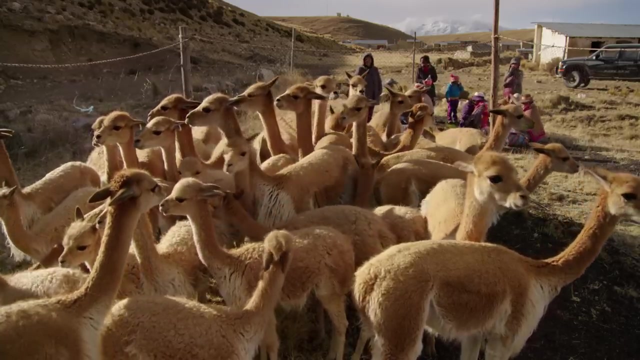 have been given their source of protein in the form of meat, and their fine fiber for their coats and their clothes. above all, No other productive creature is hardy enough to weather the conditions at this altitude. Hunter-gatherers the first ventured here in pursuit of animals like these. 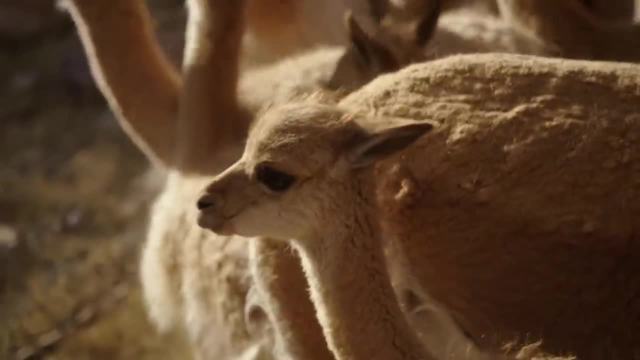 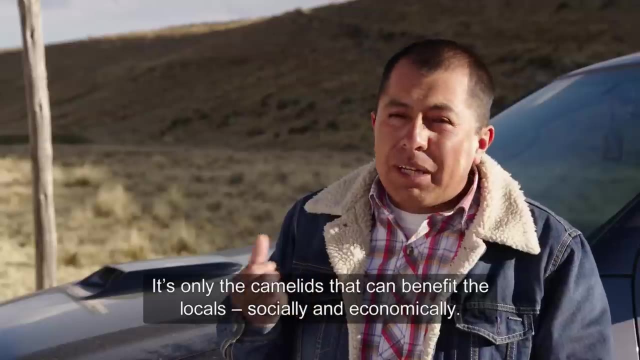 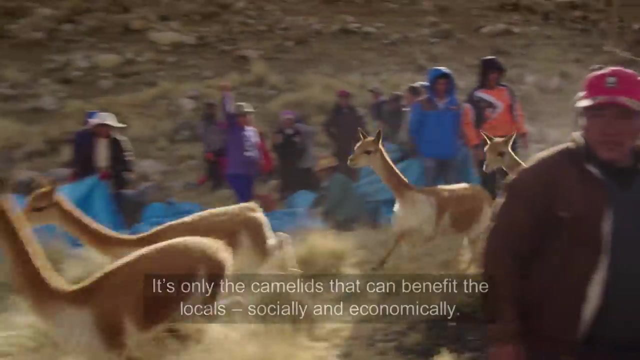 thousands of years ago. Today, Victor's relatives in Trapiche still prepare them. Only the camelidos take advantage, to benefit the inhabitants of these areas both economically and socially. Other species don't take advantage. they can't live in these areas. 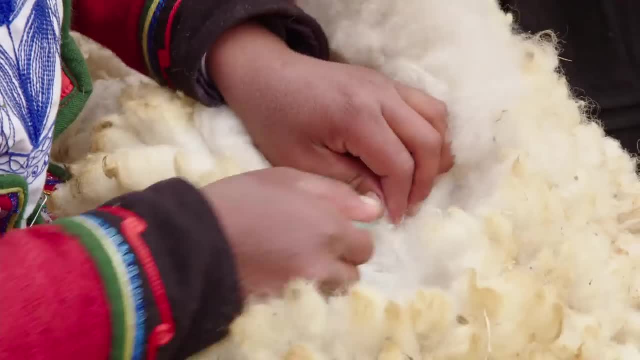 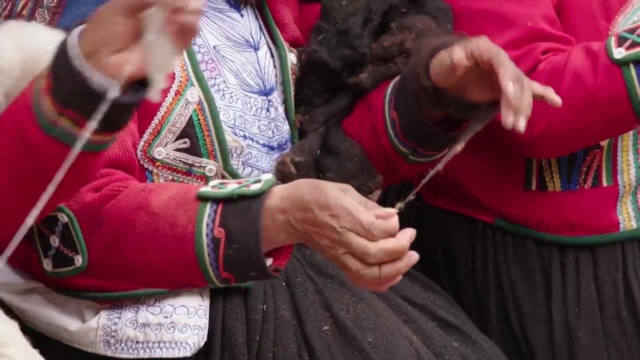 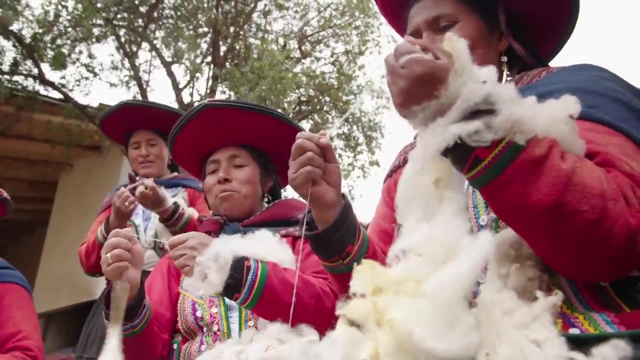 It's not just the Trapiche farmers who rely on the camelids. The economic value the animals generate sustains another important tradition in these mountains: weaving. Andean weavers are great innovators, developing over the centuries techniques which have spread throughout the world. 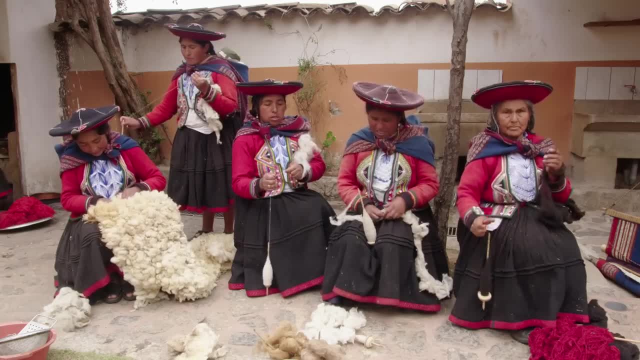 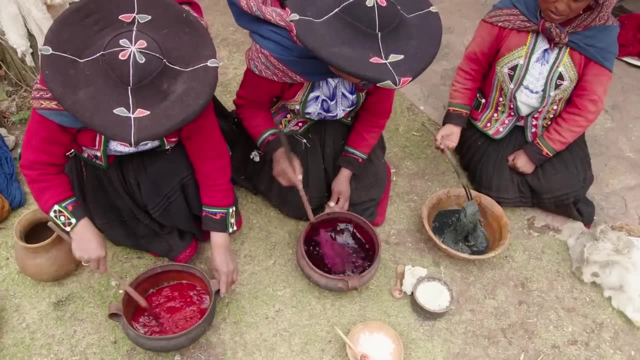 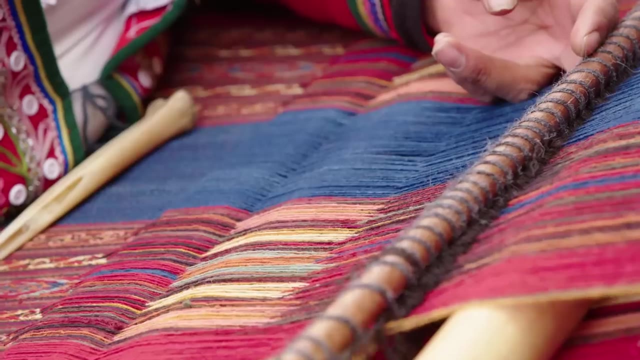 But there's one thing that makes them unique, and that's their craftsmanship. The clothes they make are highly practical. They keep people warm in the cold mountain air. But they're also badges of identity. The patterns and colours indicate the region and status. 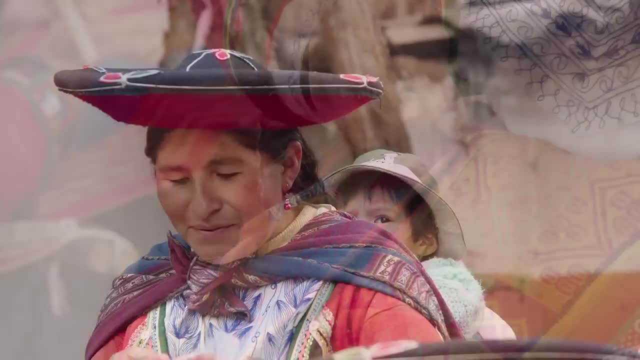 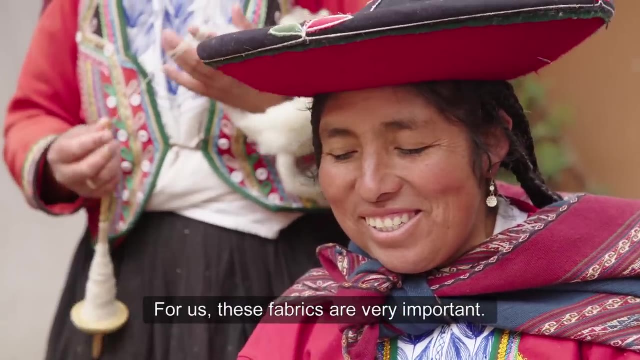 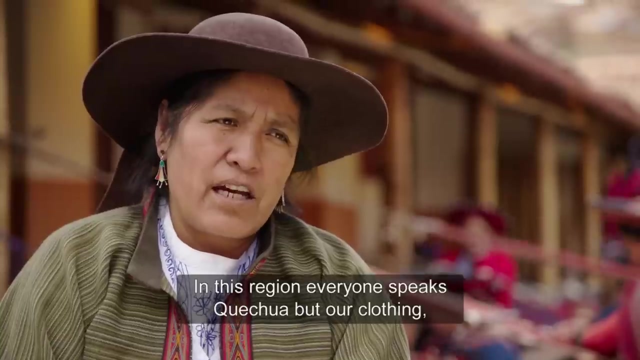 of those who are wearing them and even something about their attitude to life. It's very important that we identify the camelids and present them to the people. We don't have a specific region of origin, but we know that there are different. 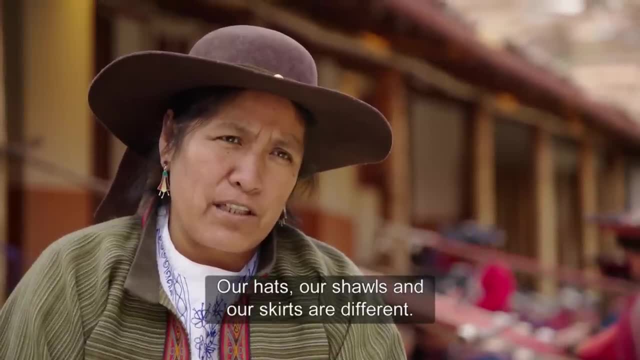 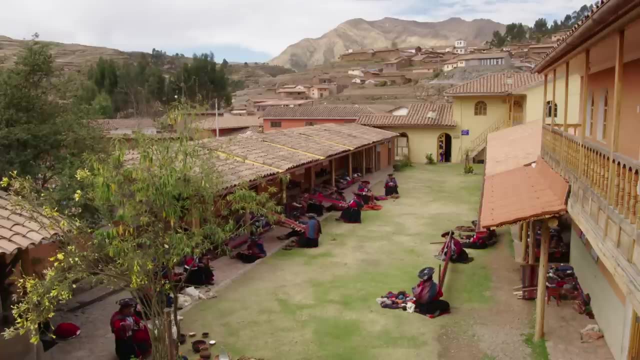 types of camelids, different types of sheep, different types of chickens. This is the mountain village of Chinchero, an ancient tambo or resting place on the Inca road through the Andes. Here, Nilda is leading a resurgence. 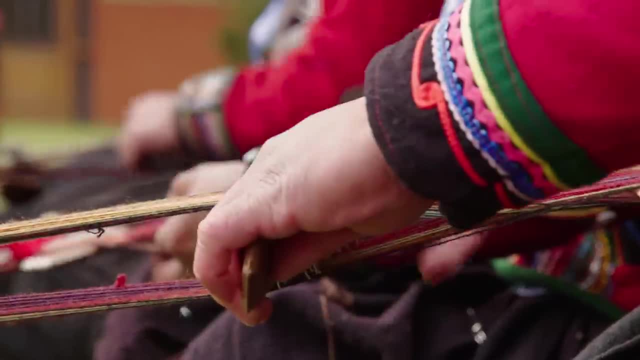 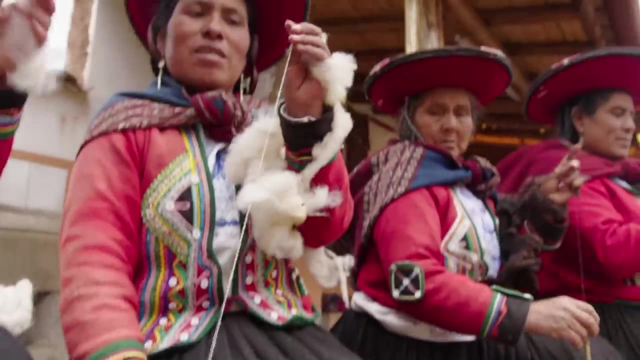 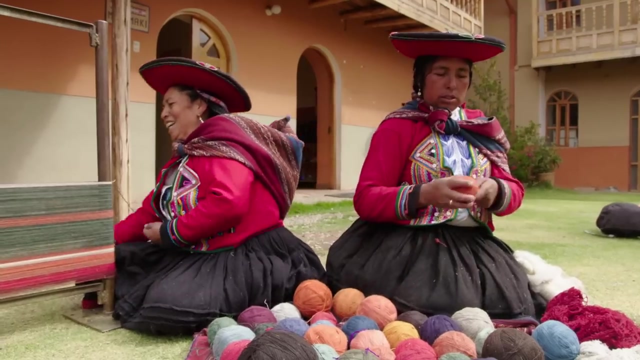 in the weaving traditions of the area. Craft skills and knowledge were in danger of disappearing as people settled for cheap, mass-produced imports rather than hand-crafted indigenous clothes. Setting up the centre for the traditional textiles of Cusco was Nilda's response. 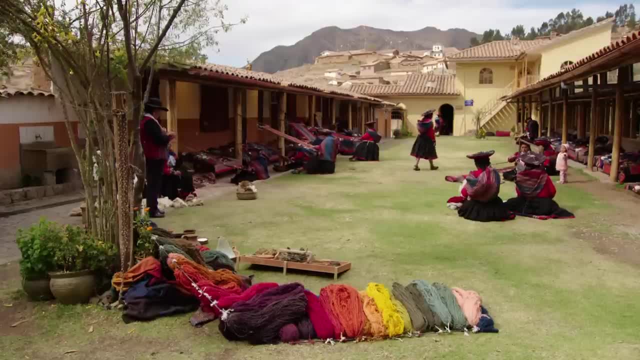 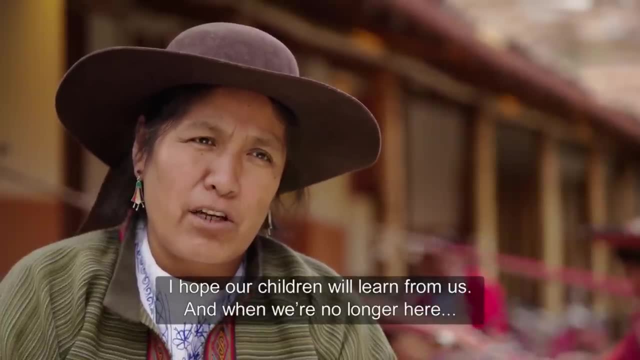 to worries that a whole way of life was passing away. We have a lot of work to do and we have a lot of work to do. We have a lot of work to do and we have a lot of work to do and we have a lot of work. 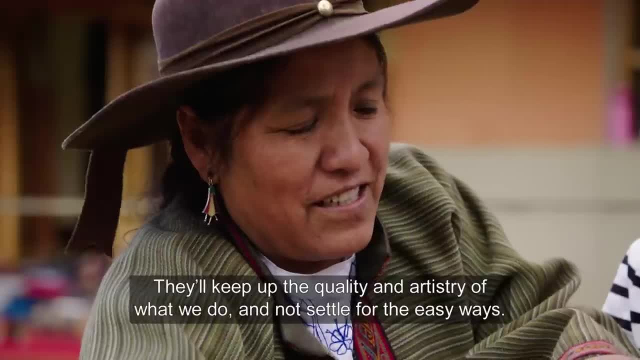 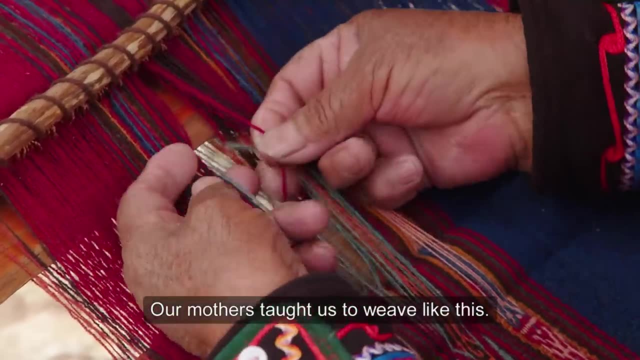 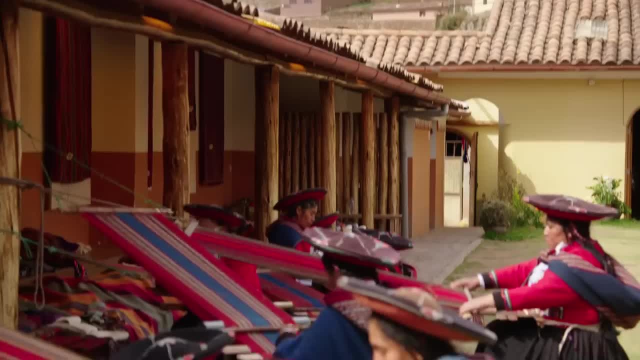 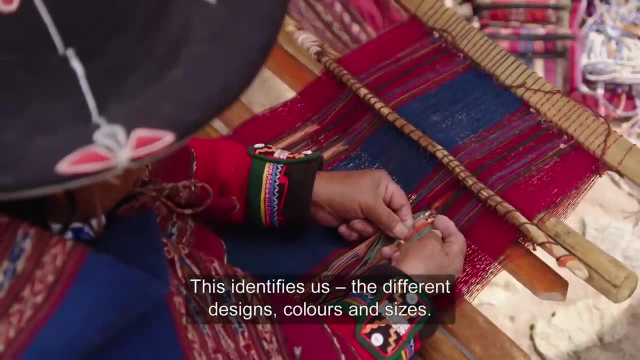 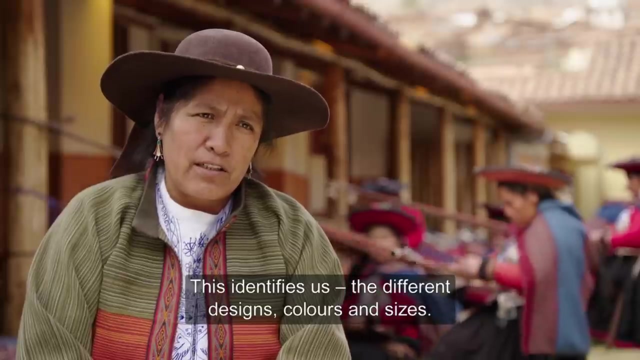 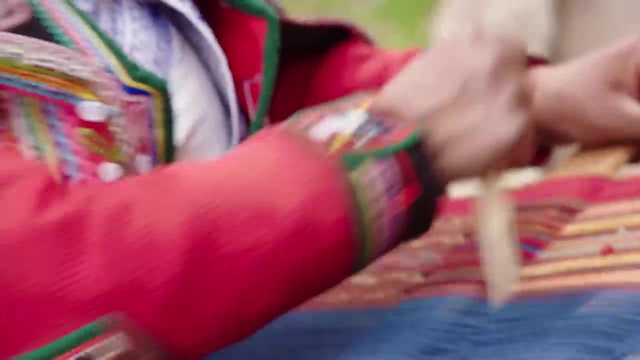 Today, the project supports weaving in villages all over the region, but the revival started right here in Nilda's home community. It's not just the fabric, it's the color, it's the size of the fabric, It's the size of the fabric and it's the size of the fabric itself. 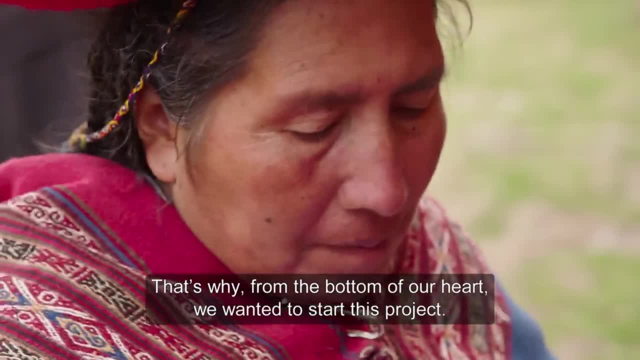 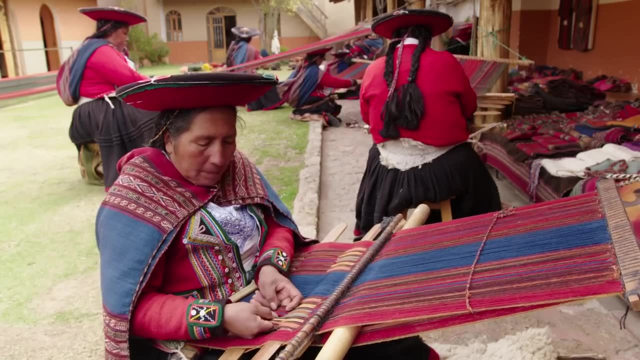 So it's the size of the fabric and it's the size of the fabric itself. Chinchero patterns are an integral part of one of the oldest textile traditions in the world. You might even say they're woven into the fabric of life here. 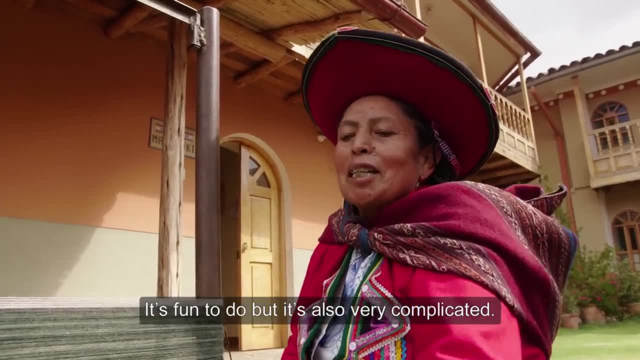 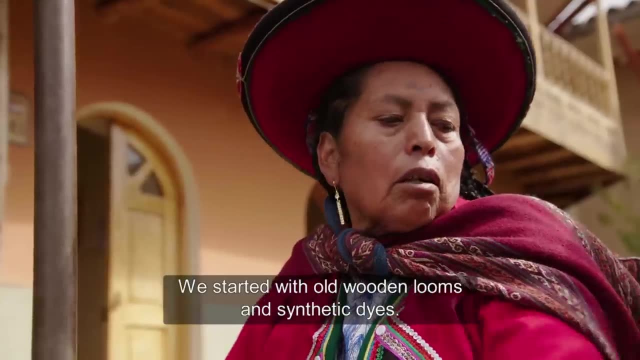 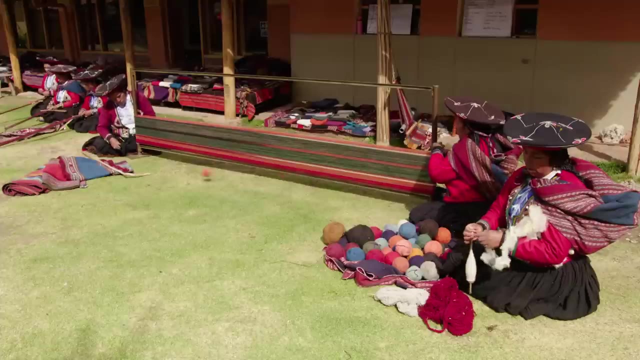 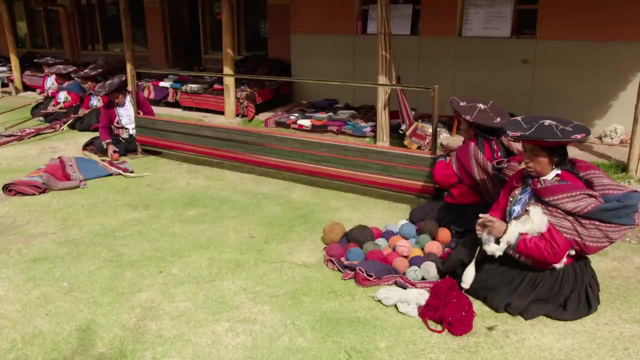 We have a lot of different fabrics here. We have a lot of different fabrics here. We have synthetic fabrics, we have pull-bombs, we have natural fabrics. We have natural fabrics here. The larger, more complicated designs can take weeks to finish. 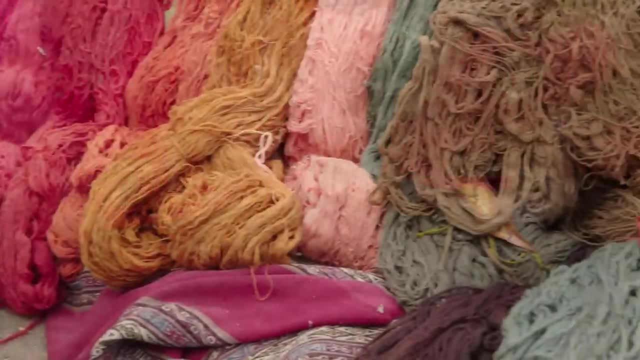 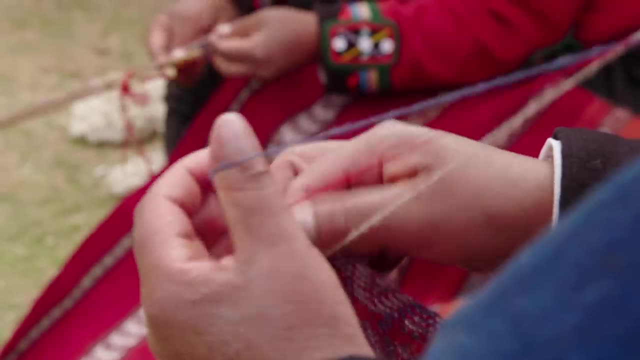 Spinning loads of fabric can take weeks to finish. Weaving local wool, dyeing it with plants from the hills, weaving it on traditional looms. There are no shortcuts to reinventing a tradition, But when each piece of cloth is finished, it's said that something of the spirit. 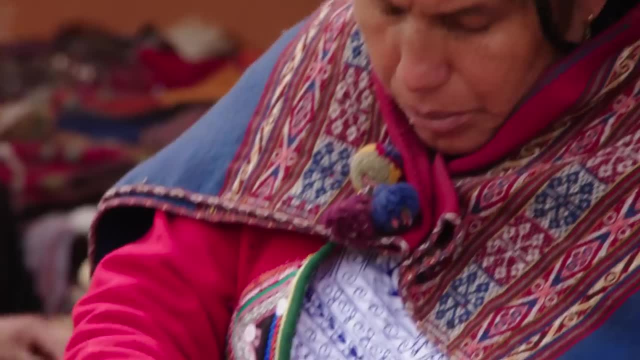 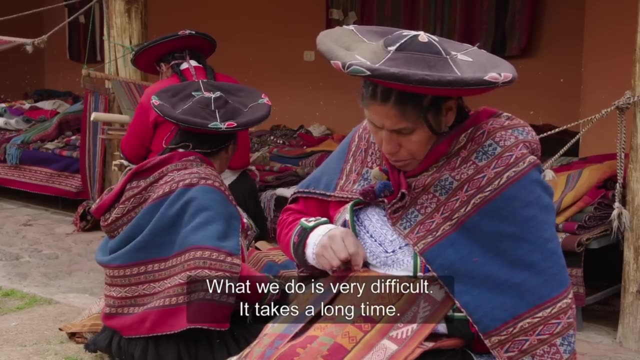 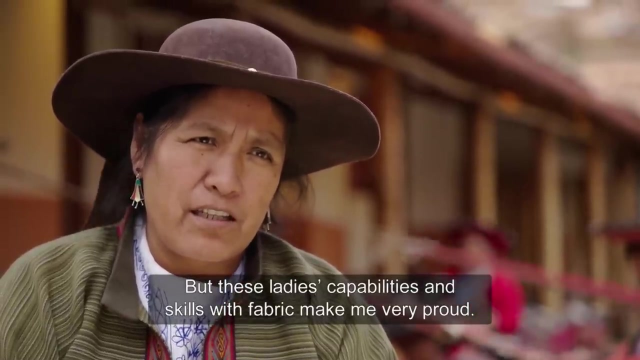 the skill and the personal history of the weaver has entered into it. It's not easy to make something like this. It takes a lot of time, But I'm very proud of what I've done. I hope that the people who have made these clothes can see the value of our art. 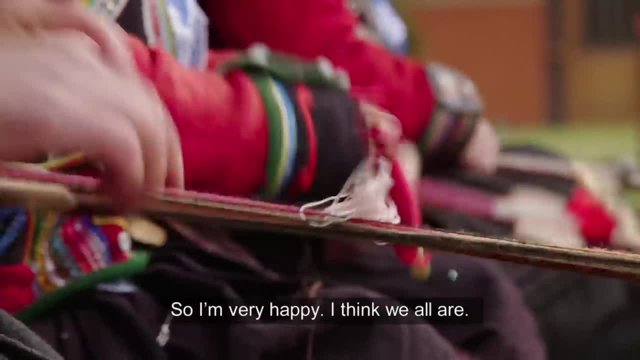 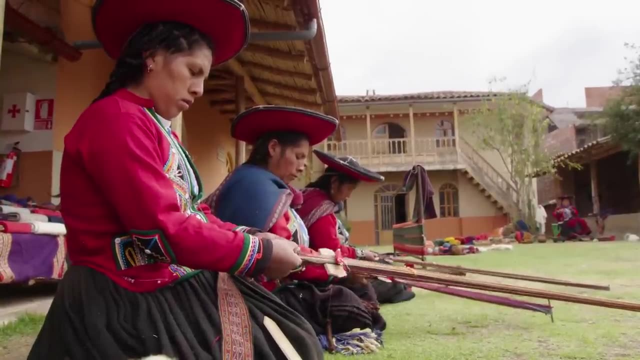 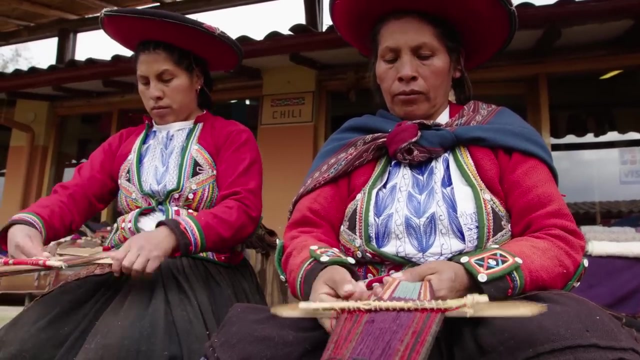 I hope that it can help them understand what it is. I hope that it will be a way of making their life happy. For centuries, indigenous people were looked down on, made to feel ashamed of their identity and traditions. This venture is helping to restore the women's dignity. 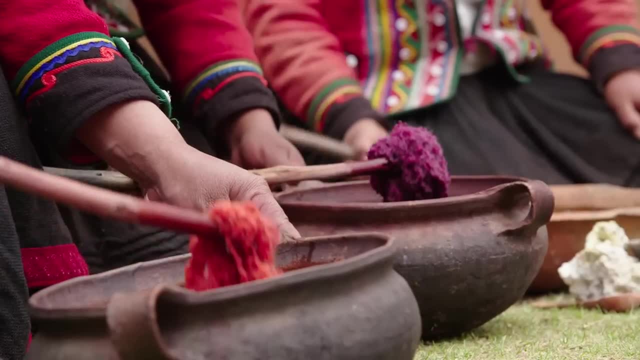 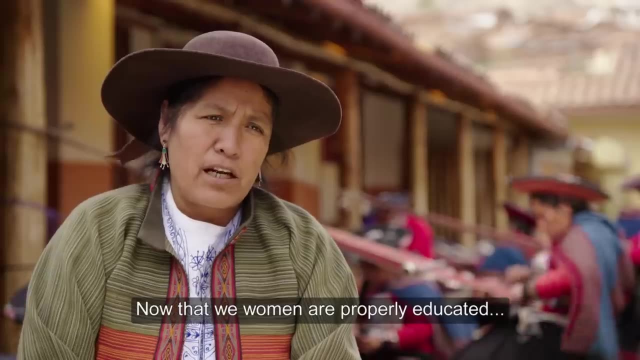 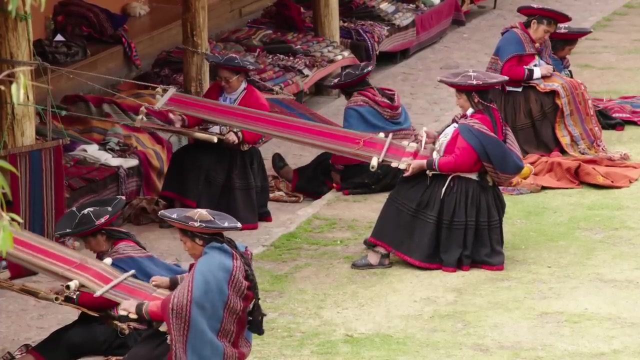 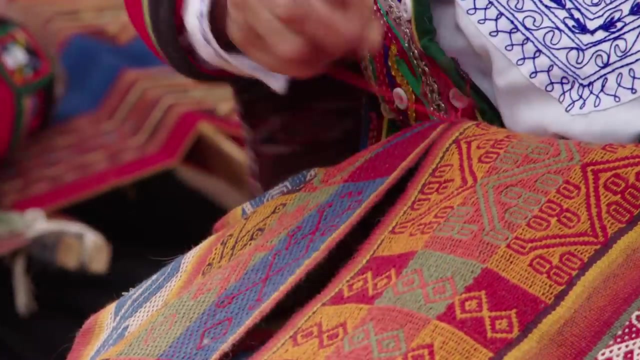 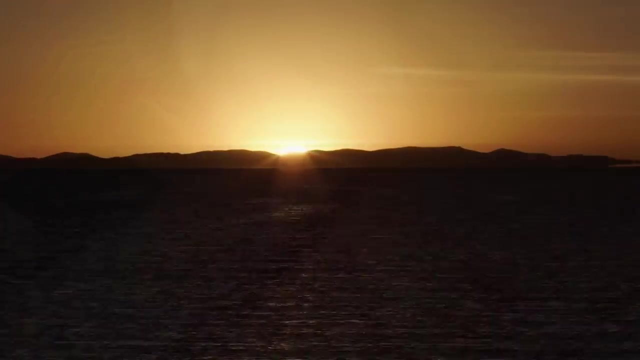 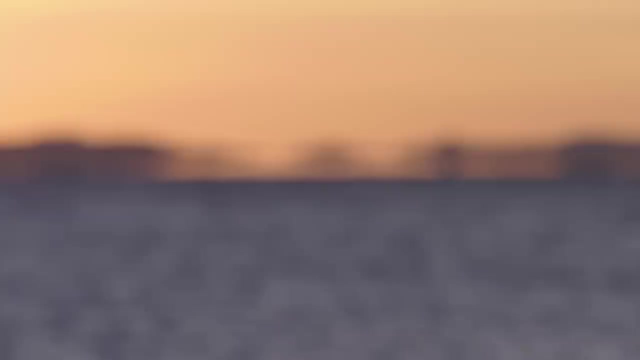 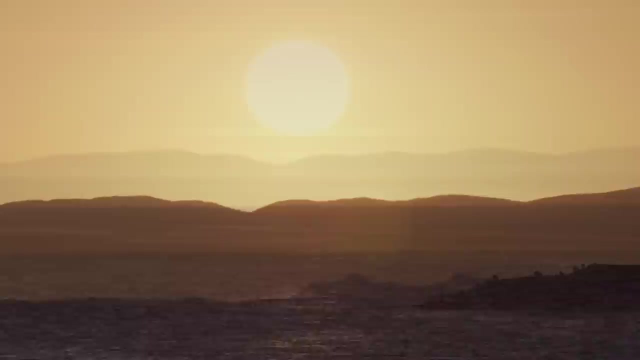 Their dignity in their work, In their community And in themselves. Mahatma Gandhi declared that weaving should form part of any true system of education. The women of Chinchero would agree. Lake Titicaca, the largest lake in South America. It's the highest body of navigable water. 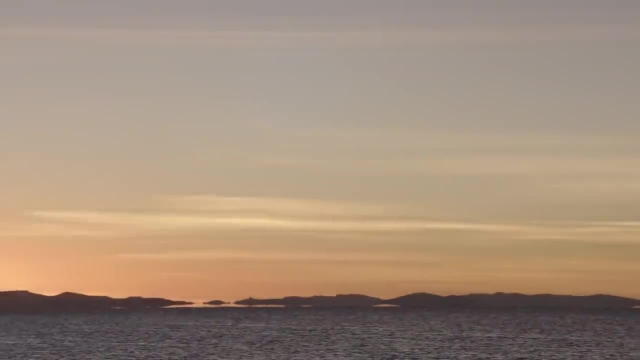 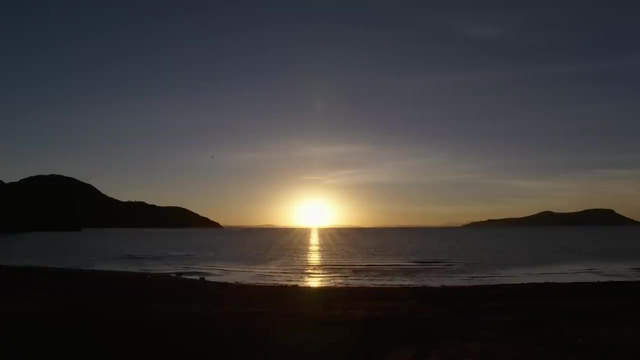 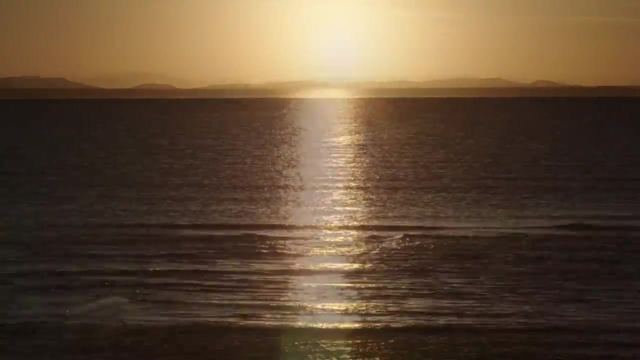 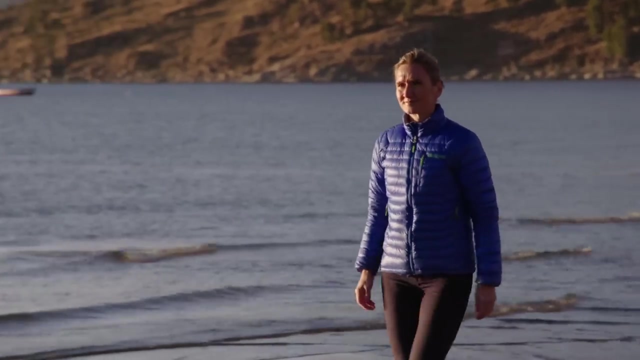 in the whole world. Sunrise over its waters is one of those must-see items on any tourist's itinerary, But one visitor today is here for more than the stunning views. Lowri Morgan is a world-class endurance athlete from Wales. in the UK She competes professionally. 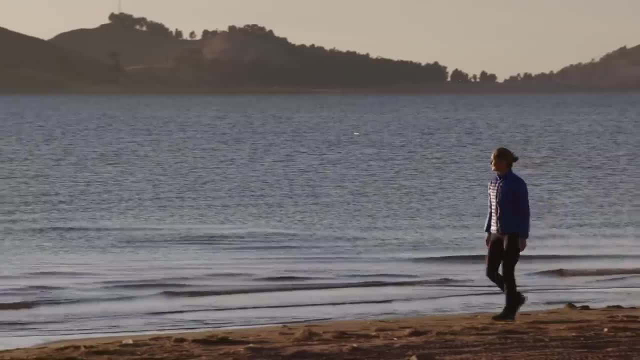 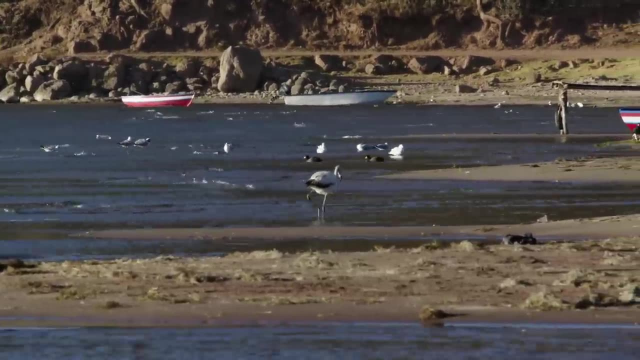 in ultramarathons. races held over hundreds of kilometres in climates as different as the jungles of the Amazon and the Arctic. As part of a short visit to the Andes, Lowri is assessing the mountains as a base for high altitudes. 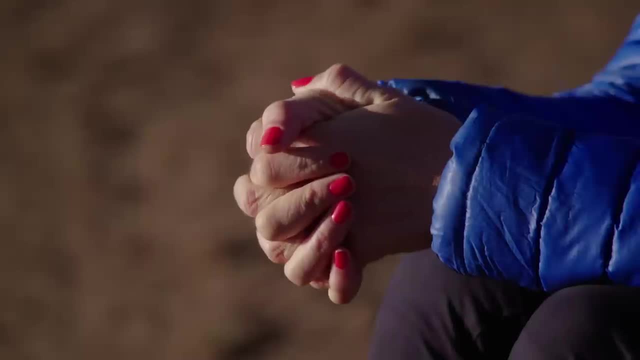 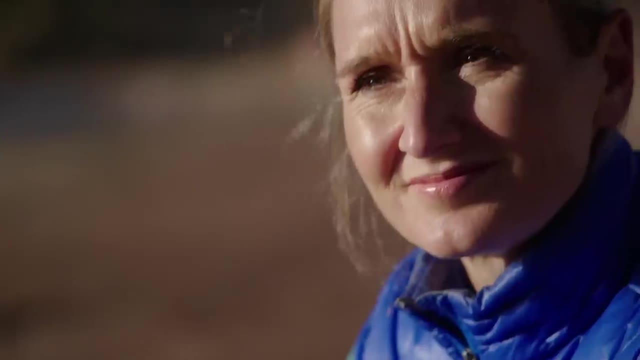 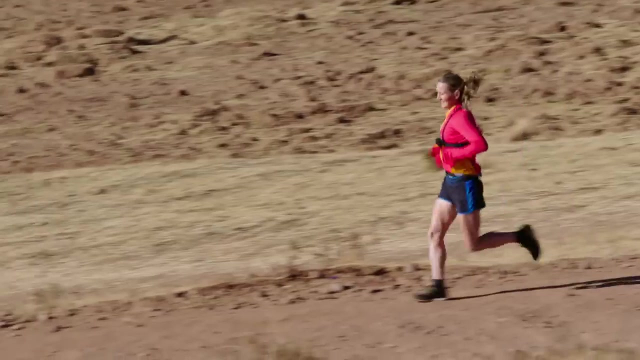 I know many ultra-endurance athletes train about 2,000 to a half thousand metres above sea level, but I think this is the extreme. Ultra-athletes have to absorb huge amounts of oxygen to sustain their exertions over massive distances. Up here there's so much less oxygen in the air: only about 60% of. 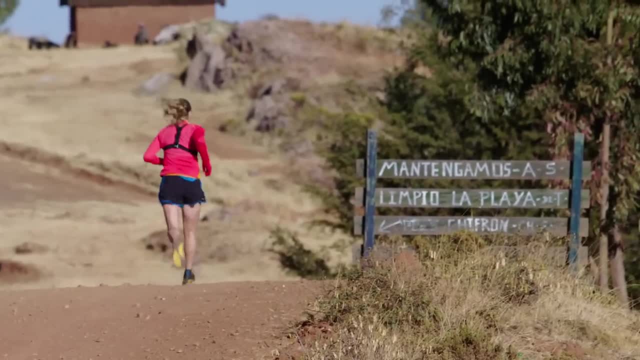 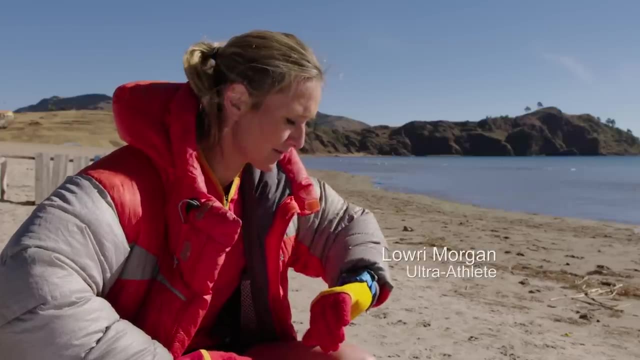 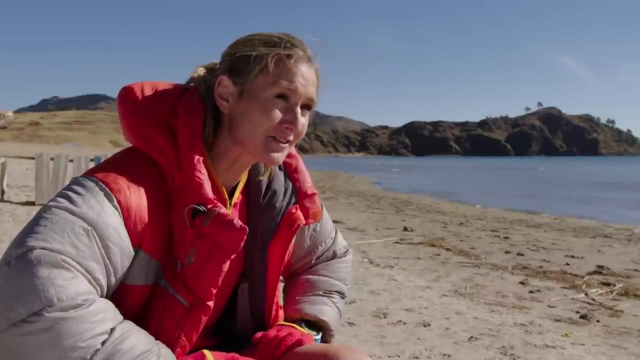 the amount found at sea level. I find it's incredible that there are so many people around me in the Alps, But nothing compares to where we are now. We are 3,850 metres above sea level and it's a new experience for me. 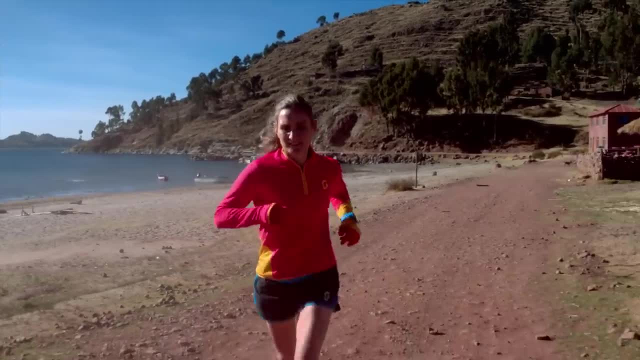 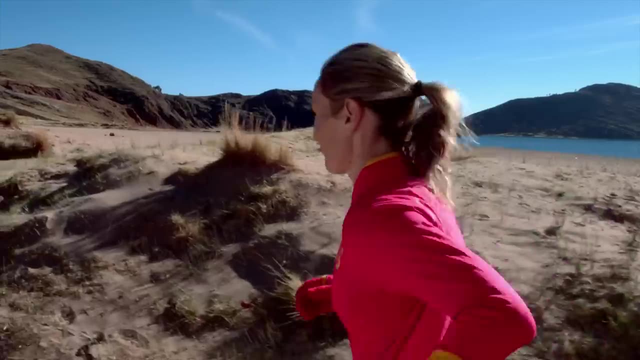 Training at altitude encourages the body to produce more red blood cells which absorb oxygen, and more mitochondria to use that oxygen to generate energy. All this helps increase an athlete's VO2 max- The amount of oxygen in your blood cells. maybe less than. 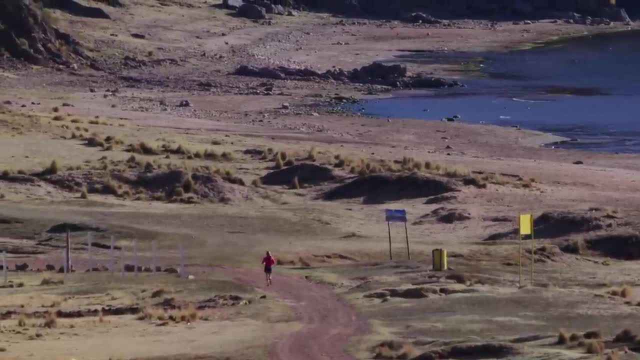 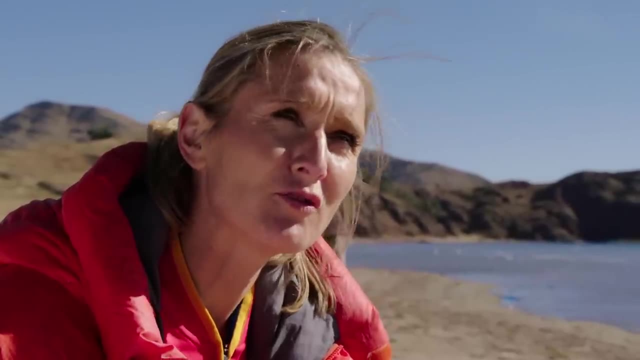 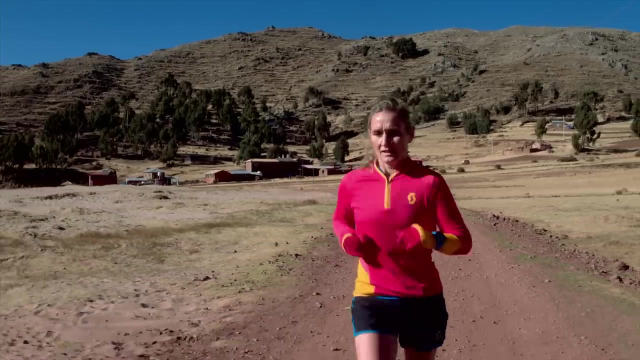 amount of oxygen they can take in. but it doesn't happen overnight. I think you need at least two weeks to properly acclimatise. They say about four weeks is a good time to be up in the mountains, but ideally you need to live in the mountains. 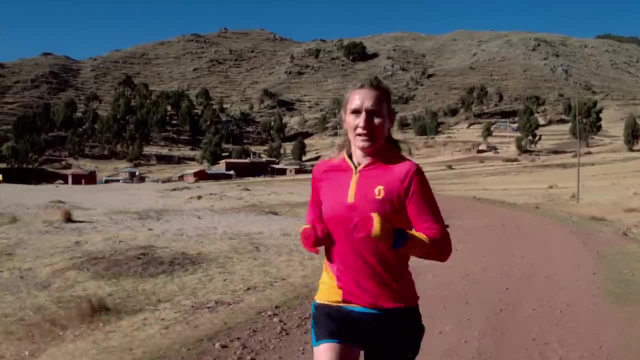 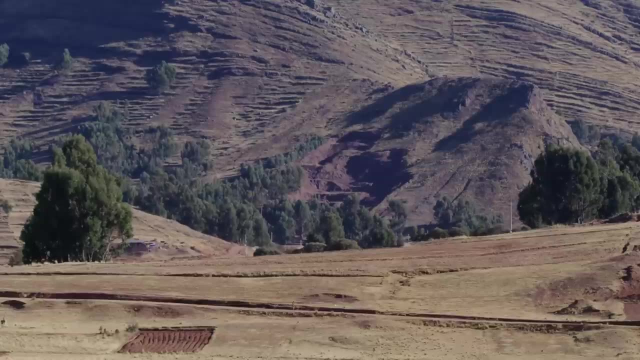 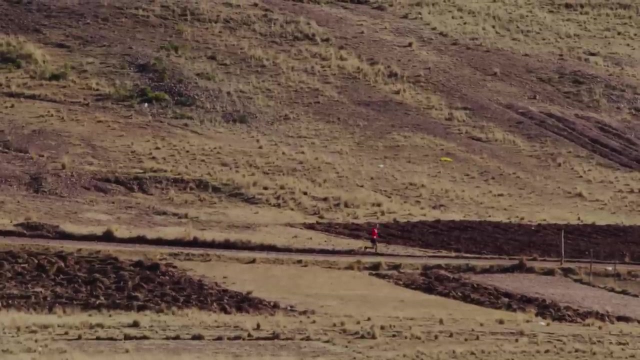 I know many endurance athletes who have actually moved to the Alps or Kenya or Boulder in Colorado to really take advantage. Their VO2 max increases, their overall strength increases. You see them at the next race and they've improved incredibly. It definitely works, but you do. 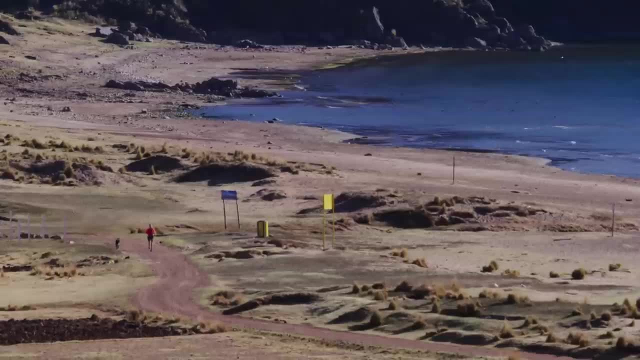 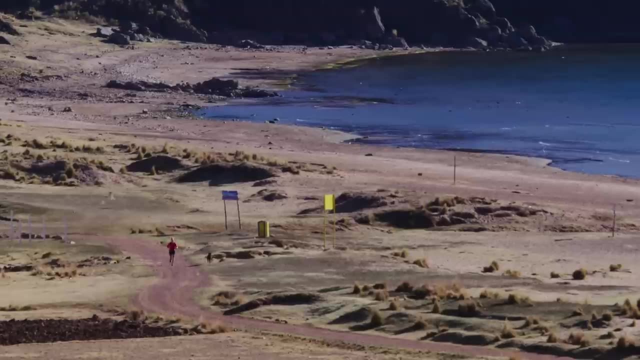 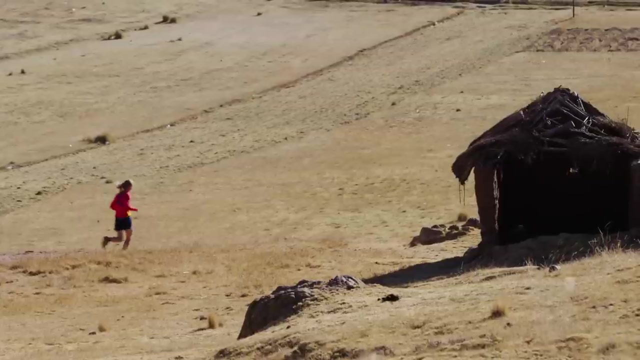 need to change your lifestyle, basically to move to the mountains. Seeing something of how the local population copes with life and work at extreme altitude has been a real eye-opener for this world-class performer. I have the utmost respect for the people who live here. It's really hard- practical and physical work. 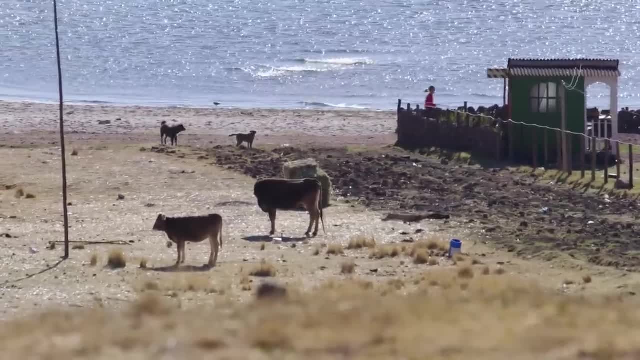 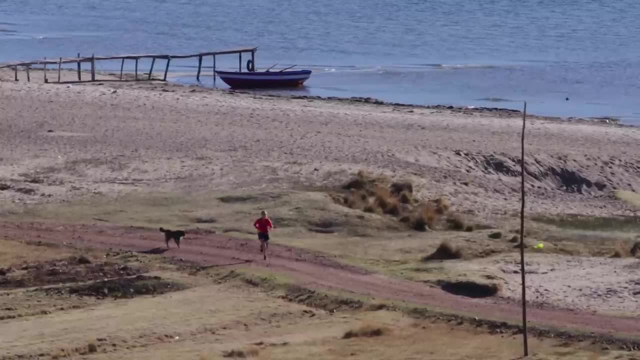 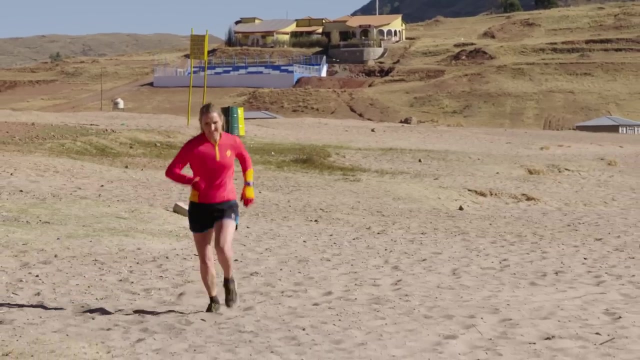 up here and to be able to do that day in, day out is incredible to see. So their fitness levels must be fantastic. I must admit I know many of us athletes use altitude masks and altitude tents, but nothing compares with living in the high mountains. 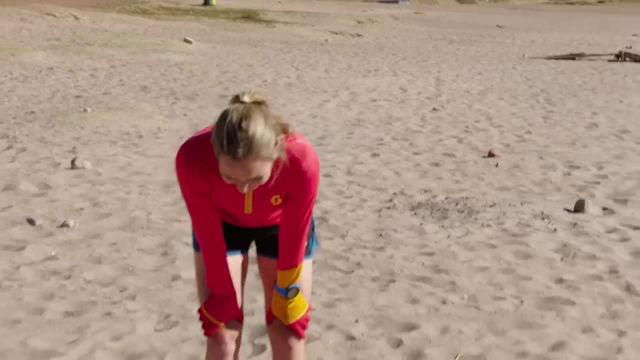 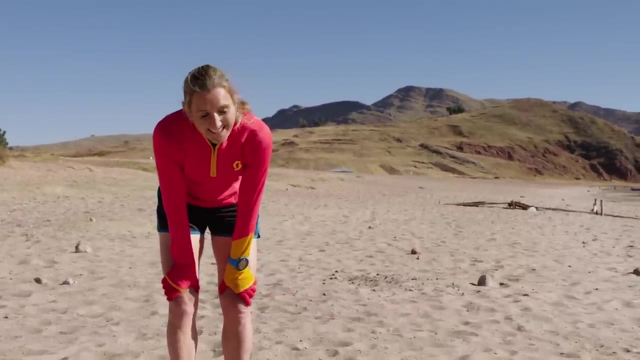 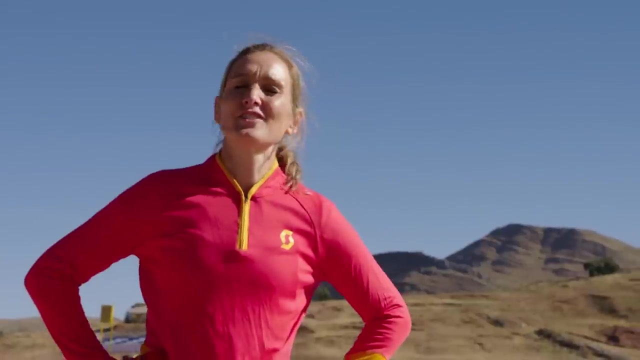 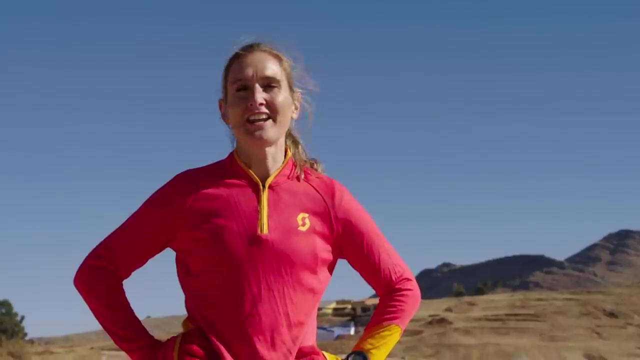 That was tough, Much harder than expected, Really really tough. It's so frustrating. so frustrating because the amount I just ran is so small compared to what I'm used to. I'm used to running 100-milers, 100-hours, 100-hours, 100-hours, 100-hours, 100-hours. 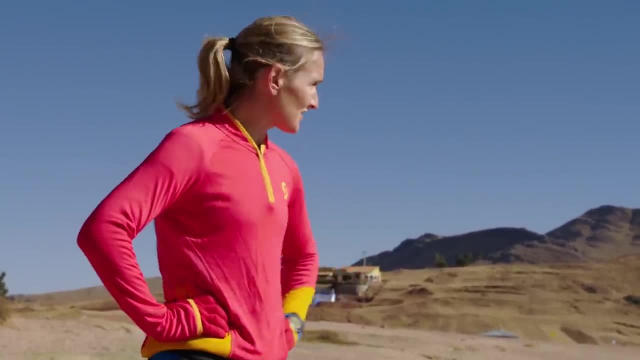 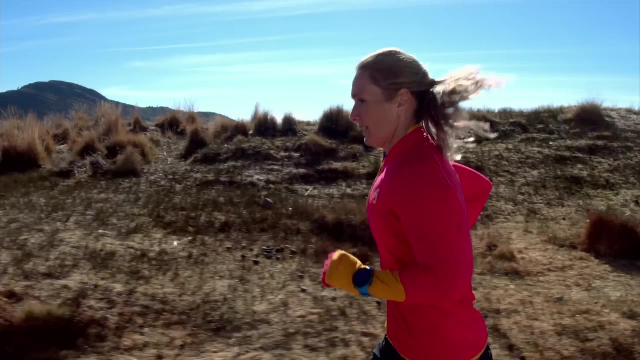 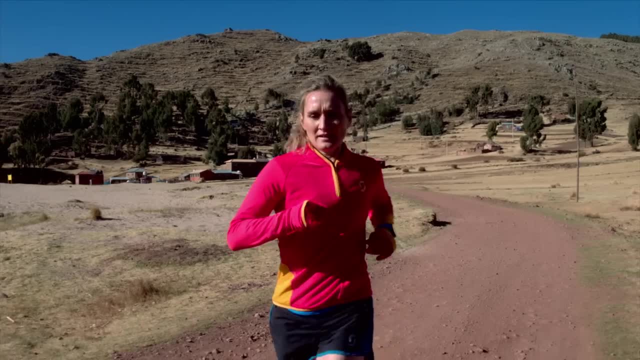 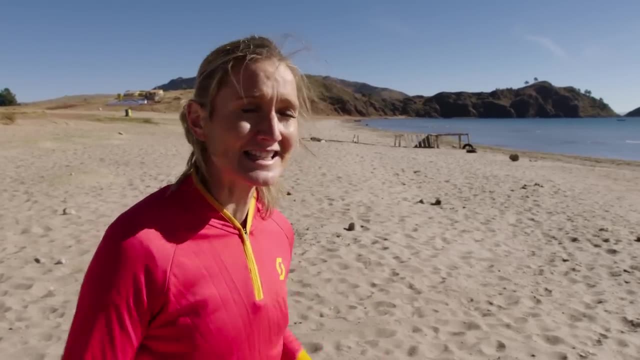 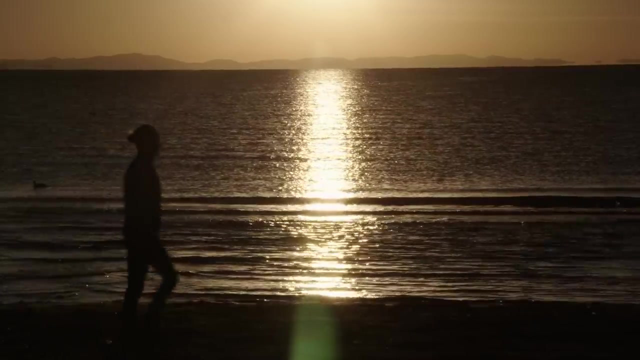 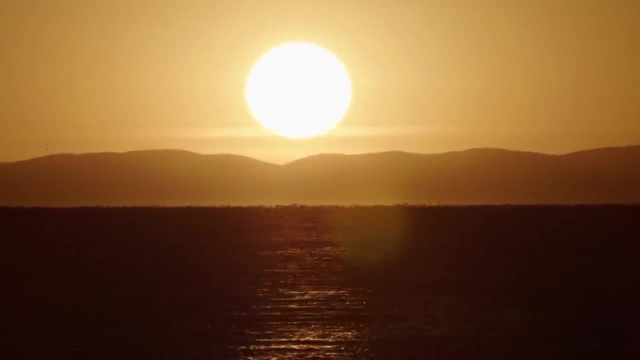 performance at altitude. this short visit has been nothing like enough to get her up to speed. The legs aren't moving fast enough because I'm not getting enough oxygen into the lungs, and the lungs are screaming. Just That was tough For athletes and adventure seekers pushing themselves to their limits here in the mountains. 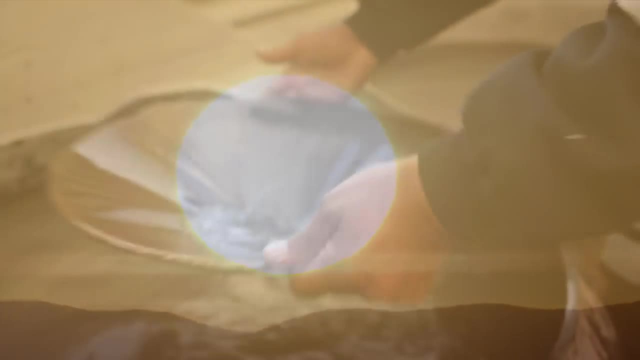 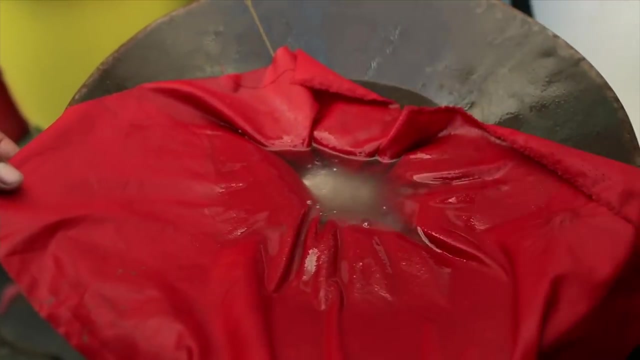 is reward enough of its type. Others put their bodies on the line for much more tangible benefits. Lust for gold has lured people high into the Andes since time immemorial. And it's not just about gold, It's about the world. It's about the world. It's about the world. 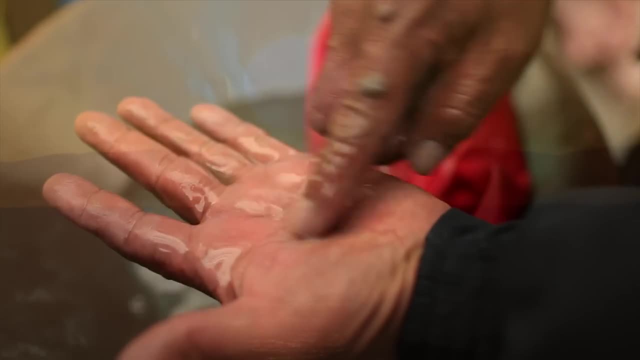 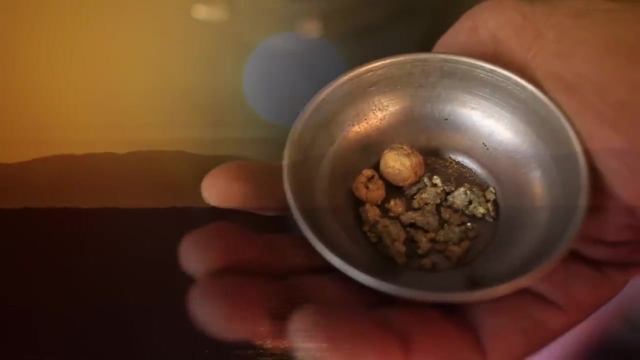 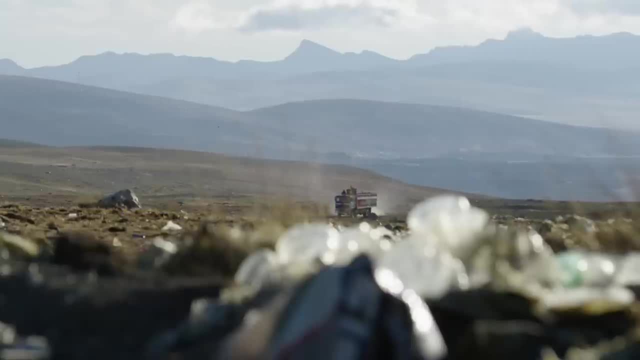 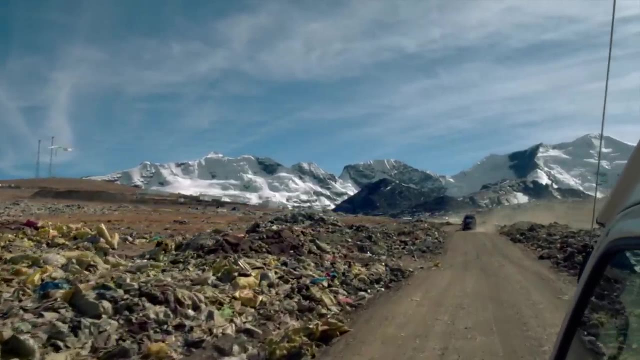 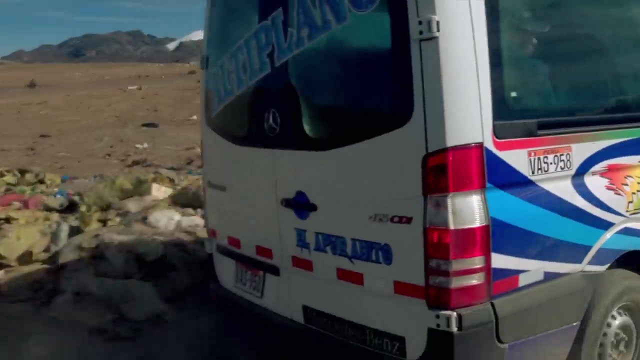 Gold is still to be found in the Andes and it still tempts adventurers to risk everything to get it. But this is not the road to El Dorado. This is the drive to La Recona. Every week, thousands of miners undertake this journey. 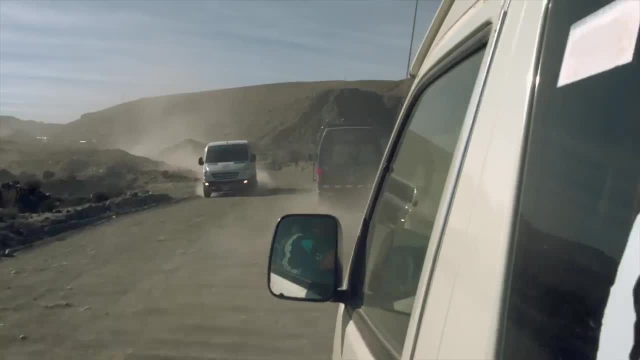 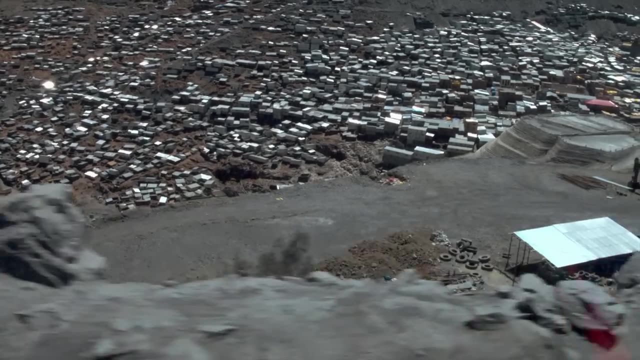 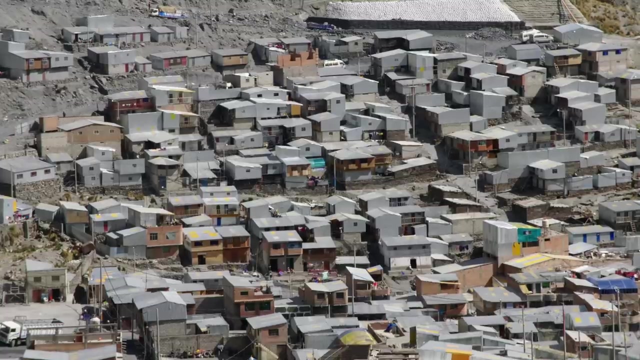 commuting up from their homes on the Alte Plane in a desperate scrabble for treasure, They're making their way to the highest town. There's gold here, 5,100 meters above sea level, but you won't find the gilded architecture promised in the myths. 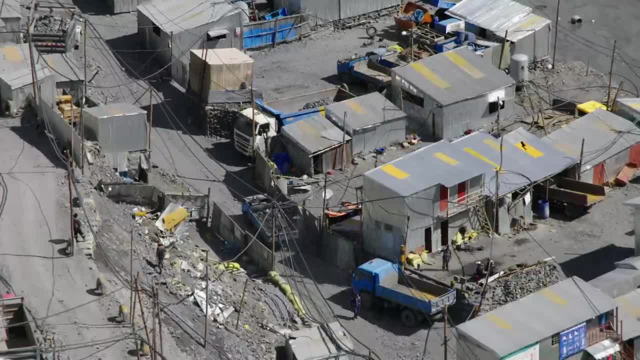 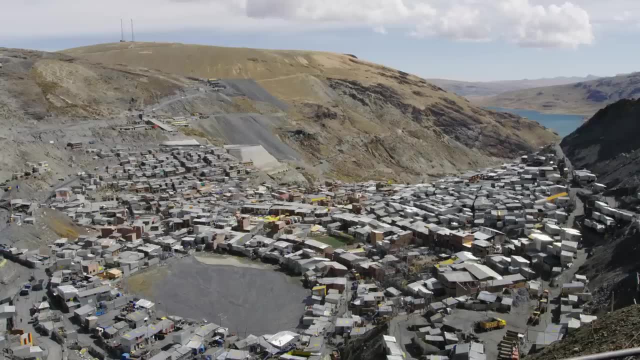 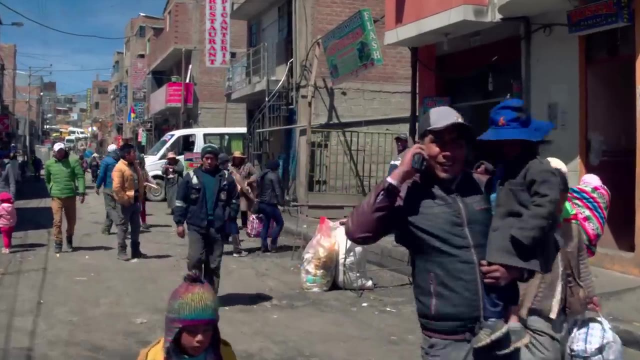 Tin huts offer shelter from freezing winds. These are the back-shift suburbs where the traveling miners sleep during their working week. The town center, a hub for the 30,000 people who reside here permanently, La Rinconada, is cursed by pollution. 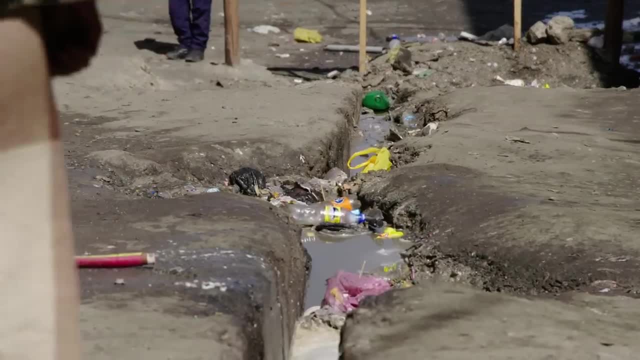 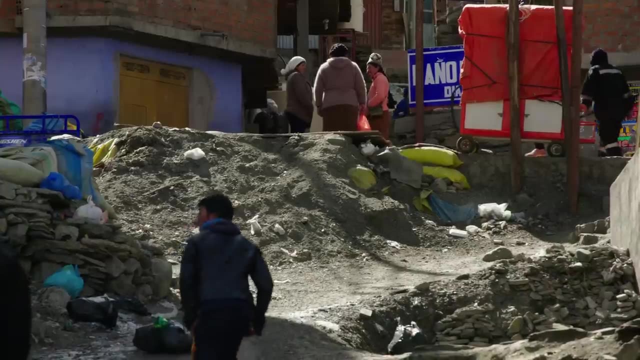 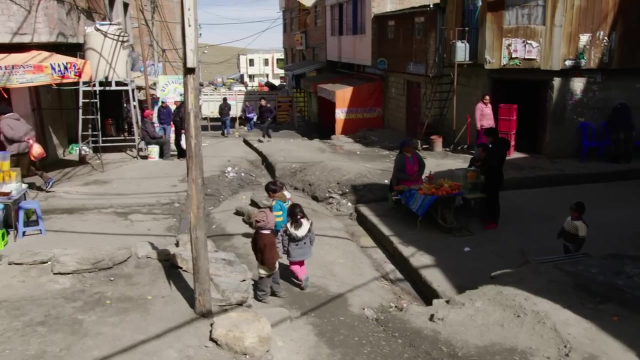 The gold-bearing quartz that's mined here is processed using mercury, and that has contaminated the water, the ground and the air, But none of that has prevented the parents of these children from rushing here. 500 years after the conquistadors, the dream of striking it rich remains all enticing. 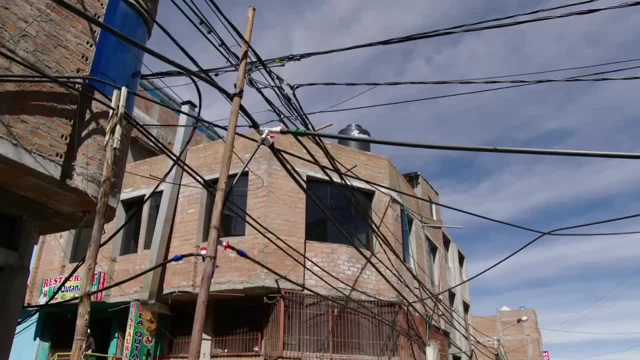 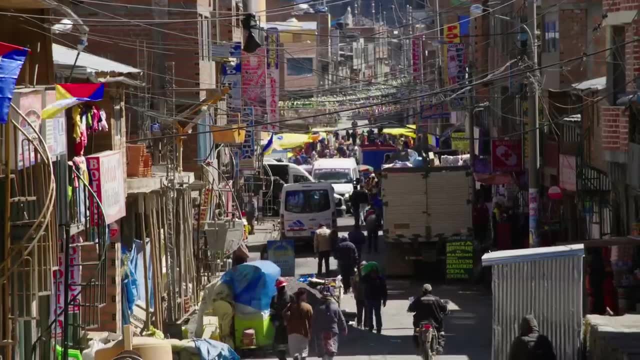 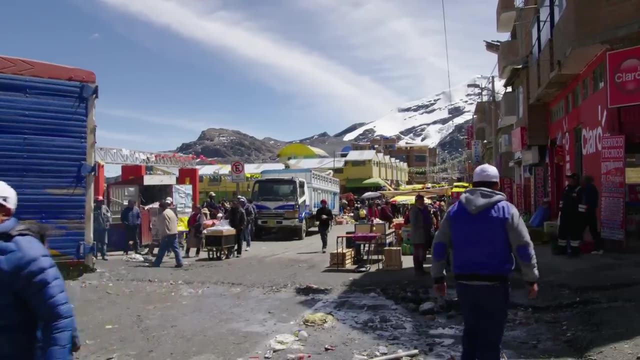 The town center is a rat's nest of electricity cables and half-built buildings. Open drains run through the main streets. There's little evidence of civic planning or control. The boom times for La Rinconada began four decades ago When mineral prices soared on global markets. 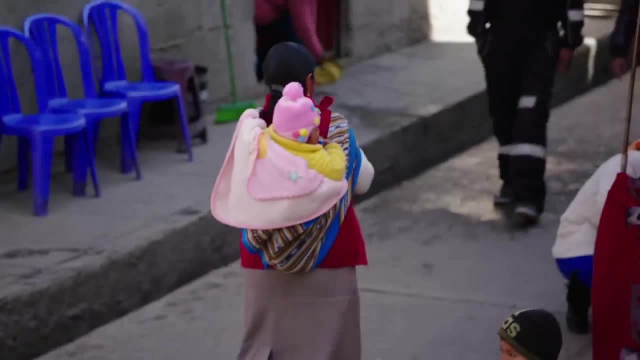 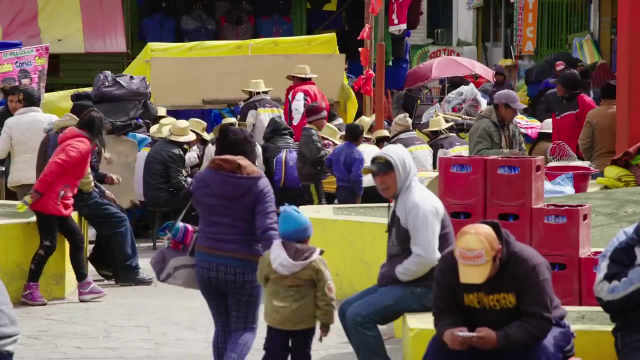 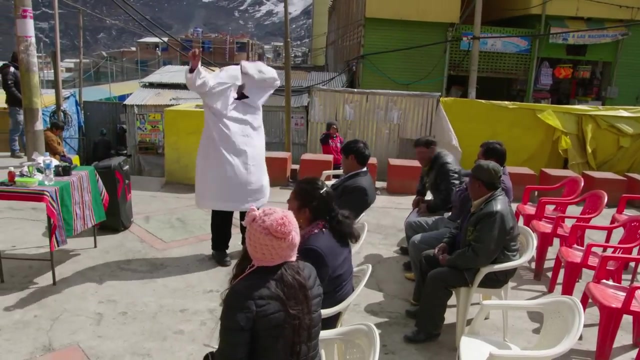 Since then, this gold-rush town has become home to a whole generation who've lived nowhere else. And despite the chaos, a sense of community is developing. New neighborhoods spring up virtually overnight. Today, the parish priest is about to celebrate an anniversary mass to mark the foundation of one of them. 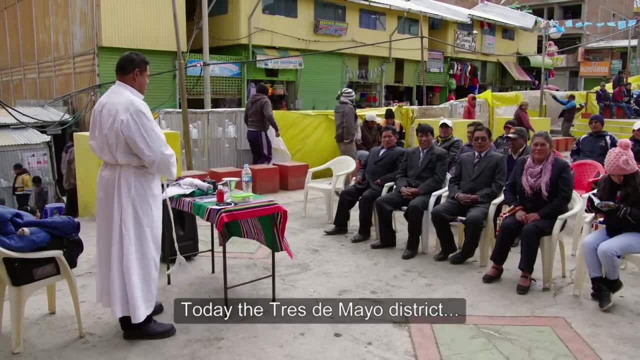 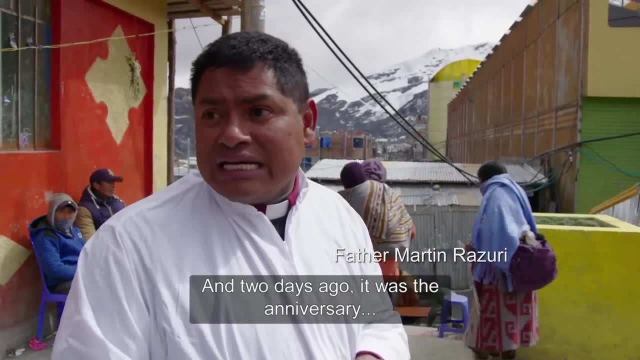 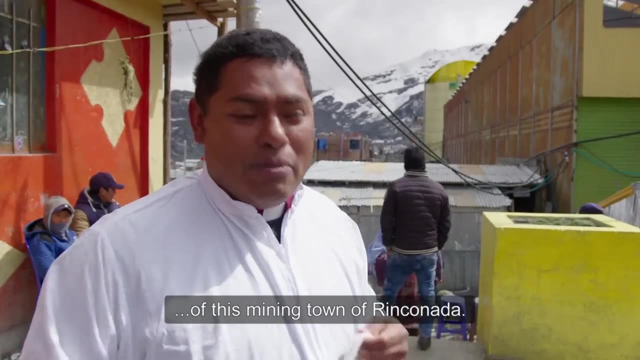 Today is Sunday, where this neighborhood of May 3rd is celebrating one more year of its creation. Two days ago, we also celebrated the anniversary of the town of Minara-Rinconada. How are you All good, And how is the family? 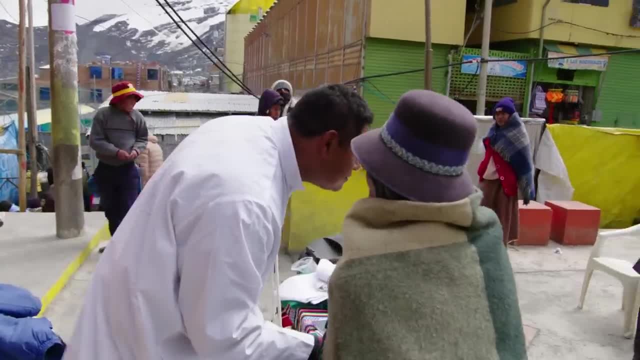 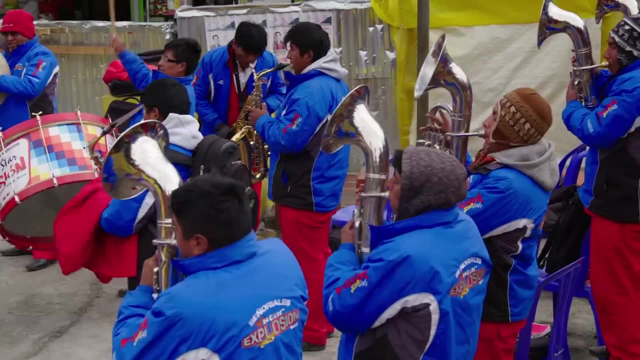 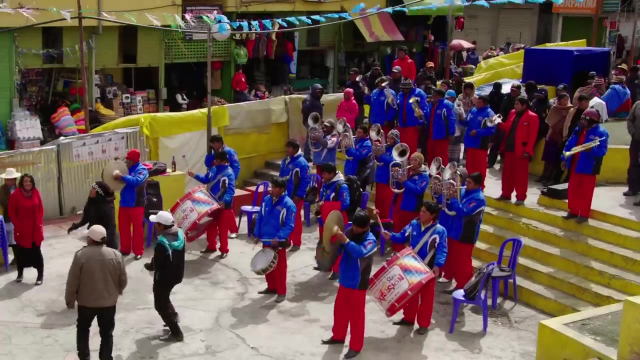 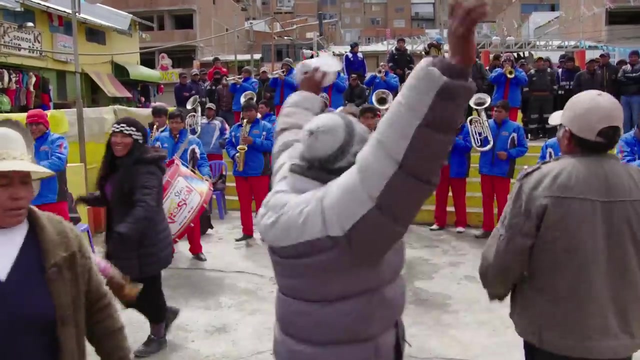 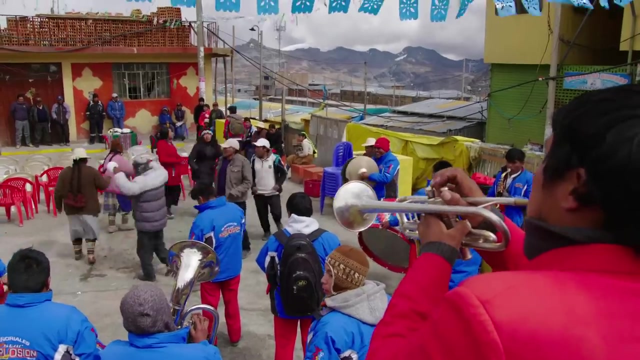 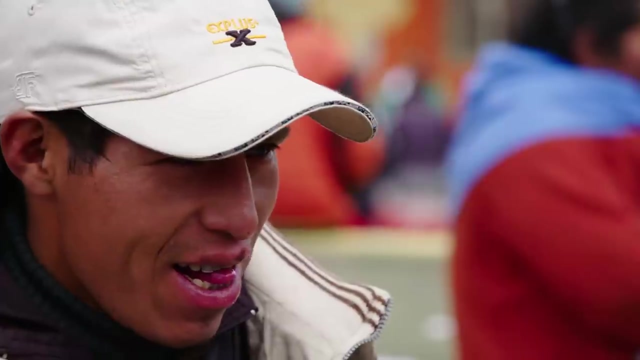 And how is your health? In the mountains, an anniversary is always a festive occasion. Andean people love to celebrate. There's a freezing wind and the threat of summer, But that's no excuse to stop the party. A special occasion can lift the spirits. 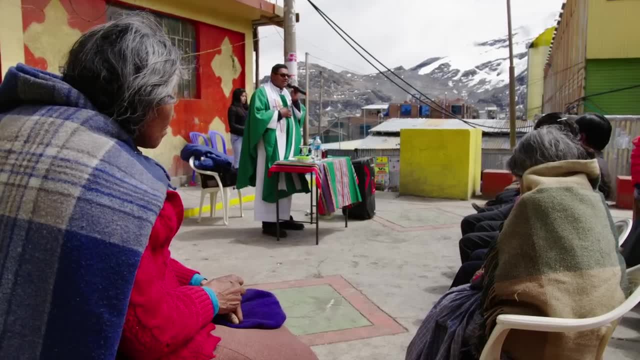 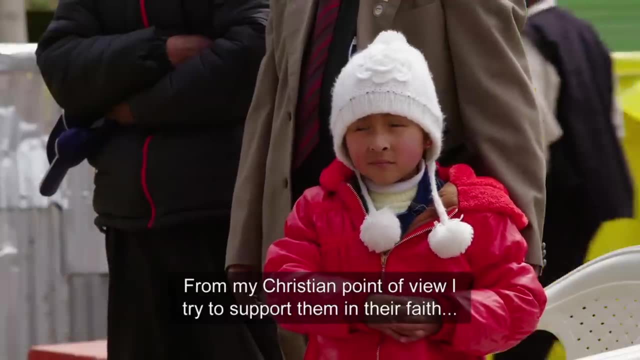 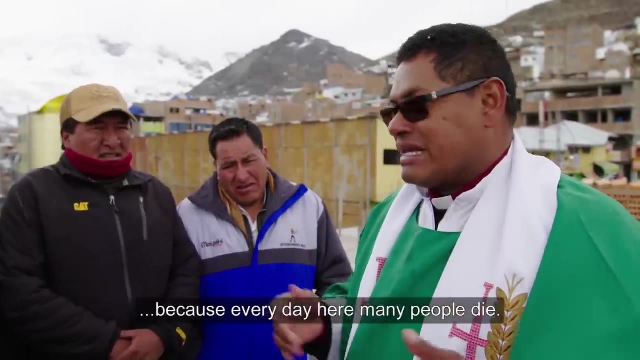 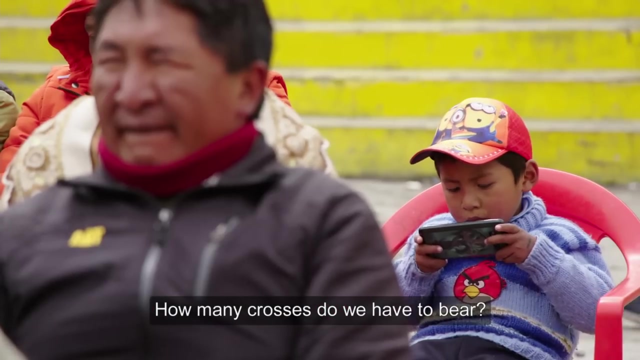 But Father Martin knows, the everyday reality for people here is much bleaker And from my point of view, from the Christian point of view, to accompany in faith, Because sometimes we know that many people die here day by day. How many crosses do we sometimes have to carry? 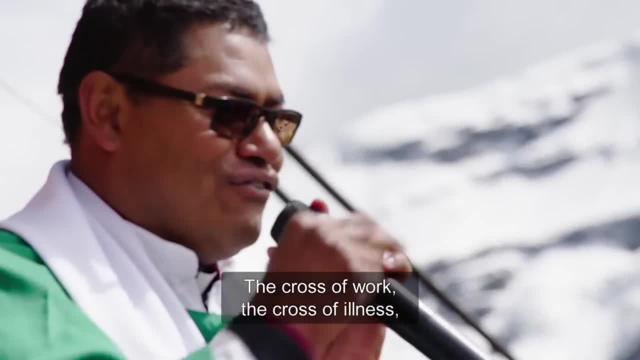 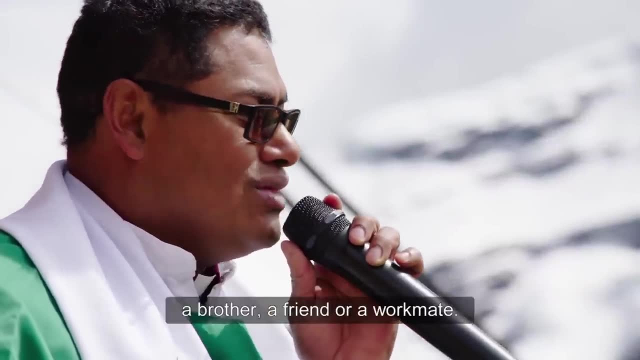 The cross of work, The cross of illness, The cross of the departure of the son of the wife, of the brother, of the friend or of the neighbor, The cross of the departure of the son of the wife, of the brother, of the neighbor or of the neighbor. 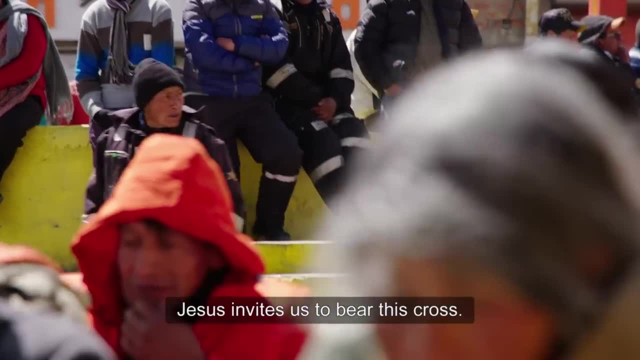 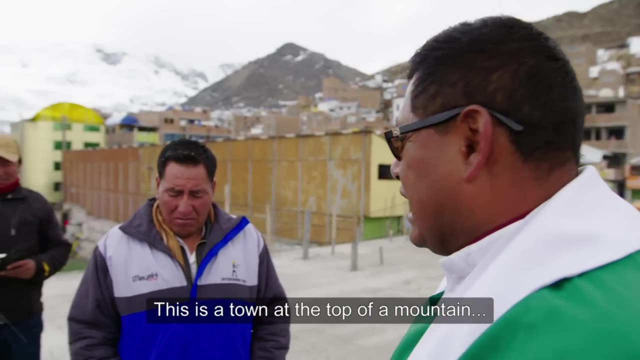 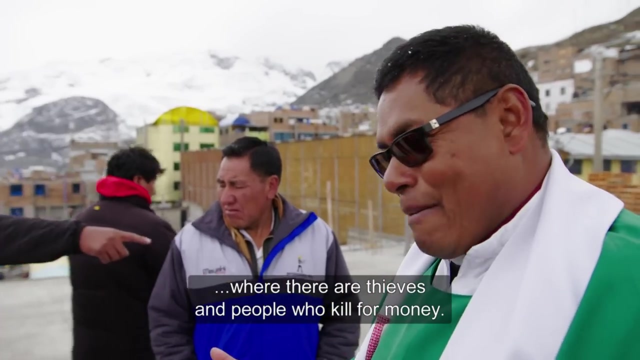 The cross of the departure of the son, of the wife, of the neighbor, The cross that Jesus invites us to take. It's a town center where, on the upper side, there are places of bad death, places of perdition, Where they go take, leave their money, steal, kill them many times to take their money. 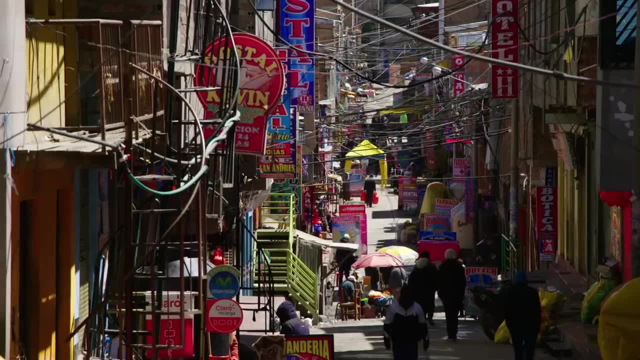 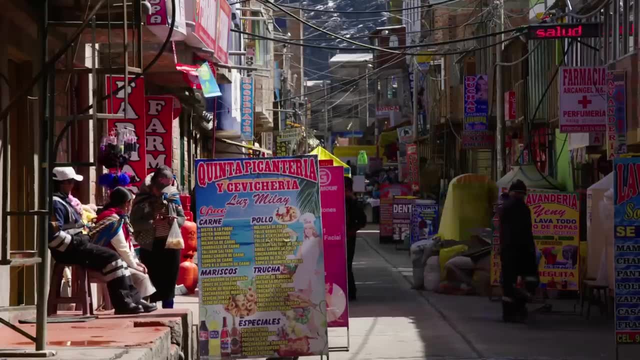 Where they go, take, leave their money, steal, kill them many times to take their money. Where they go, take, leave their money, steal, kill them many times to take their money. The bars and cantinas in the center of La Reconada echo with Gothic and Scandal. 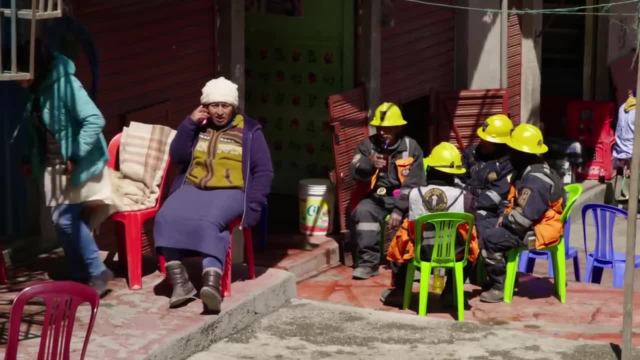 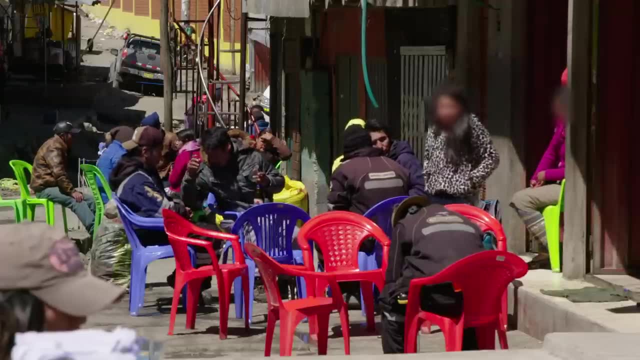 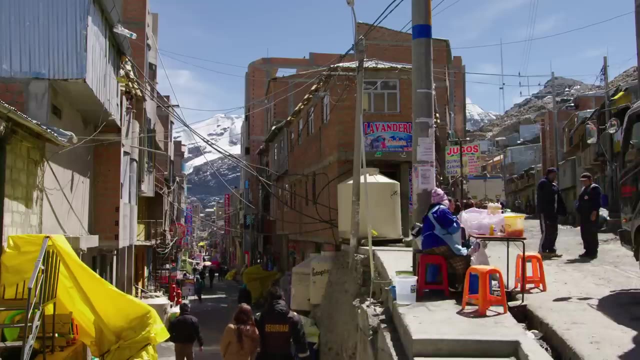 And they're awash with enough drink to fuel a Wild West style brawl now and again. Prostitution is rife here, And some of the money made in the mines gets spent in these streets. Most of it heads straight down the mountain, Leaving little behind to fund civic amenities or beef up law and order. 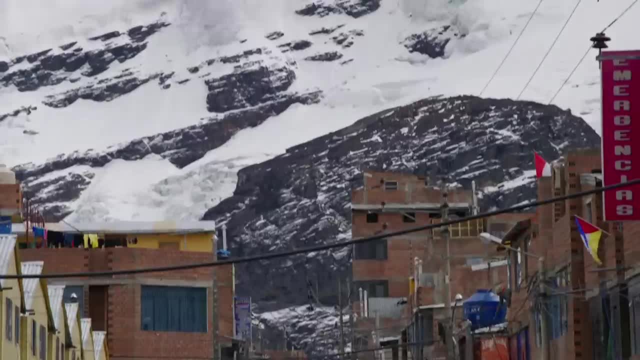 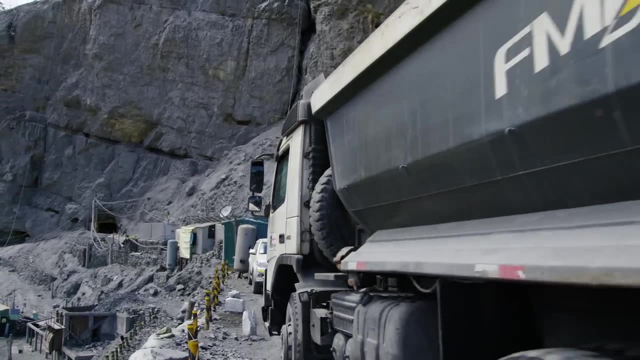 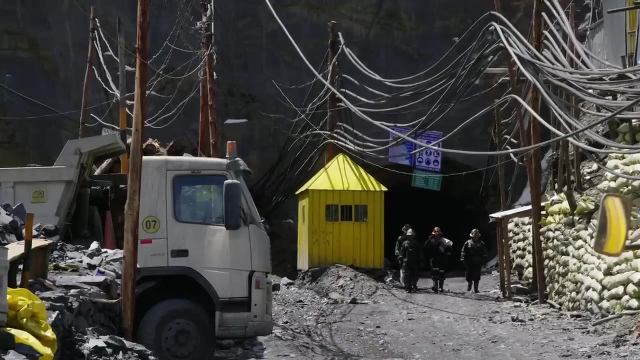 But this isn't the business end of town To find that you have to climb higher still. La Reconada's gold is dug out from shafts, and tunnels cut deep into the mountain above the town. Mining at this altitude is shot through with risk. 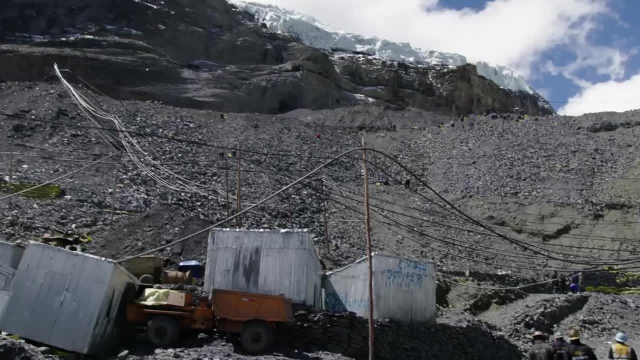 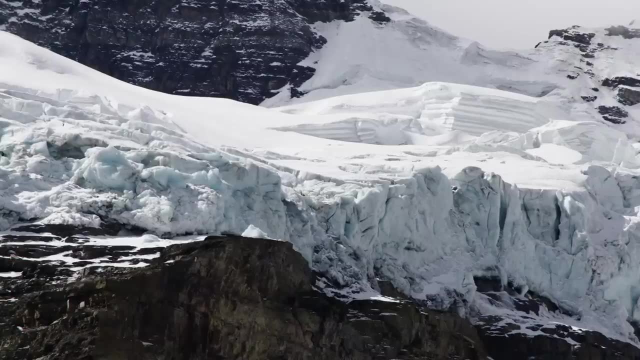 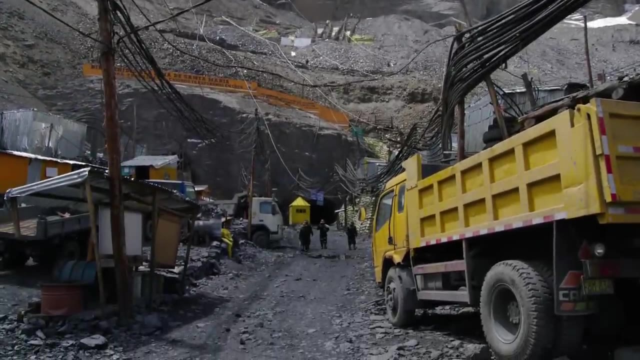 Even before they enter the darkness of their workplace, The miners brave a little danger. Directly above the works is a huge glacier called La Bella Dormiente, The Sleeping Beauty. When she stirs from sleep as the seasons change, she sends ice blocks crashing down onto the works below. 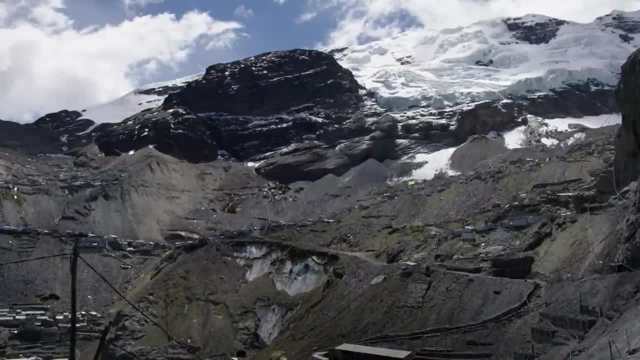 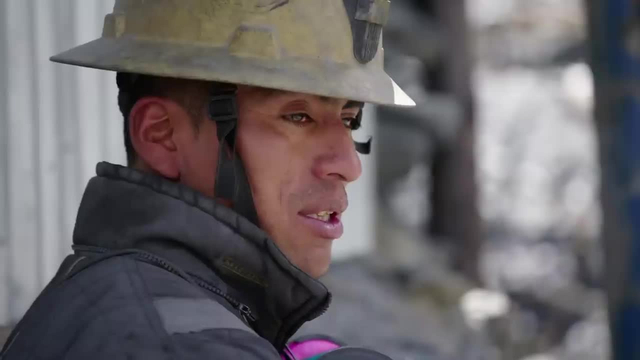 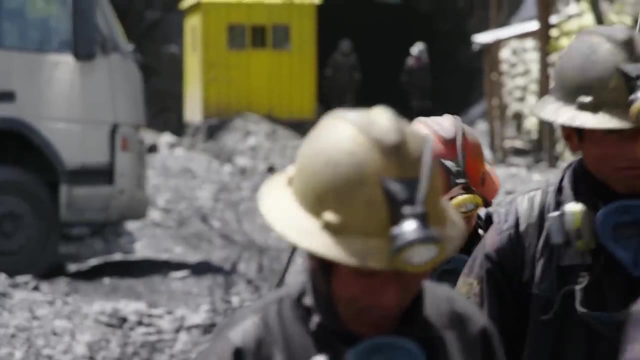 No wonder La Reconada has been dubbed an ice hell on earth. Yet thousands are willing to risk life and live here, Even though most of them aren't even paid a salary. Instead, they're rewarded under a traditional system called Cachorreo. 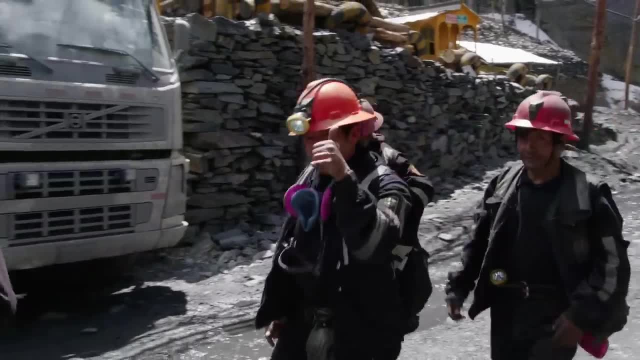 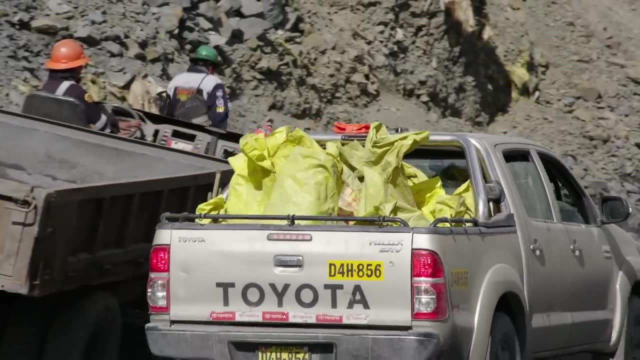 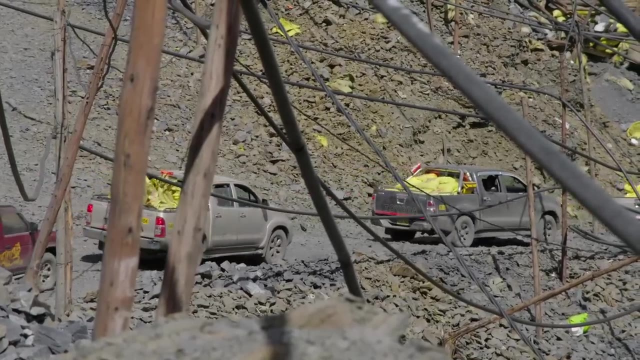 They get no cash at all, But for every month they work they get to keep whatever they can dig out from the mine on a single day. In reality, they may drive away with a little more, But there's no guarantee that there's any actual gold at all in whatever they take. 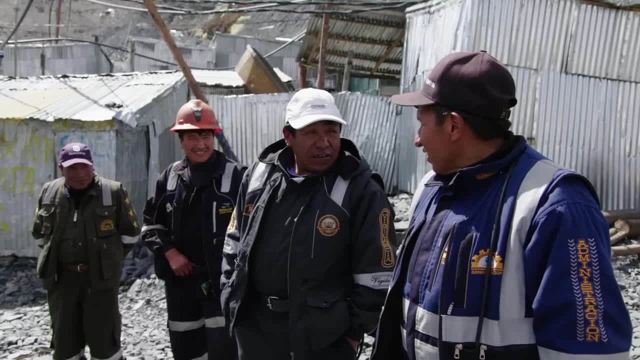 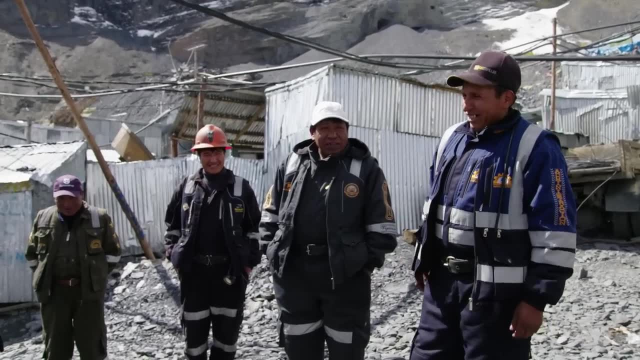 Fortunato Choque lives up to his name. He's fortunate to have survived here long enough to have graduated from laboring at the rock face. Now he's an engineering foreman on a salary, Working with one of the cooperatives who control mining on the mountain. 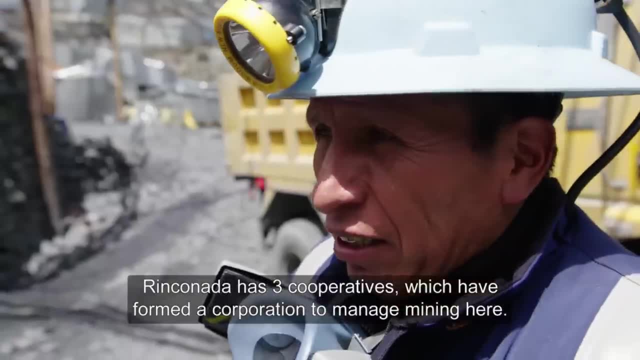 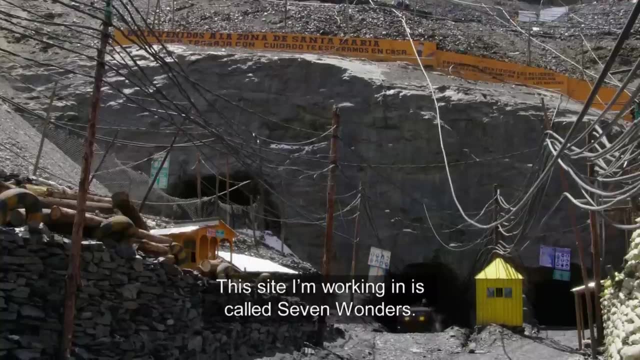 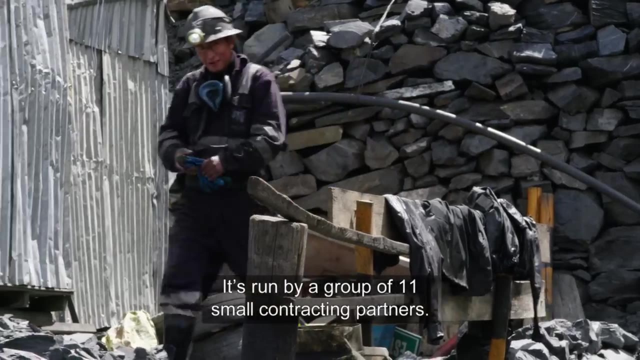 In La Reconada there are three cooperatives Where the corporation manages and the three cooperatives are the corporation. I'm working in an area called Siete Maravillas. The name is Siete Maravillas. We've entered seven contracts. 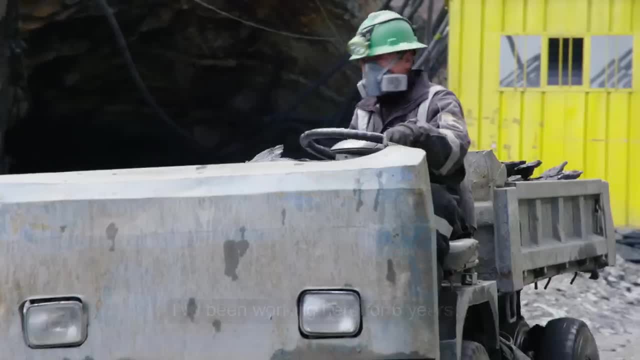 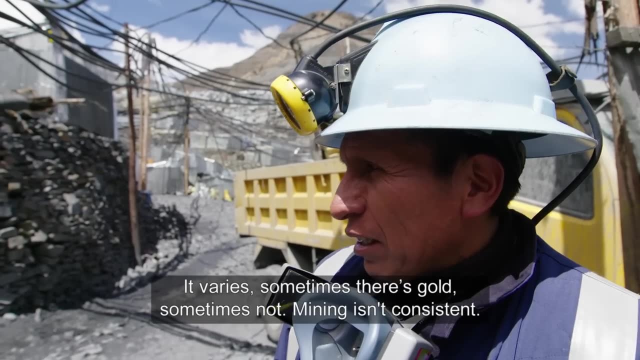 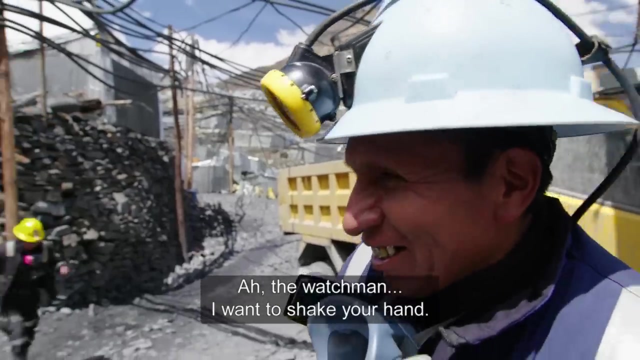 Among them there are almost eleven partners. I've been working here for at least six years, So there's a variation. Sometimes it's low, Sometimes it's low. The mine is not even. There's a strong bond between the miners here. 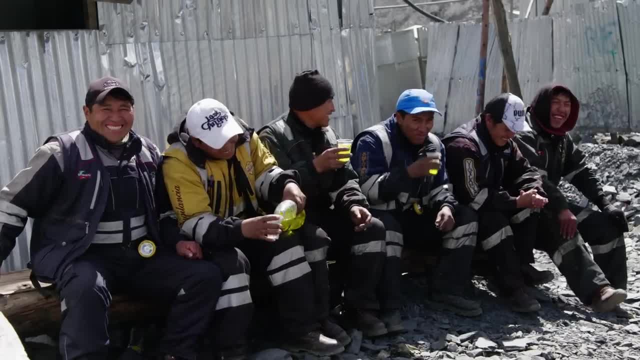 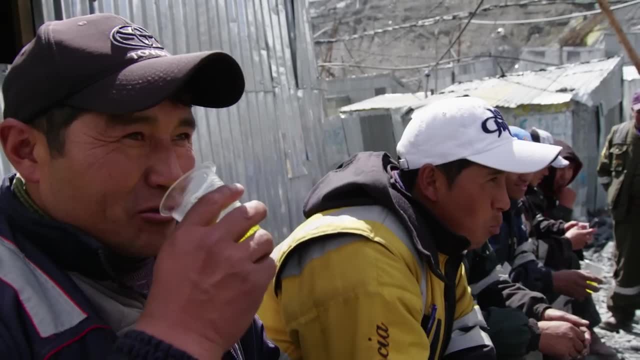 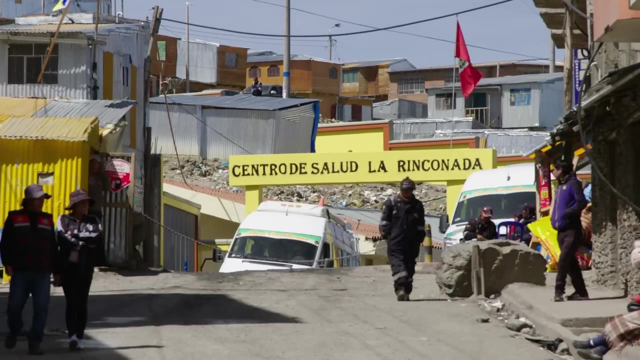 The camaraderie of men who face danger together as part of their daily working lives, But there's little for them to fall back on in the way of welfare when accidents happen. And accidents do happen. It's La Reconada's medical center which has to deal with the aftermath. 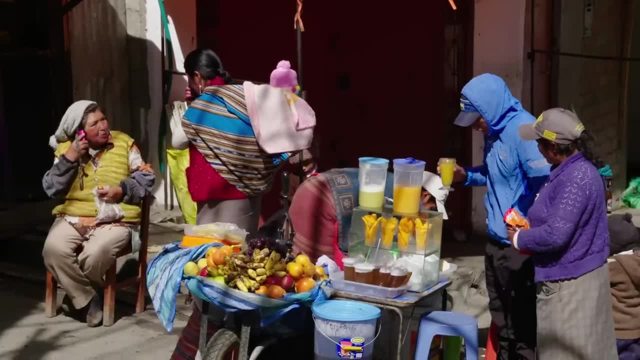 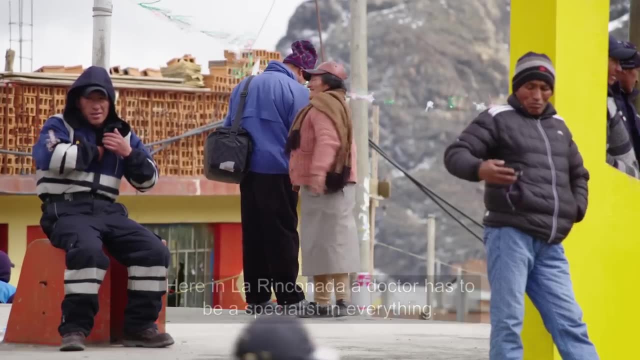 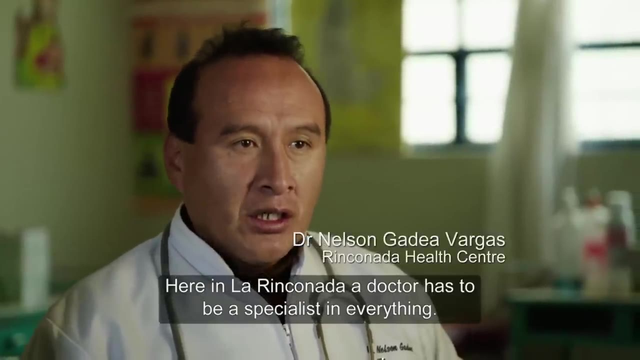 And with tens of thousands of people isolated at extreme altitude on this mountaintop. the clinic also faces a host of other calls upon its expertise. Here in the La Reconada health center the doctor has to do all the specialities. He's a gynecologist, a pediatrician, internal medicine- all the specialities. 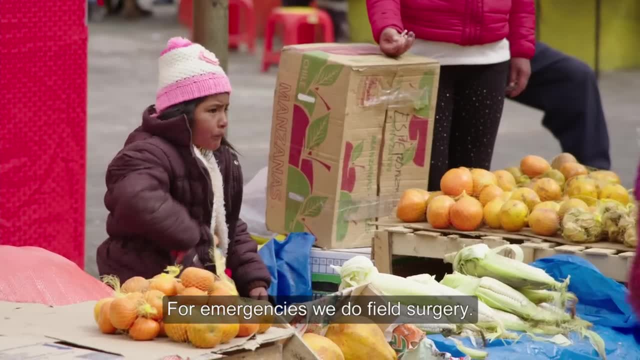 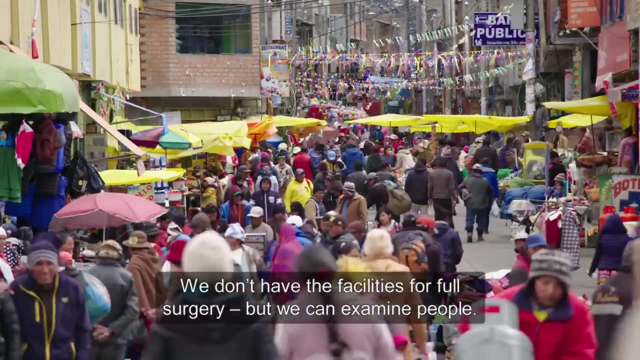 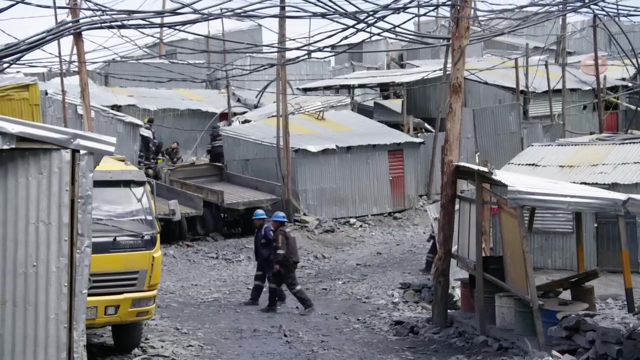 Here. in terms of surgery, we do war surgery. We don't have all the proper conditions to perform the surgeries, but we do perform them, Directly or indirectly. it's the fallout from the mine which puts most strain on the medical facilities here. 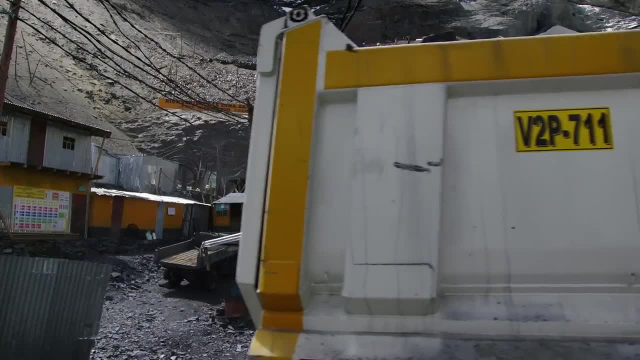 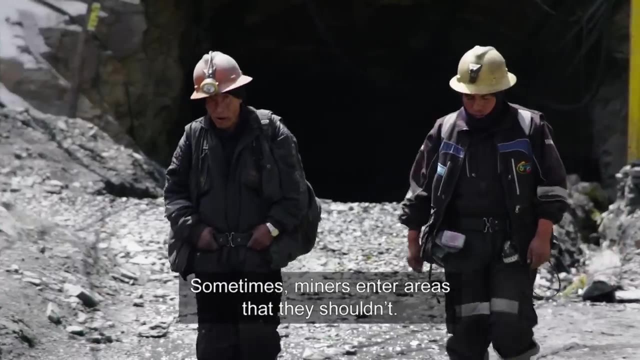 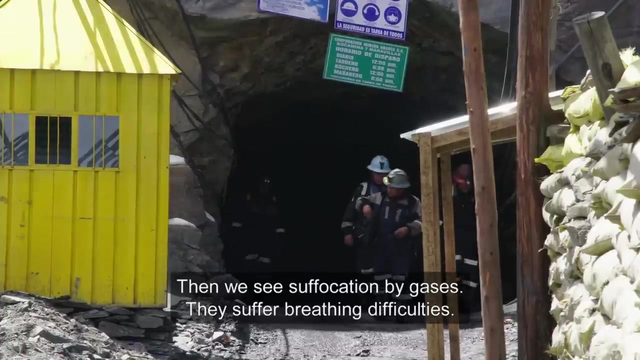 Compared even to other South American countries, Peruvian mining has a very poor safety record. There are times when the people of the mining population are neglected Places where they shouldn't enter they do, And that's where they get suffocated. 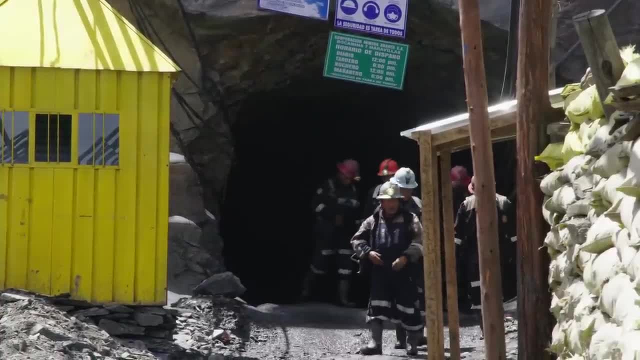 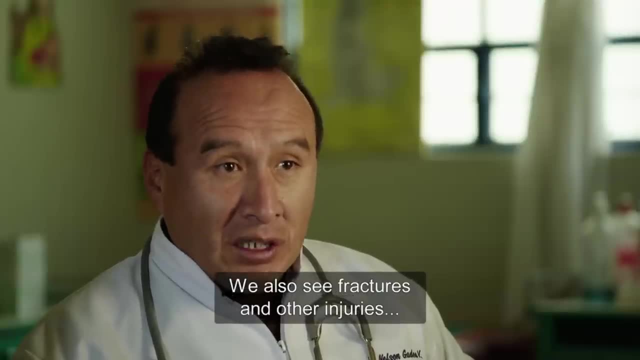 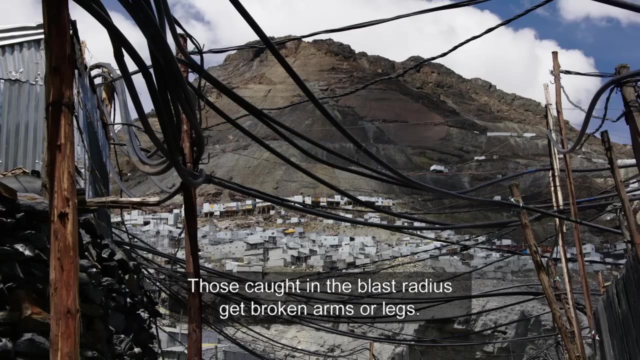 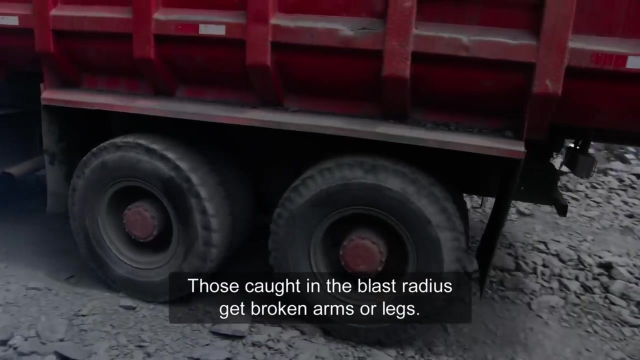 That's where they get gassed. that's what they call it. Another case is sometimes the fractures that some patients have When they manipulate something wrong. it could be an explosive. Sometimes the expansion radius alters the human limbs, the upper or lower limbs. the fractures, 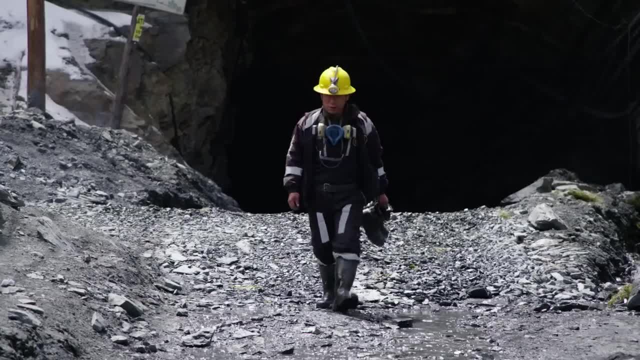 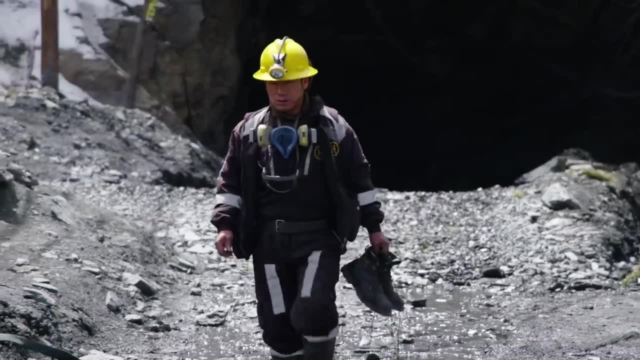 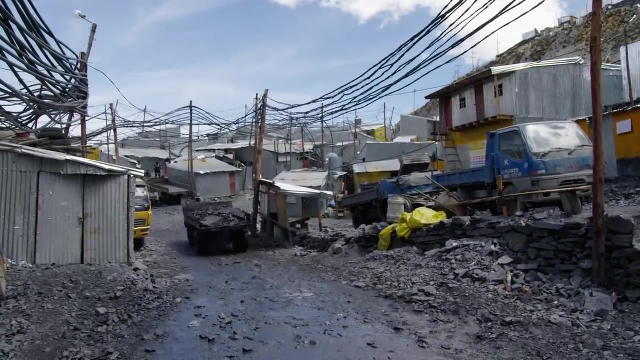 And that's where the pain begins. Tragedy is something medics in mining communities all over the world have had to learn to cope with. Here it's so free, it's virtually an accepted fact of life. But that doesn't make it any easier. 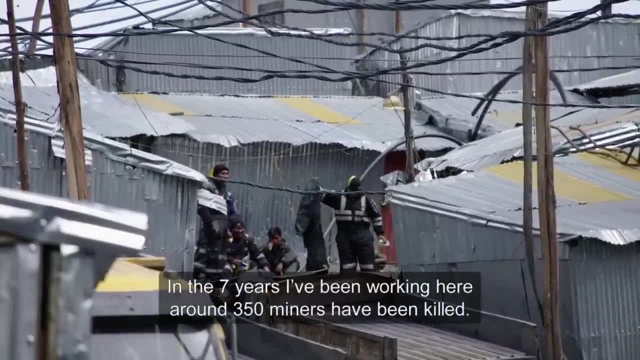 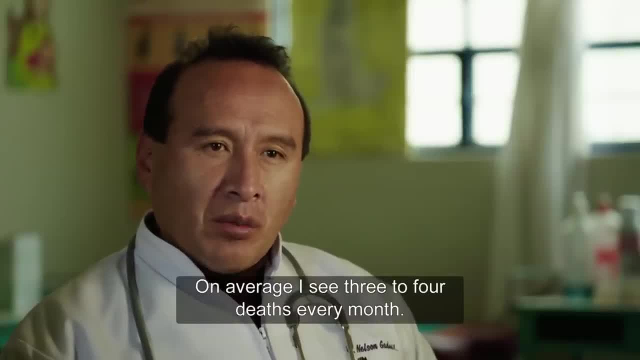 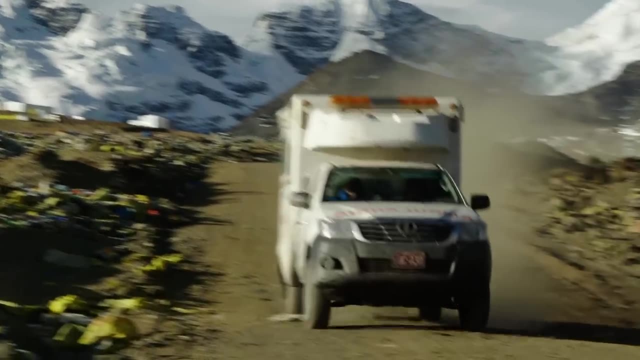 So in these seven years that I've been working here in the Rinconada mine, there are an average of 350 people Monthly. about three to four people. That's the average per month of deaths. Other dangers lurk in town. 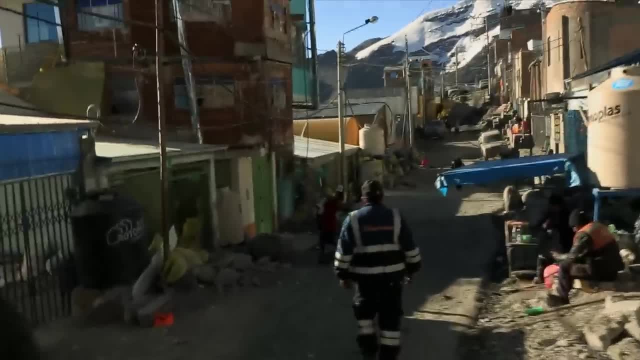 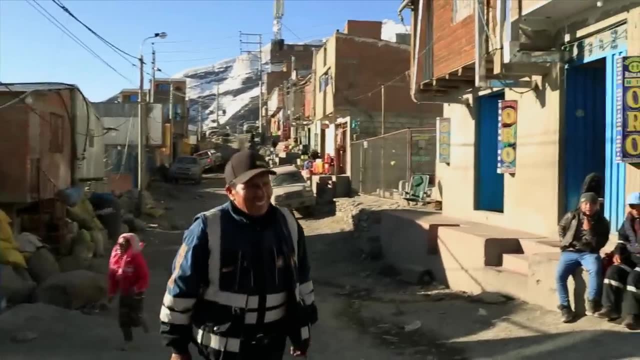 Fortunato is keen to take us to a notorious backstreet neighborhood, But only if we film undercover Using a tiny palm quarter. we followed him to a place where miners bring their small caches of ore to be refined. Film crews aren't welcome here. 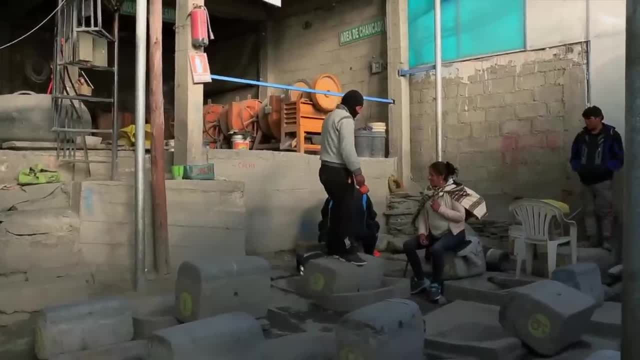 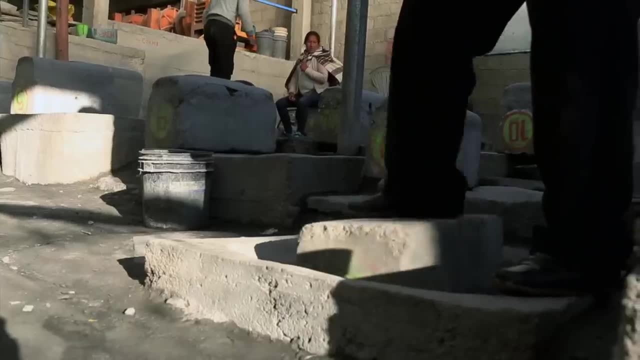 It's an edgy sort of place, with a whiff of the black marketing gear and a hint of violent crime not so far away. This is where the quartz is ground down and then mixed with mercury, which sticks to the gold Despite the obvious health risks. 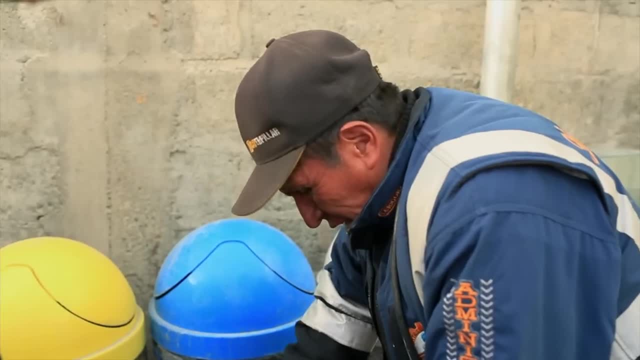 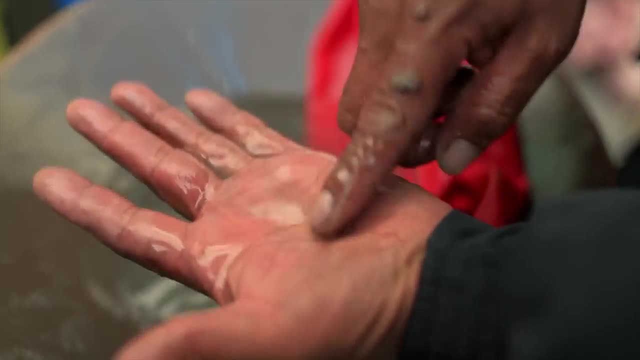 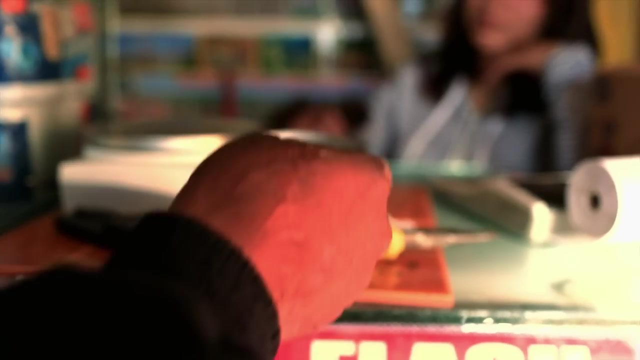 getting hands-on with mercury themselves is the cheapest way for miners to refine their gold. The amalgam is heated to evaporate the mercury And this is the end product: Nineteen grams of La Rinconada's finest, worth around $800 on the street. 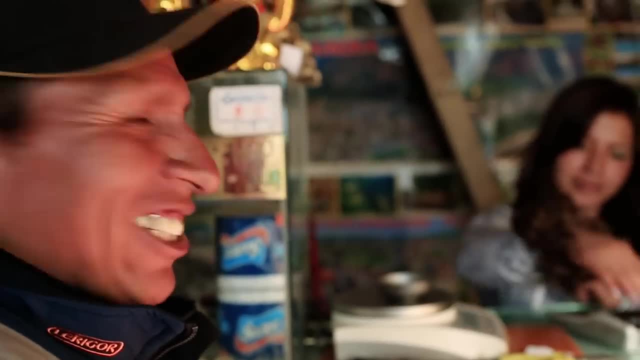 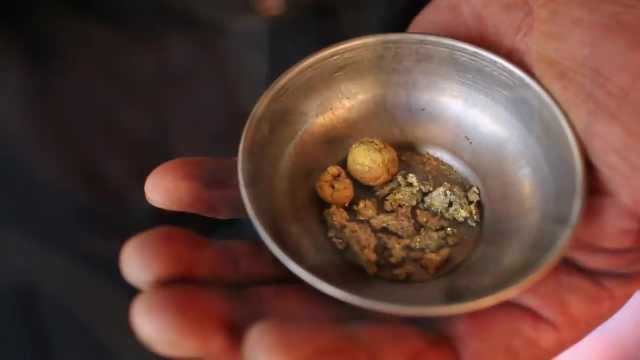 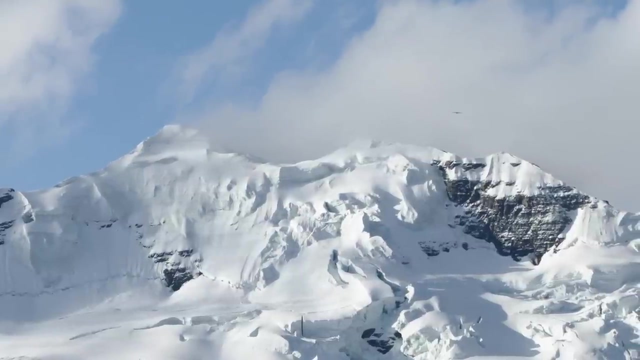 cash in hand, no questions asked. It's the currency of life here, legal or otherwise. There are other ways in La Rinconada to try to get your hands on the precious metal: Combing through the waste tips for tiny pieces of quartz. 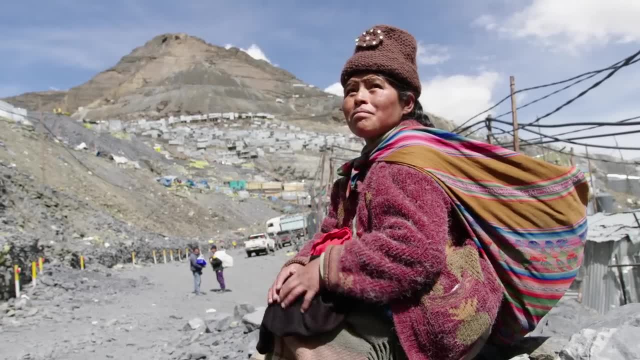 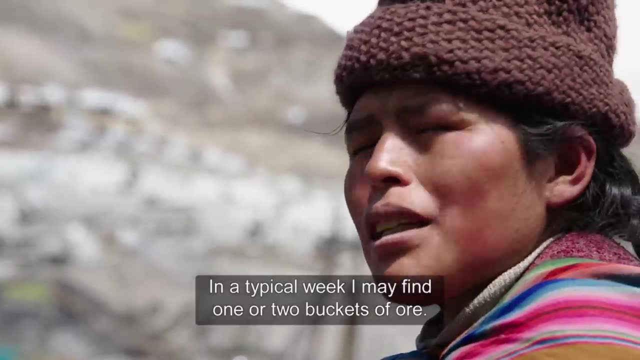 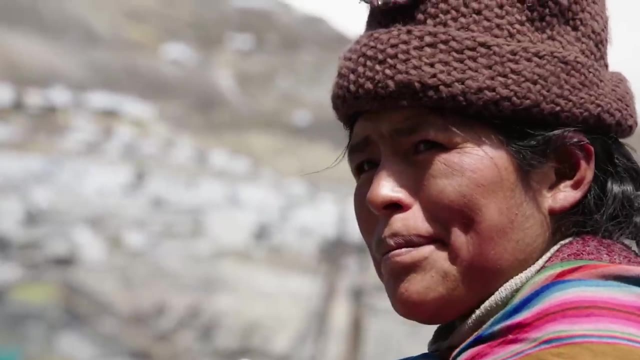 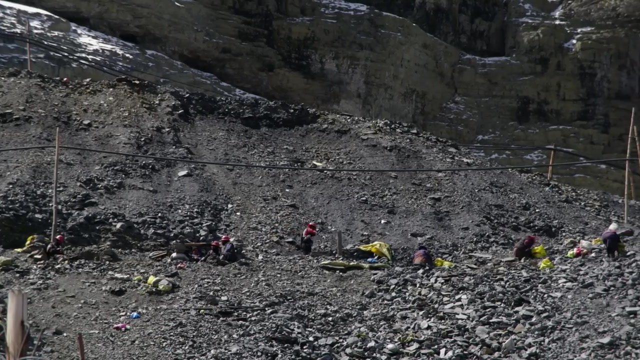 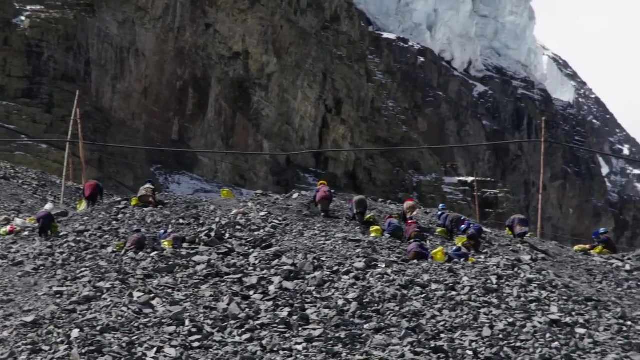 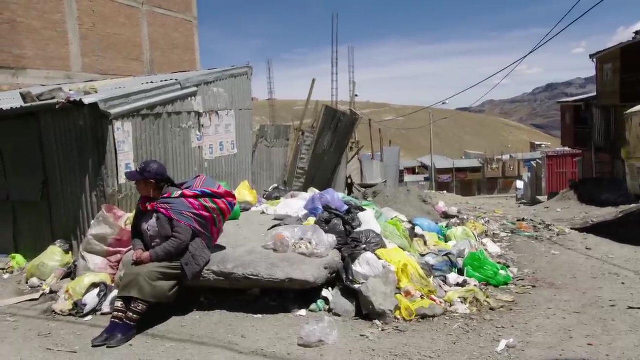 These are the palaqueros Gold scavengers. Most of the palaqueros are women driven here by extreme poverty and the faint hope of earning a few soles. Each has her own story, but typically it adds up to desperation. 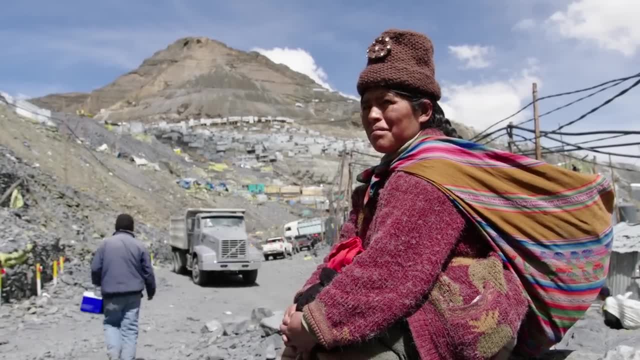 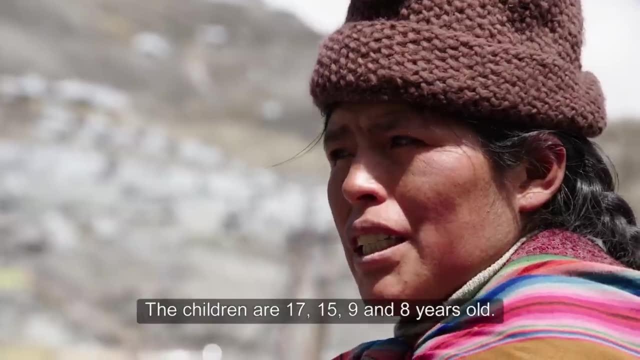 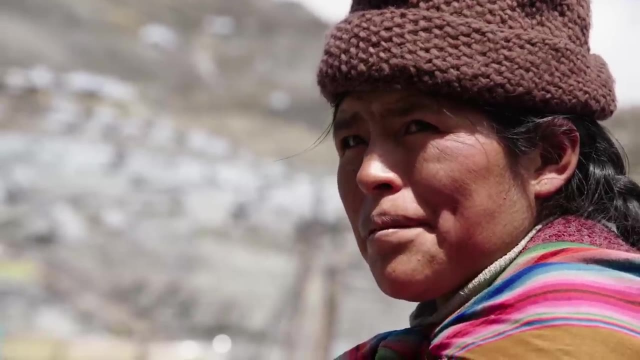 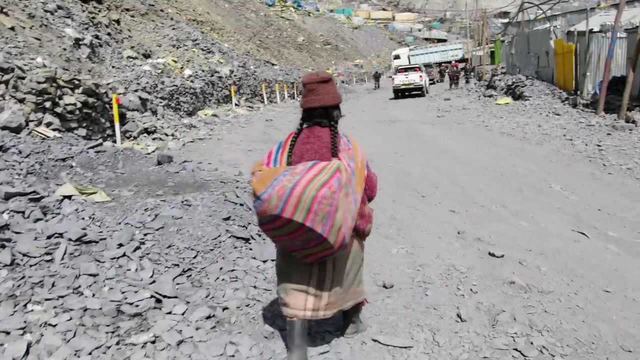 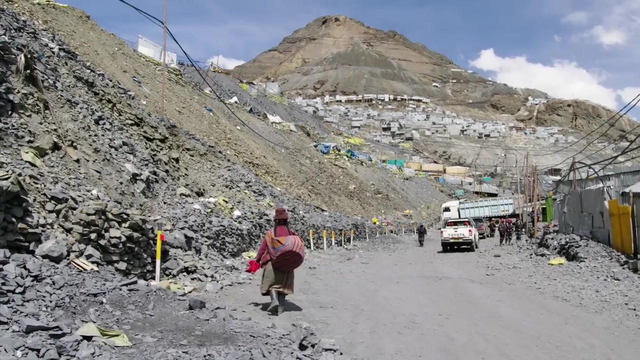 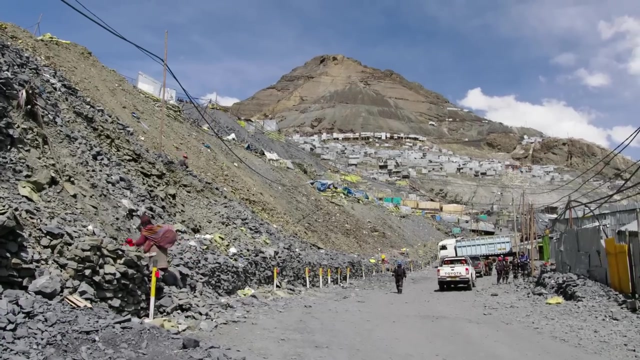 A last throw of the dice to save the families they've left behind. Mountain gold seems to promise an answer to so many people's pain and poverty. Just one small nugget may change a whole life, While the wait for a lucky strike goes on. 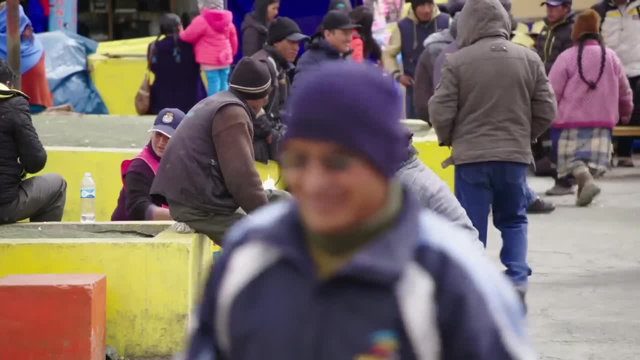 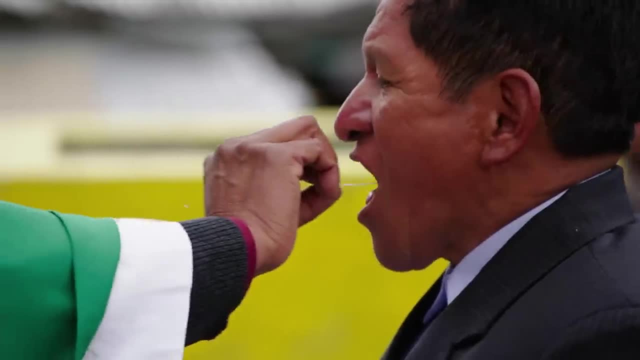 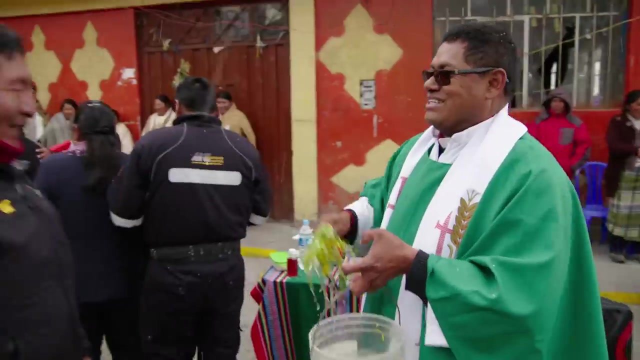 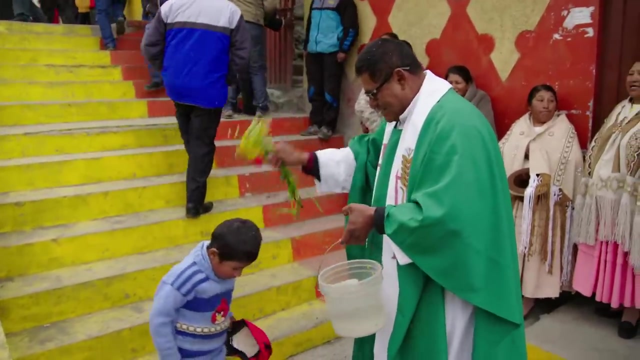 people develop their own mechanisms of survival. Even when danger and misery seem overwhelming, the human soul finds sustenance: Compassion, tenderness, comradeship. Something is holding this town together in spite of the chaos and suffering. After mass, Father Martin climbs the steps. 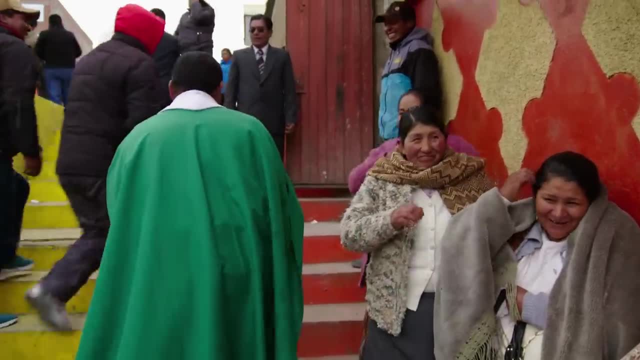 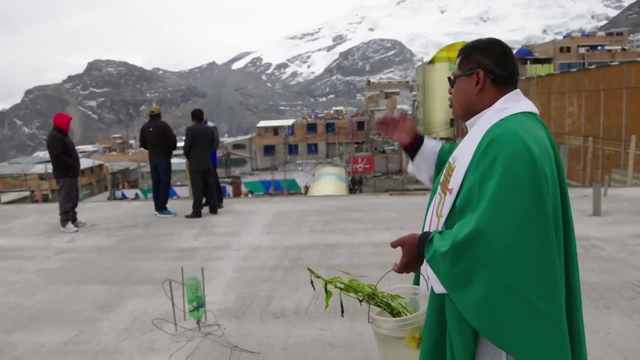 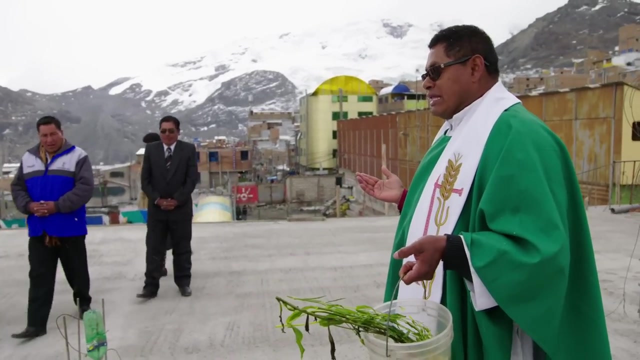 to inaugurate and bless the roof of a brand new building. It's a community centre, a tangible sign of the common purpose the residents have found here In the name of the Father, the Son and the Holy Spirit, Amen. It's proof that even for those, 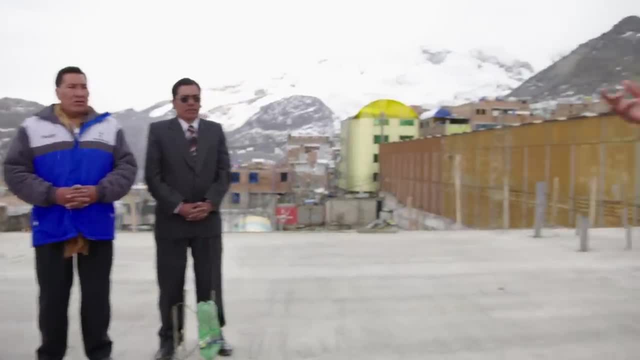 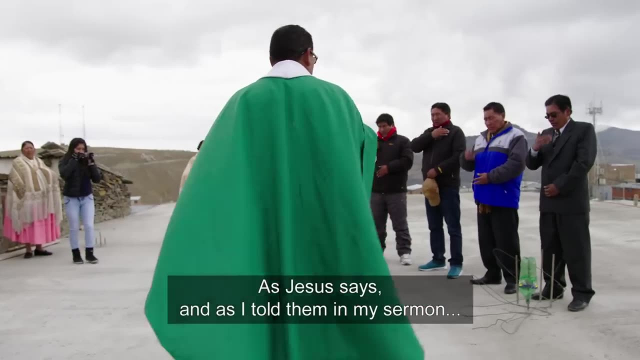 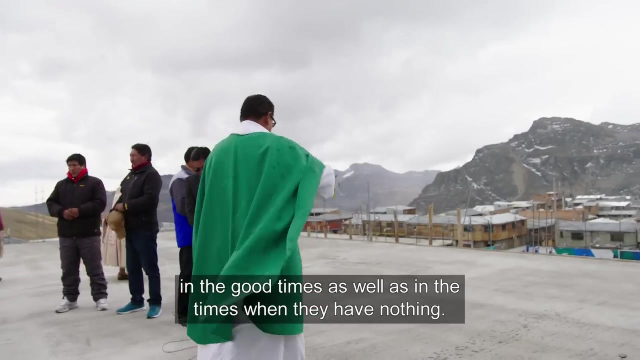 at the edge of human endurance. there's more to life than grasping for gold, As Jesus always tells us. what the Gospel says today: carrying the cross every day, at work, in the good times they have as well as in those times.